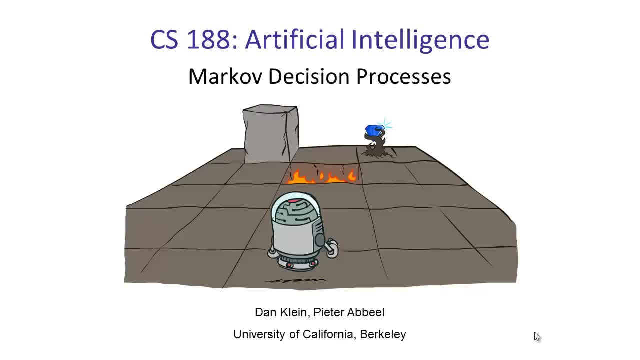 All right, any questions before we get started today? Any questions? All right, All right. well, today we're going to talk about Markov decision processes. Whenever you hear those words, what you should think is non-deterministic search. 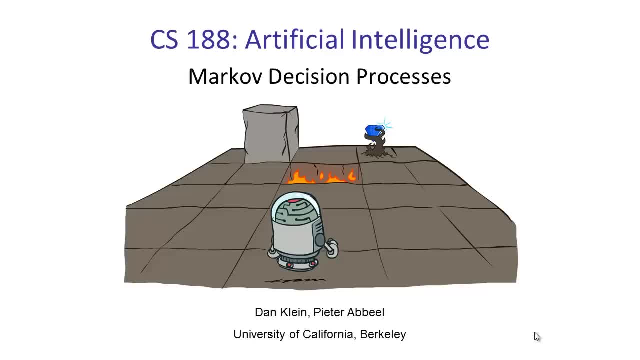 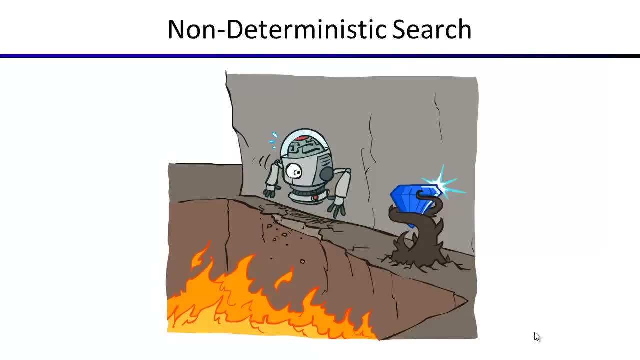 Okay. so MDPs, though they sound like something totally new, are in fact just a kind of search, where the outcomes of your actions are uncertain. So why might you have non-deterministic search? Well, in the real world, you can choose the actions you take, but you can't choose how. 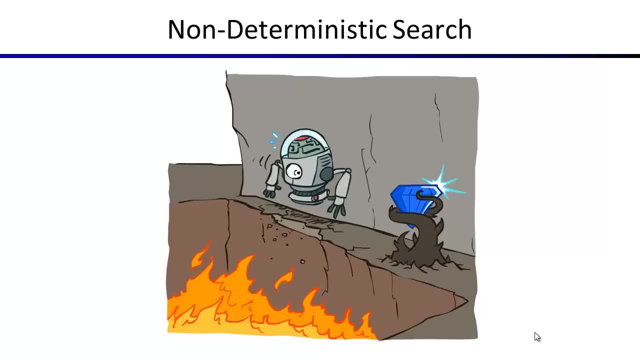 they'll actually play out in the world. So, for example, if you're this robot here and you're kind of skirting the edge of the cliff to get the gem, well, you can choose to move towards the gem, but you don't actually. 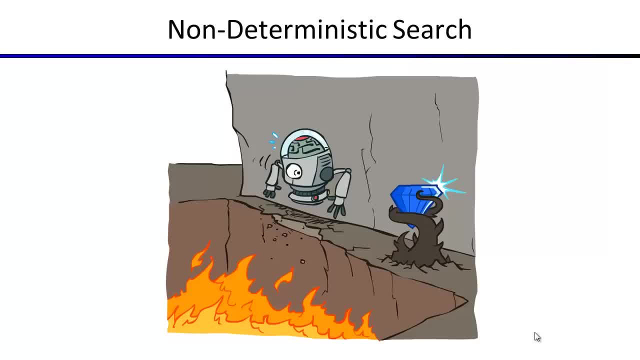 control whether or not the cliff is going to collapse and you're going to fall to your fiery death. So in this case, we would think of the choice to move rightward as an action. You control that And the outcome- whether you reach the gem or fall to your fiery death, that's the outcome. 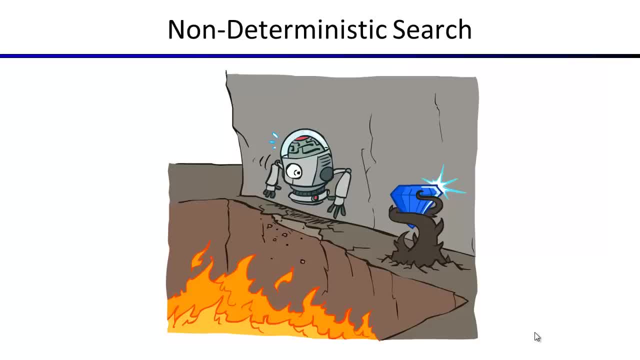 of the action which you don't control. Now, even though you don't control it, you'll be able to place a probability distribution over it. So a lot of this machinery we've seen from Expectamax will be very relevant here. 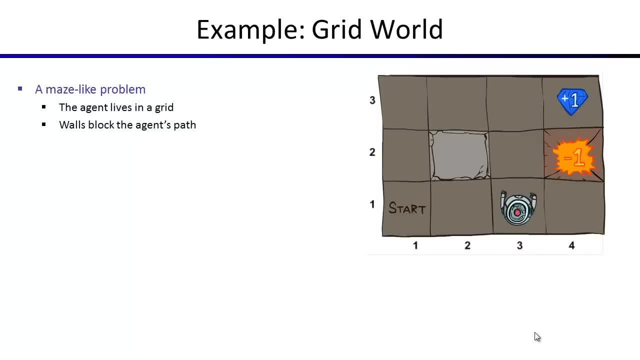 We're going to have a couple examples of Markov decision processes, or MDPs as we'll call them for short. The first example is going to be a grid world, So it's kind of going to be a maze again, like our search example, which was a maze. 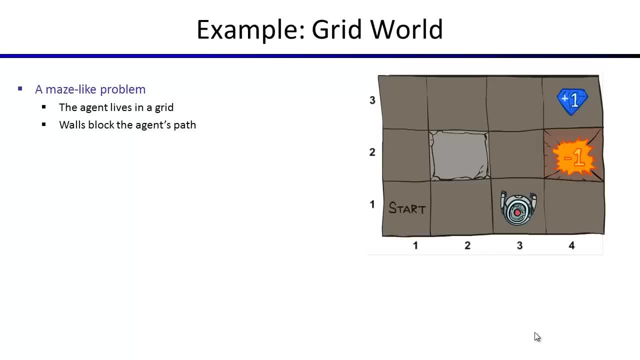 But we'll see other examples that aren't maze-like. So let's just first think about this maze-like problem. In this problem, the agent lives in a grid and here's a 4x3 grid. This is actually the same grid if you're following in the Ruslan Norvig book, if you're. 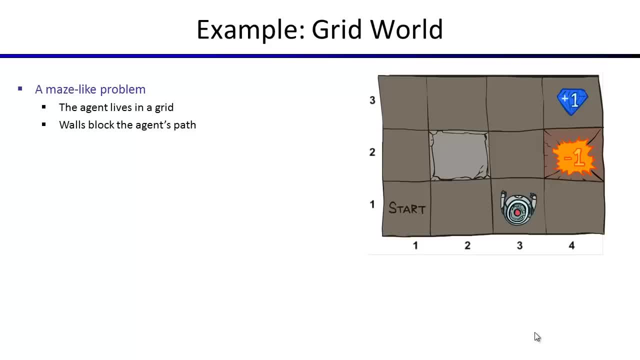 using that. they use this exact same grid here so you can line everything up. The agent lives in a grid and there are various walls, So here that kind of light gray area is a wall And you want to move around. 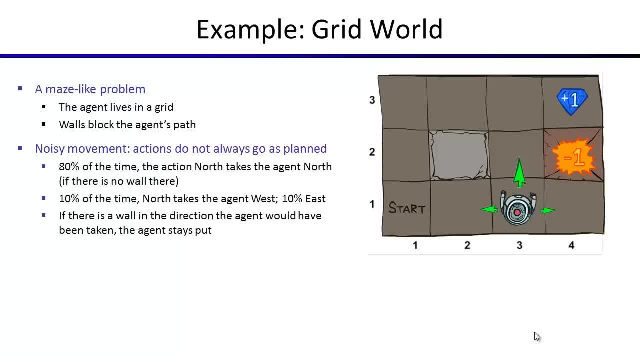 The problem is your movements do not always go according to plan. So, in terms of actions, you always have the choice of moving north, south, east or west. That's your action. Whether or not you actually move one square north or east or west is not entirely under. 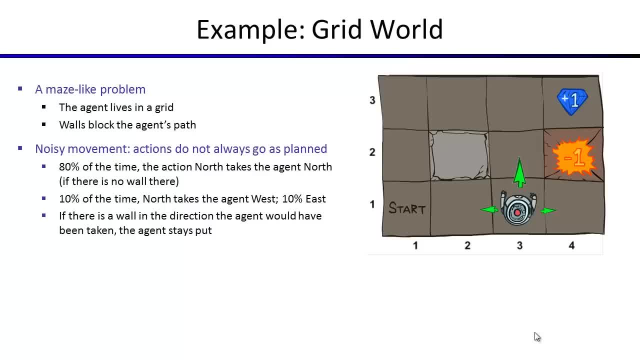 your control. So the rules okay and you only really need the fine print when you go to work out an example. So the rules are that 80% of the time the action does what it's kind of meant to do. 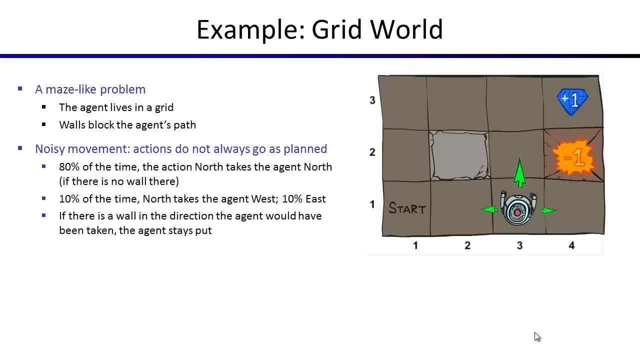 So 80% of the time, if you choose the action north, you actually move one square north. 10% of the time the action goes at a right angle clockwise, and 10% of the time it goes at a right angle- counterclockwise. 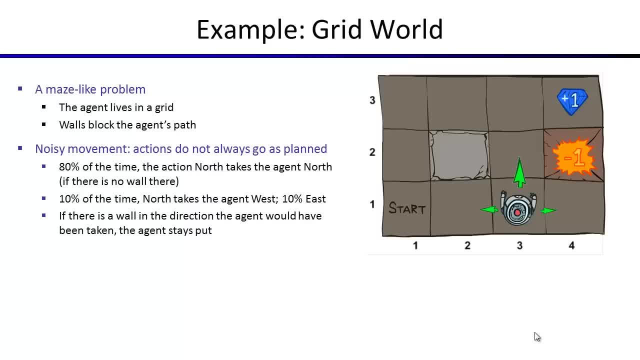 So, in the case of north, 10% of the time you actually go west instead and 10% of the time you go east. Okay, you can't actually directly stay in place or slip backwards In this grid world, though you can make up your own grid world where the details are. 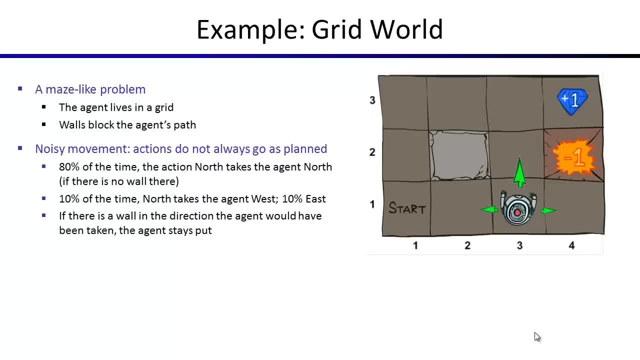 a little different. Okay, there's one complexity, which is, once you resolve this 80-10-10 thing, if that direction would result in hitting a wall, then you stay put. So, for example, if you are where this robot is right now and you choose south, 80% of 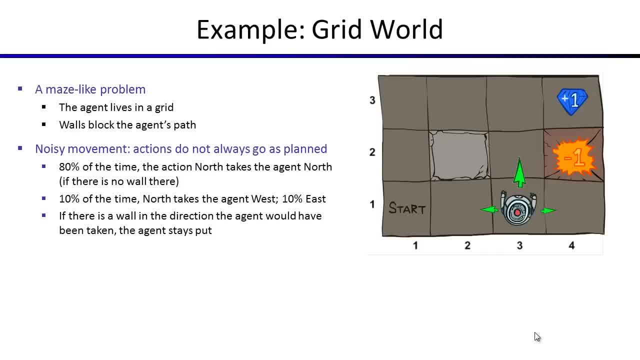 the time you'll go south. but going south means staying where you are. Okay, So we'll come to know and love this grid world. but you get the basic idea, You have directions, but sometimes your actions don't actually move you in that direction. 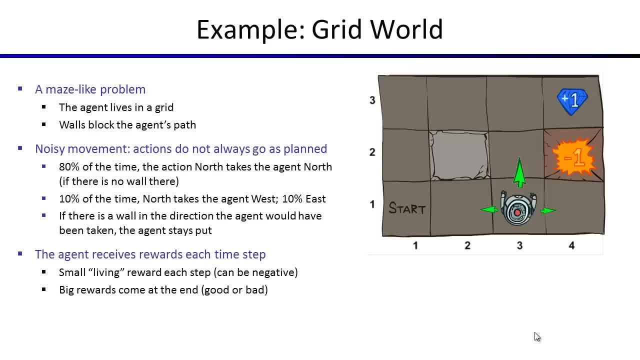 Now, of course, if you're in a grid world, you should have something you're trying to achieve right, And in a search we might have been trying to get the goal right, which might have been the closest dot or something like that in Pac-Man. 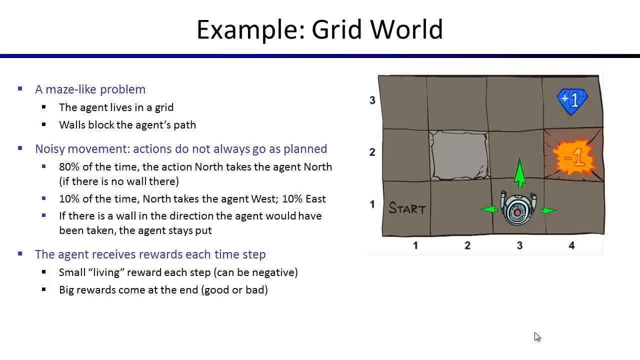 In this case, what you're trying to achieve involves rewards, which come at every step, and in this particular grid world, we're going to break rewards up into two kinds. There's a big reward that comes at the end of the game. 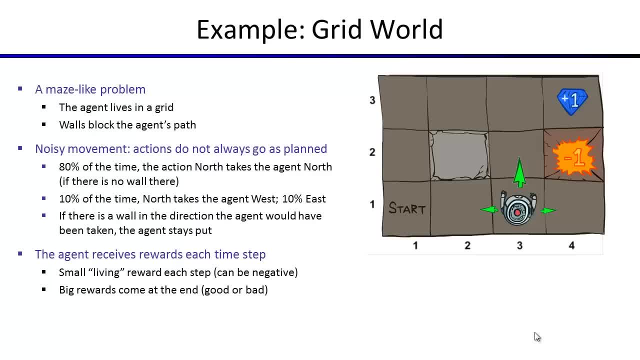 Okay. So in this particular case, if you get to the gem, you will receive a reward of plus one when you choose the action exit on that square. If you get to the fiery pit of death, then you'll get a minus one when you choose the. 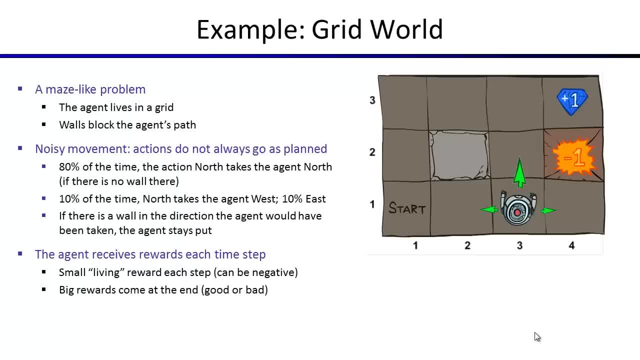 action, exit from that square. In addition to this big reward- positive or negative- at the end you also get a little reward that we'll call a living reward, at each step, and this could be positive or negative. This is a little bit of bonus or a little bit of cost that you incur every step. 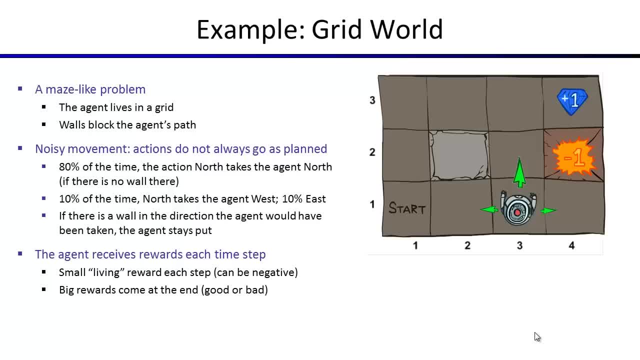 When you just take an arbitrary move. Now, there's nothing special about living rewards or a big reward at the end or anything like that. That's grid world. Other MVPs don't have that, but this is grid world here, and so basically, your goal is: 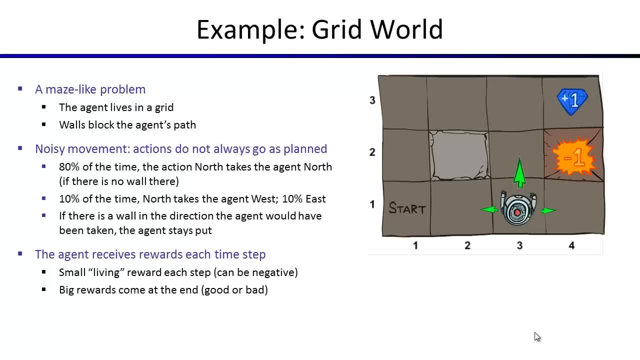 to move around right and you'd like to eventually get to that plus one in general, and you'd like to do it relatively quickly if you have a negative living reward, because kind of your bank account's ticking downward every time step and you'd like to avoid the fiery pit. 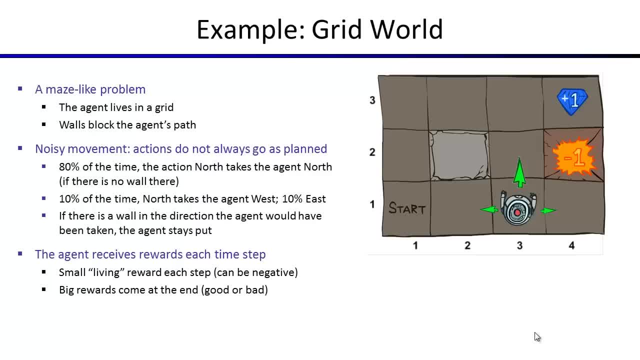 of death as you do it. So these are the kinds of things that this agent will be thinking about when it computes this action. So what's the goal? The goal is to maximize your sum of rewards. There's some fine print here. We'll come back to that. For now, just imagine that points are just like Pac-Man: they're score and plus one is a good score and minus .02 for a living reward is bad, and you'd like to get kind. 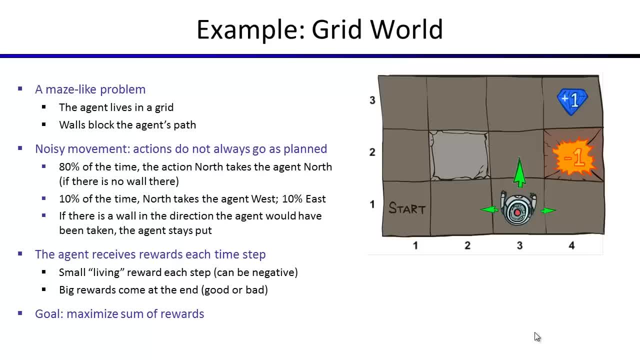 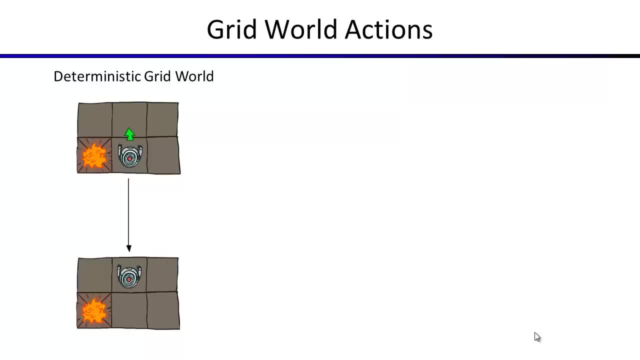 of the largest sum of rewards that you can. So in a deterministic grid world, which would be just a maze right, you have actions like go north and they have one result. The result is you are now one unit north on the grid. 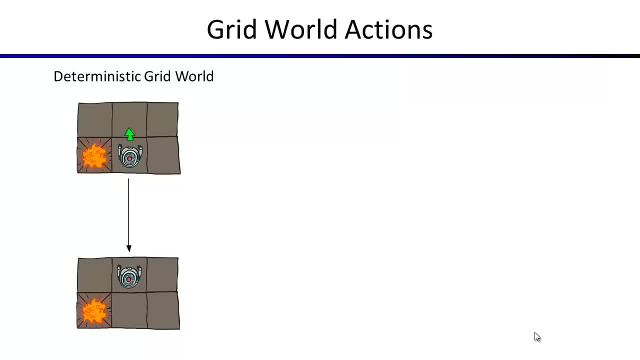 So actions are really simple and when we did search, this is how the actions worked right. You knew what your actions were, You knew exactly what they did, and we thought about a successor function which told you from your current state what successor states you can get to and you can pick among them. 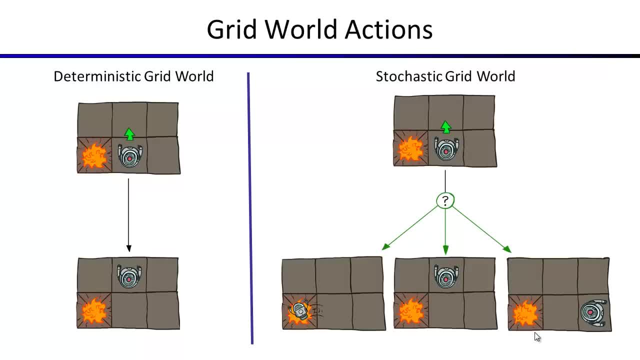 right. You can guarantee any of those successors In an MDP. you can think of this as just the same kind of thing, but with some noise in your actions. So you can still choose to take the action. You can choose to take the action north, but now you don't know what's going to happen. 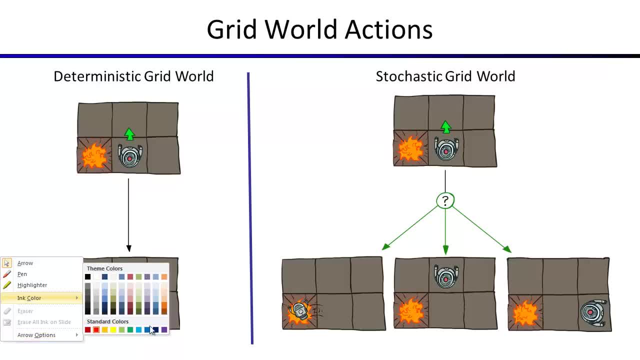 Probably, and according to these grid world rules that means kind of with any chance you will actually move north, but there's a 10% chance you'll actually end up slipping and moving right, and there's a 10% chance you'll end up slipping and moving left, which 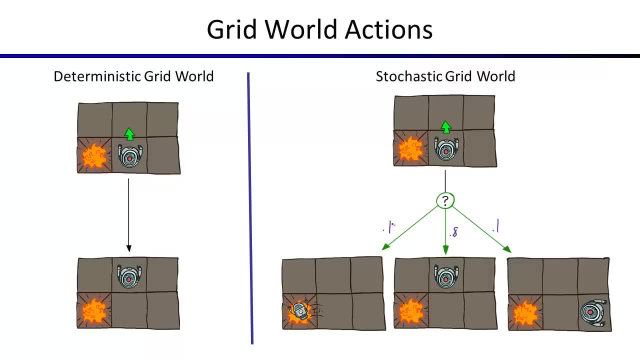 in this case is a fire credit deficit. okay, So it's still the same set of you saw this notion of states and actions, but now actions have multiple possible results and we're going to need to change our search formulation to kind of unpack that successor function in a way that lets us talk about what the 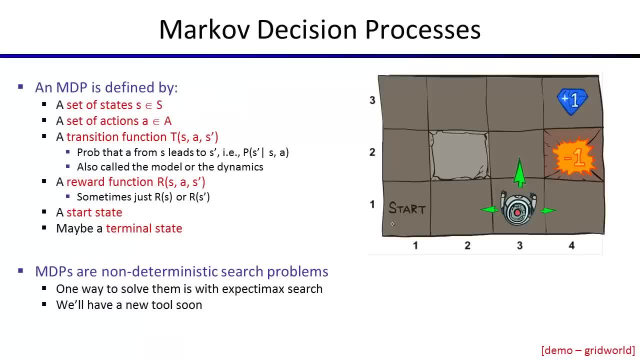 possible results are and how likely they are. Let's formally describe a Markov decision process. okay, So a Markov decision process formally is described by a set of states, just like search. So these states are just like the search states. 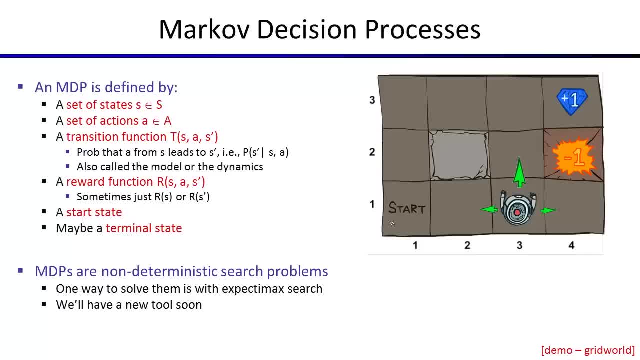 A set of actions, and these are just like search too, except we typically, in the formalization we just said, states have successors, But if you remember in your project one, each successor actually comes along with an action, which you'd need to, for example, compute the sequence of actions that constitute 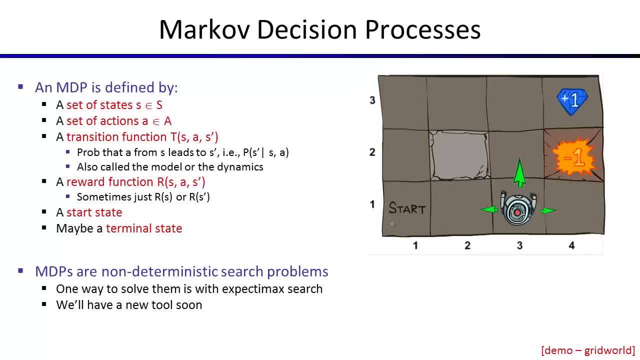 the solution. So we have states and actions, just like in search. Now all this other stuff is a little bit different. So all this stuff here is, in essence, the successor function, but unpacked with a lot of notation. and it's very important in this unit that we not go into symbol shock, because 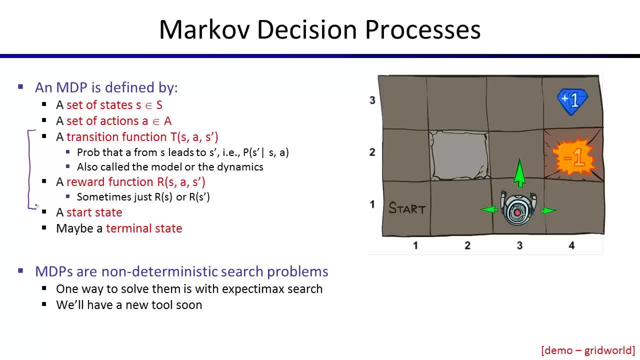 you're going to be seeing these same kinds of things: Transition functions and states and successors and actions. you're going to see these things over and, over and over again and it's very easy to kind of glaze over. But it's really important because we're going to be building on these concepts in the next. 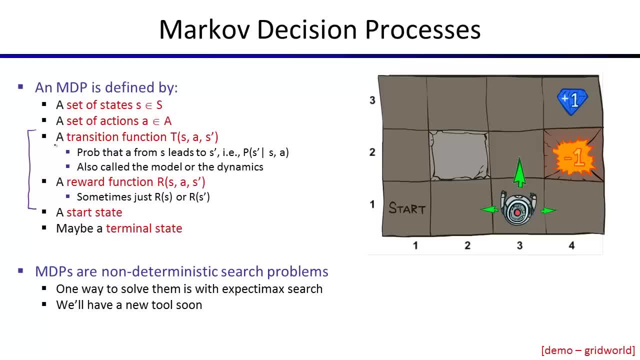 probably four lectures. Okay, so what does the successor function look like now? Well, there's now a transition function here. What a transition function says is: from state S, which is your current state, and choosing action A, which is under your control. there are multiple possible S functions. 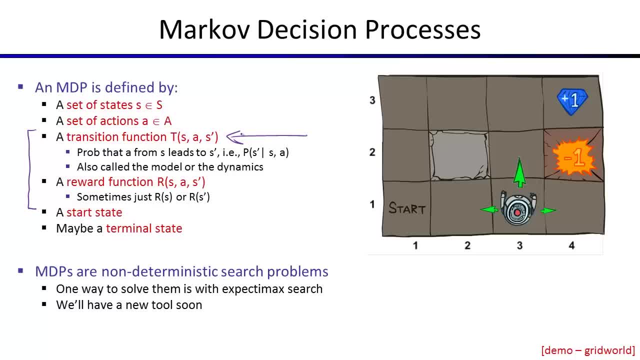 There are multiple S primes that could result In single-agent deterministic search. there was one possible result: S prime. Now there are lots, And so what we have is we have a function which tells us, for any S prime, how likely it is to result. 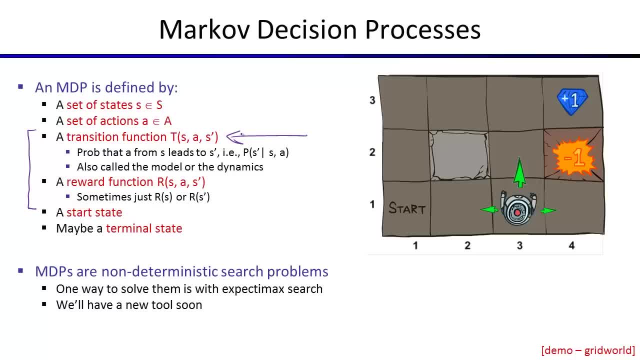 Okay, so you plug in an S, you plug in an A, That's your state and action pair, And then you can try lots of different S primes. Some of them will have probability zero. perhaps That means they can't happen. 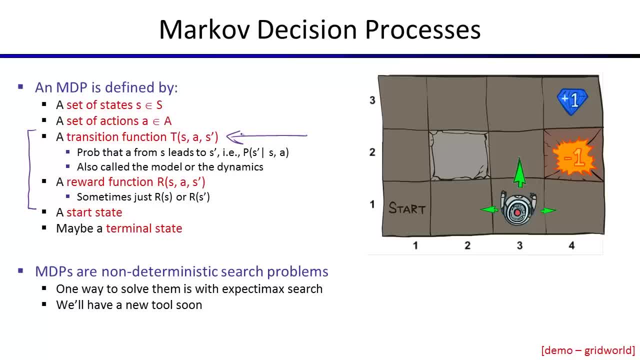 Other ones will have non-zero probability. That means they might happen, And if one of them has probability one, it means it's actually deterministic After all. So that's your transition function. Another way to think about TSAS prime is as a conditional probability. if this is clear, 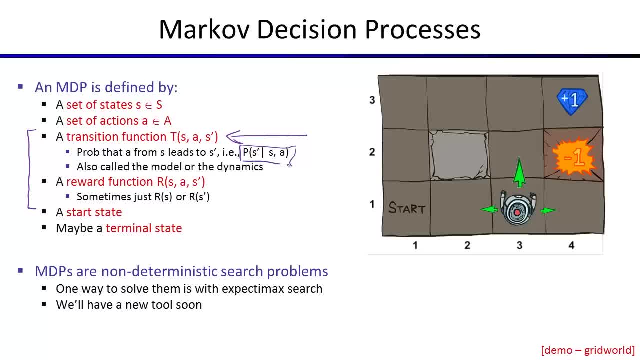 for some people. In other words, TSAS prime is the probability, given that you're in state S and take action A, that your result state will be S prime. So this is a distribution over S primes. All right, that's the transition function. 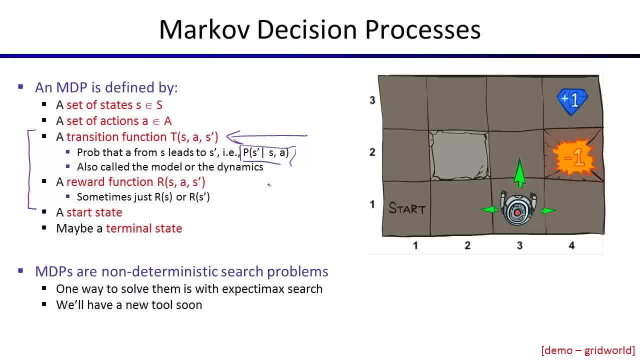 It tells you the things that might happen and how likely they are. Then you have a reward function In search. remember we have costs right, So each action had a cost associated with it. Well, now the cost is going to depend on what happens. 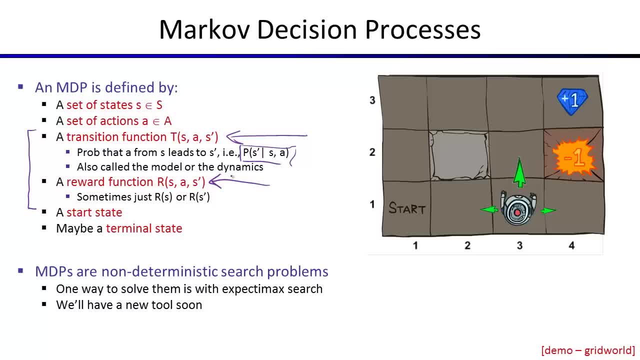 So, for example, in that last case where you might fall into the pit of death, maybe you want the cost to be high if you fall into the pit of death, but low if you don't. So you can't just say how much an action costs until you see what happens. 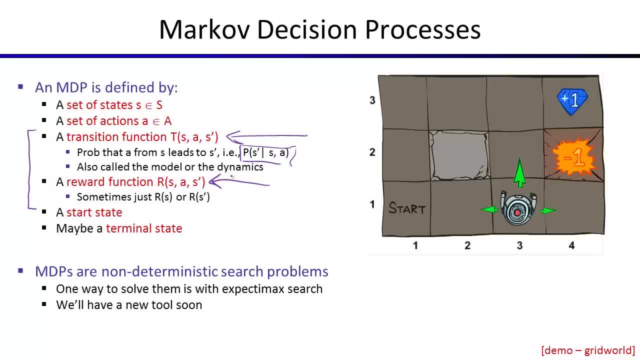 Therefore we have a cost function, or now it's called a reward function, which is R of SAS prime. This says, if you're in state S and you take action A and the outcome that comes out of that happens is S prime, how many points will you get? 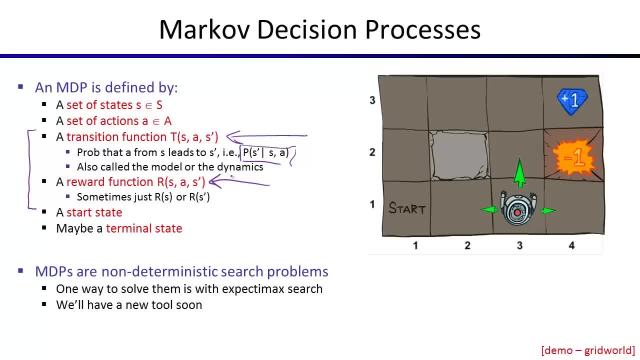 Costs in search were bad. You always wanted to minimize costs, But now we're in this framework of maximizing expected utilities, And so rewards are essentially negative costs. Rewards are good. So instead of minimizing costs, we maximize rewards, And so the sign has changed. 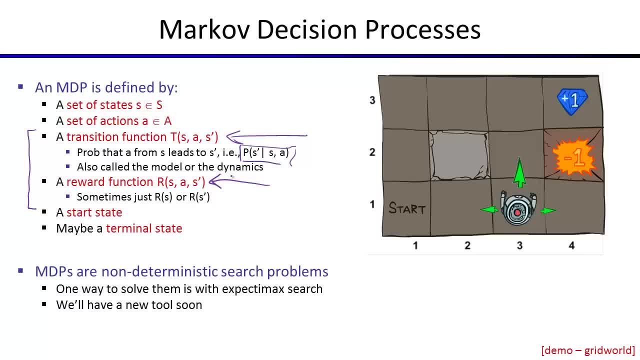 But the reward function is really just the cost function in disguise States actions. transition function tells you what might happen And the reward function tells you how much it will cost if it does happen. Typically then there's a start state And sometimes there's a terminal state. 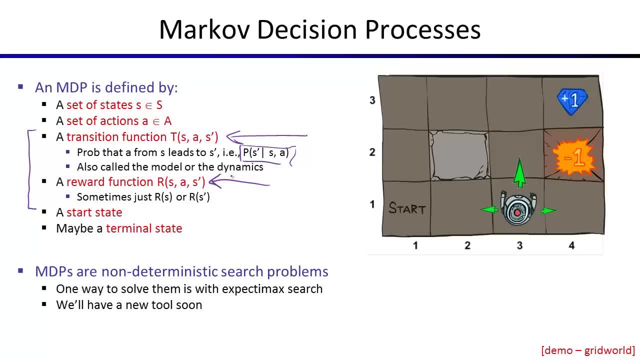 A lot of the math works out nicely when there's a terminal state, But there doesn't have to be one. So, for example, in grid world, we might imagine that there's an extra state that you don't see called. done Like that there. 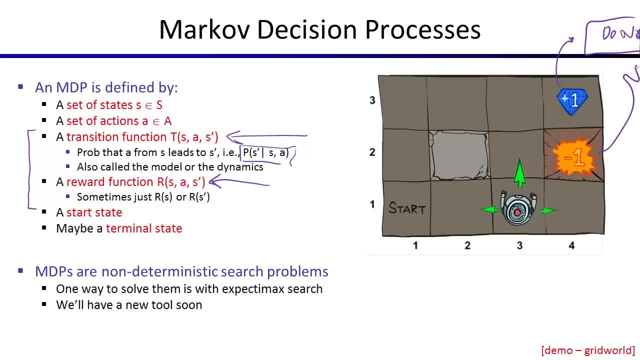 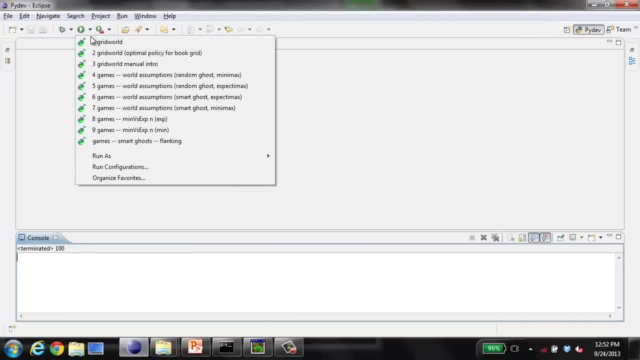 And done, kind of goes out there. You get there from the states. that end the game. OK, All right. So MDPs are essentially non-deterministic search points. Let's see one in action, All right. So this is that same grid. 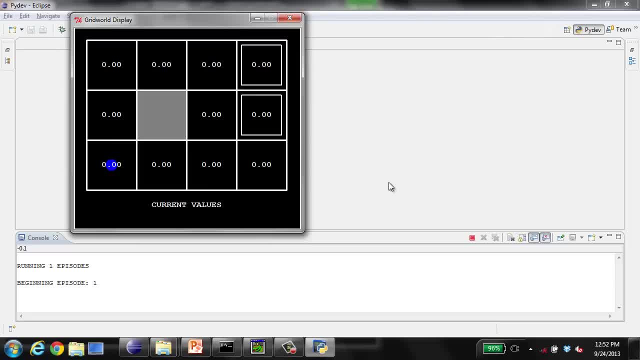 And you can ignore the zeros for now. For now, just black means it's a square I can traverse, Gray means it's a wall, so I can't move into that square. And the double squares are these special states? They're not actually terminal states. 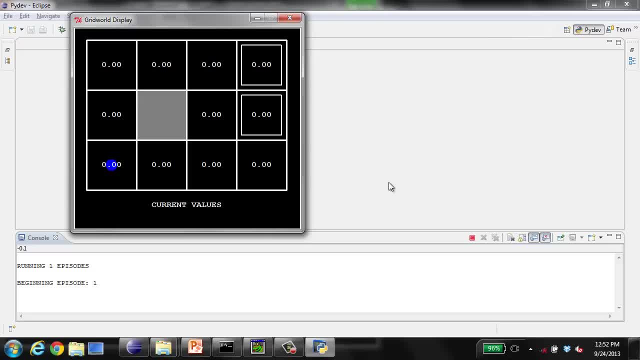 They're states from which you have only one action available. That action is called exit And when you take it you're guaranteed to go to the terminal state. That's a little bit weird but it helps with the bookkeeping if you try to work. an example: 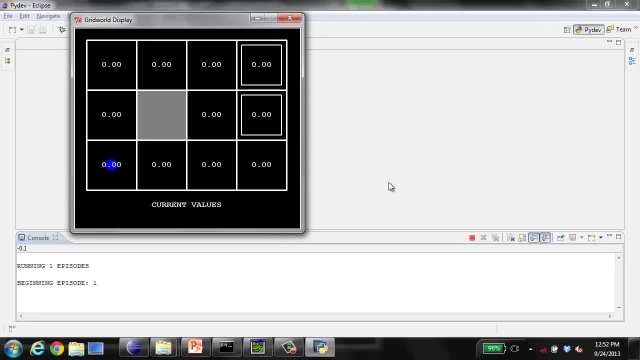 by hand. All right, So at the moment I've done nothing And my robot, who's now a blue dot, is in the lower left. What I'm going to do is I'm going to try to get to the upper right corner and get that. 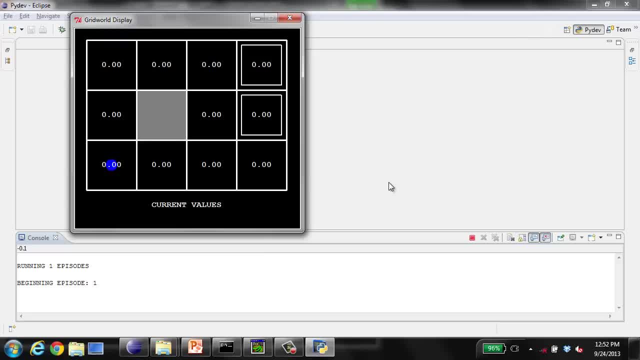 plus 1.. And as I go, every time step, I'm going to receive a reward of minus 0.1.. So it's a cost. So what I'm going to do? how should I get there? I'm going to go east. 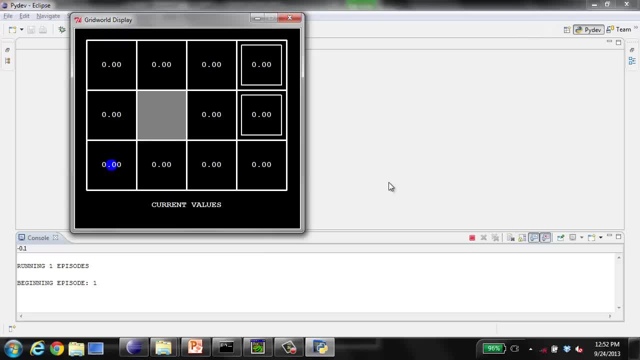 So I'm going to press the east key on my keyboard, which is the right key, And I don't actually know what will happen. Probably it will move east. OK, so it did, Actually. let's look down here at the text output. 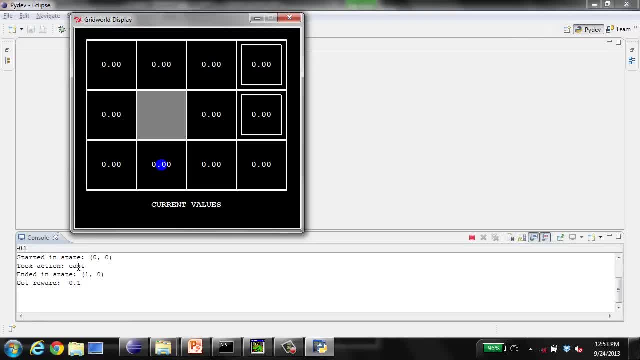 It says I started in 0, 0.. That's right. I took the action east, That's right. And I ended in state 1, 0.. OK, great, And I got the reward: negative 0.1.. 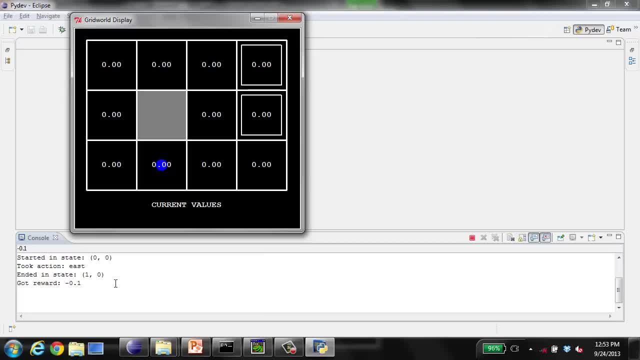 So that's my starting state, my action and my ending state. Other ending states are possible, but that's the one I got this time, And then I got a reward along with it, So that's going to be really important. Every one of these transitions is a state, an action, a resulting state and a reward. 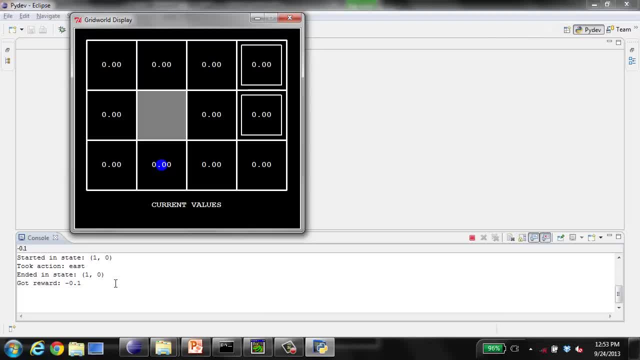 So I'm going to do it again. I'm going to press the east key. We'll see what happens. OK, So it says: started in state 1, 0, took action east. ended in state 1, 0, got reward minus. 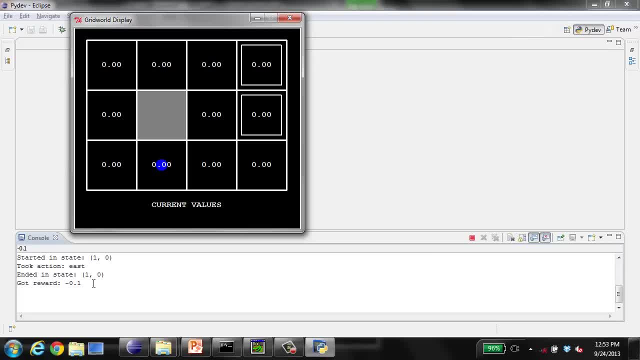 0.1.. So why didn't I move? Well, because 20% of the time you don't actually go east. You either go north or south And, according to grid rules, if either of those happens, you stay put. 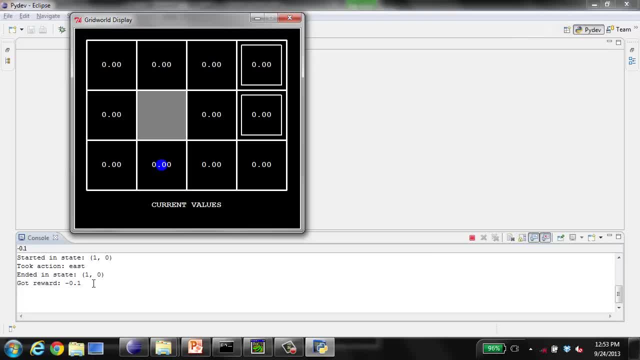 Right, Because you can't go north or south. All right, So I got unlucky. I'm going to try east again. OK, Unexpected, But I you know it can happen. OK, I pressed east again And now I finally move over into the square. 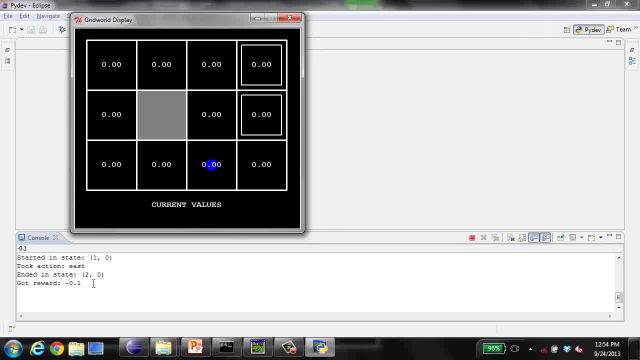 You can see, it's kind of annoying being in a grid world like this, because not everything that you try works out, But now I'm going to try to move north. OK, Now you've got to cross your fingers as we pass the pit of death. 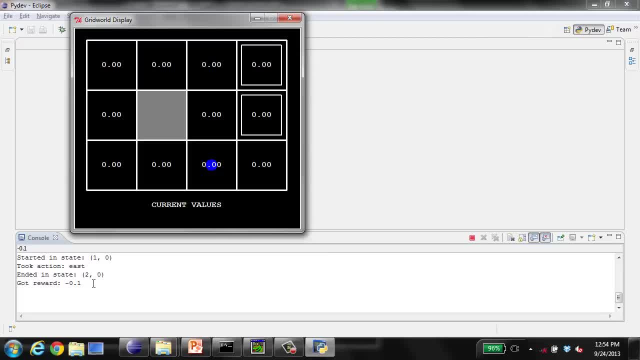 I'm going to try north. OK, That worked. OK, I'm going to try north again. Something bad could happen here, Right, I could fall into the pit, OK, And that's that. Let's do that again. Lies. 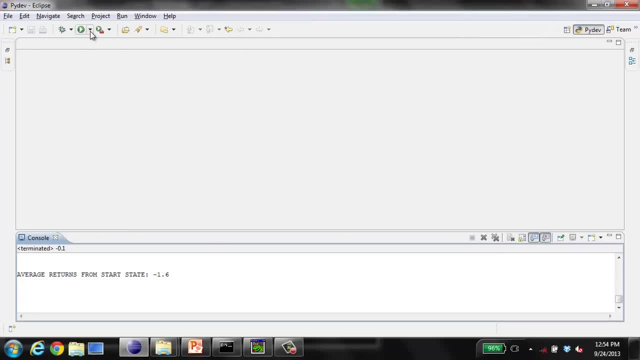 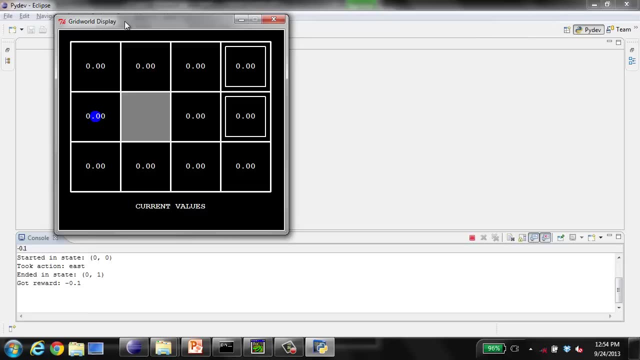 OK, I'm going to try north again. Something bad could happen here. Right, I could fall into the pit. OK, And that's that. I have demos. OK, Let's go. Let's try it again East. What should I do now? 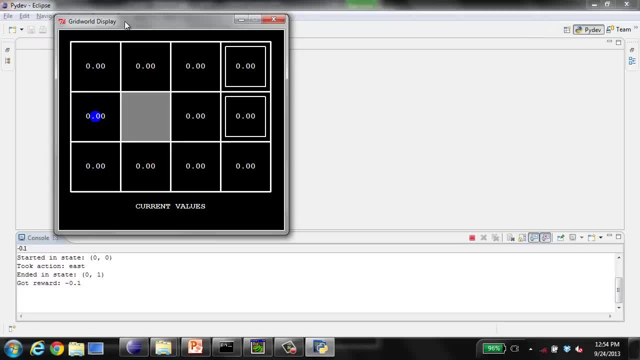 Let's just, We had maybe We had wanted to go east, But now that we're here, probably a better policy is to try to go north. So I'm going to try to go north. OK, Good, Now I'm going to go east again. 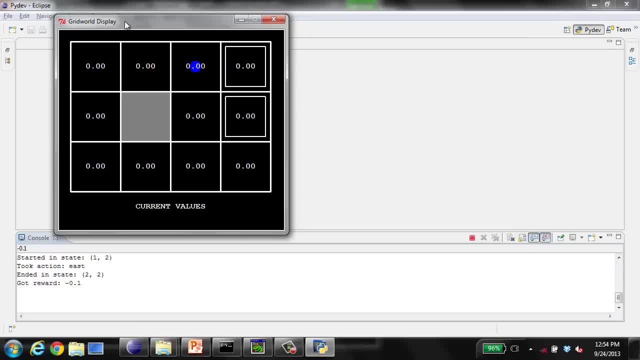 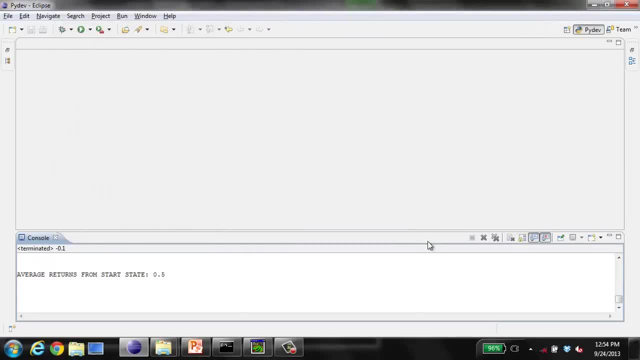 East, East. I'm going to go east again, Hopefully, Good, OK, So I went into that east square. I'm going to now choose the action exit and receive my plus one, OK, So. So I'm working on the text. 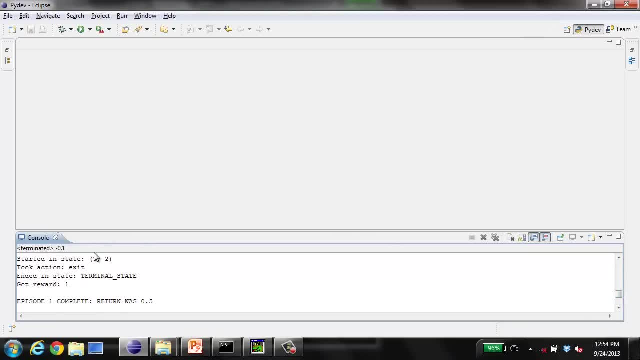 It says. It says that I went from 3-2.. I took the action exit. I ended in terminal state. I got my reward of plus one And my return, meaning the sum of my rewards, was 0.5.. 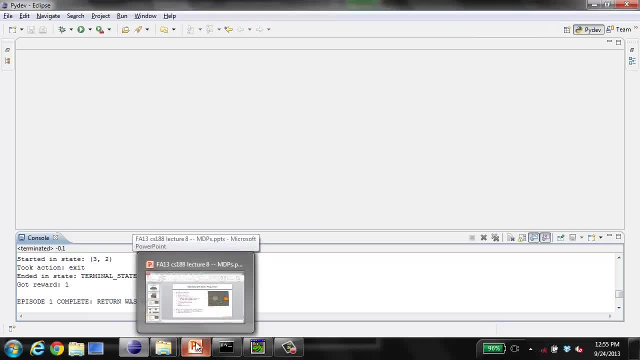 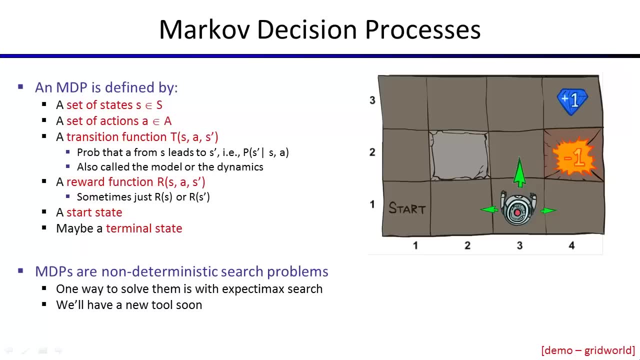 So it was plus one, But I lost. You know, every time step I lost a little bit. That's the way grid world works. OK, So you can see, things don't always go as expected. It's always exciting in grid world. 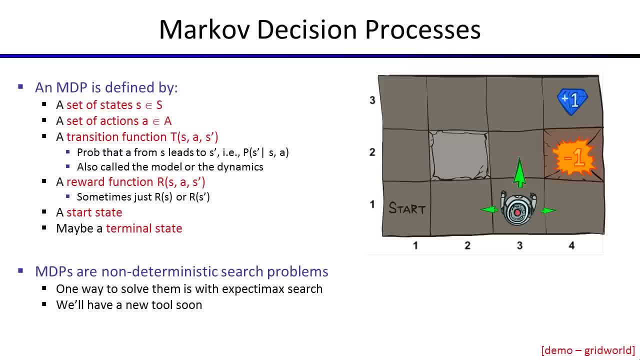 And that's because this is a non-deterministic search problem. Now the question is: since you don't know what's going to happen, what does it even mean to solve these things? Well, first of all, you don't come up with a plan anymore. 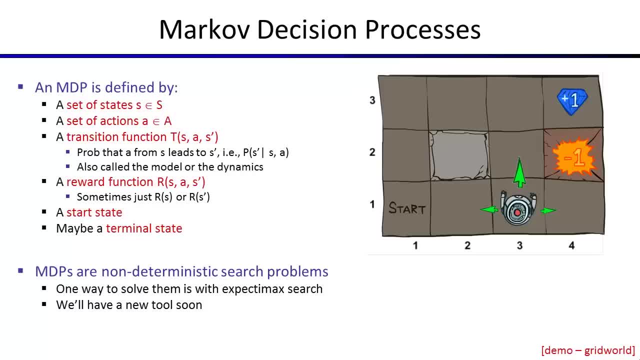 So we'll talk about what you do, But it's actually more like what we had for Expectamax Right, And so if you think that what this agent should do in this context is do an Expectamax search where all of the uncertainty in the action resolution is treated as a chance node, you're 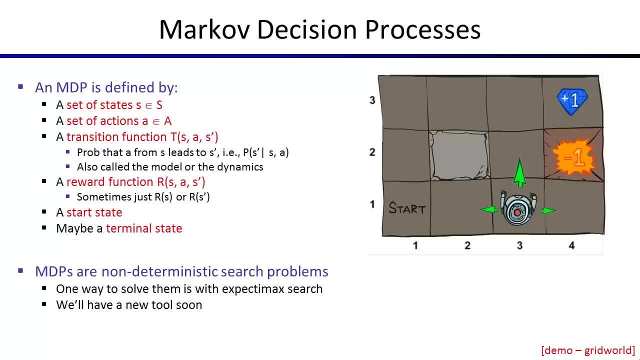 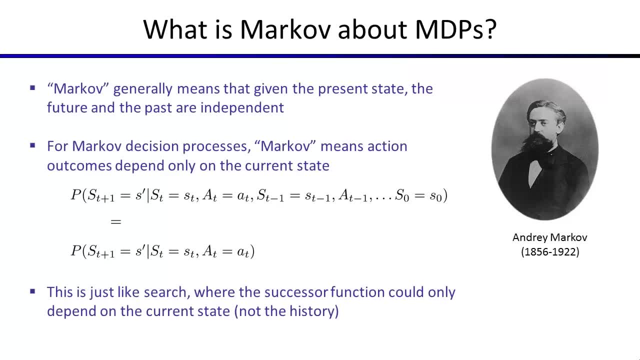 actually 90% of the way to solving MDPs. We'll have a new tool soon, But for now, one way to solve these things is with Expectamax. OK, So this is Markov guy, And why is he in our search problem? 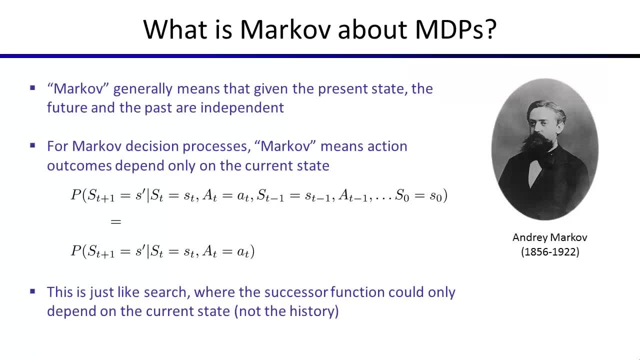 So whenever we say Markov in this class or really in any setting where we're talking about probabilities and things like that, Markov means that, given some present state or information, the future and past are independent. OK, What does that mean? 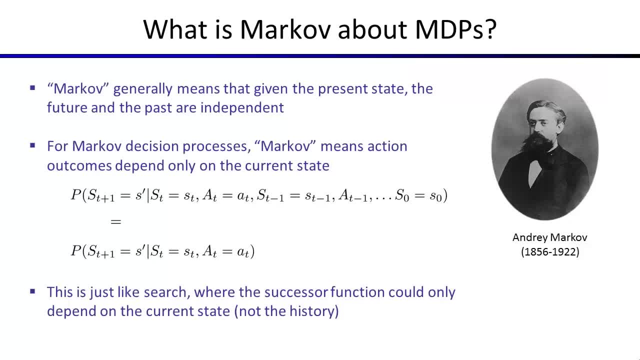 In the case of a Markov decision process. Markov means that the action outcomes. that is what state you'll end up in when you take this action. of course, it depends on your current state. Whether you fall into the pit of death depends on whether you're next to one. 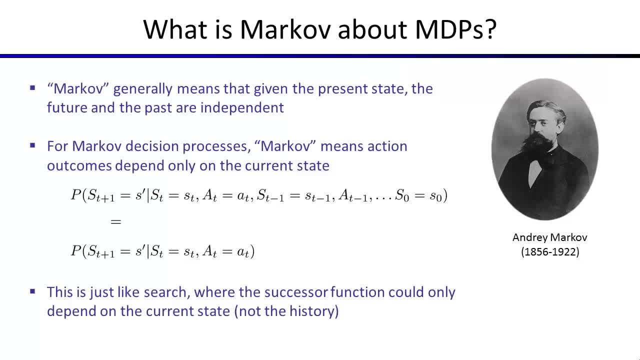 Right, But it also depends on your action, Right. Some actions are riskier than others in a grid world, And so, of course, the outcome, the S prime you land in, depends on your state and action. The question is: does it depend on things that have gone before? 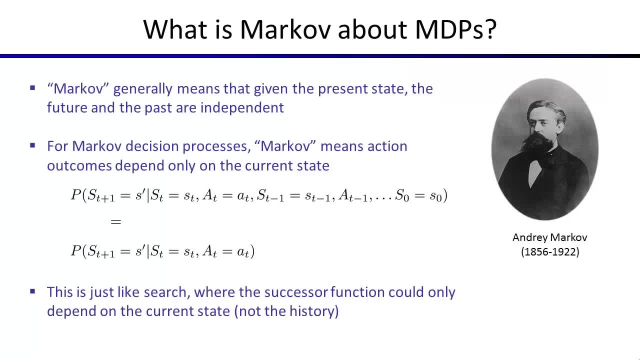 Or is your current state and action enough to completely determine the distribution, though not the outcome, of your transition? OK, Markov, here, if it's a Markov decision process, that means you're guaranteed that this giant conditional probability, which, formally, the S prime you end up in, is going to be the 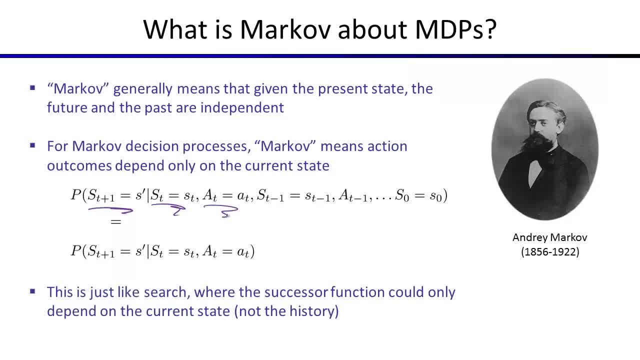 outcome. The S prime you end up in in principle could depend on where you are, the action you've taken and everything that came before that in this episode, But we're guaranteed that it only depends on the current state and action. 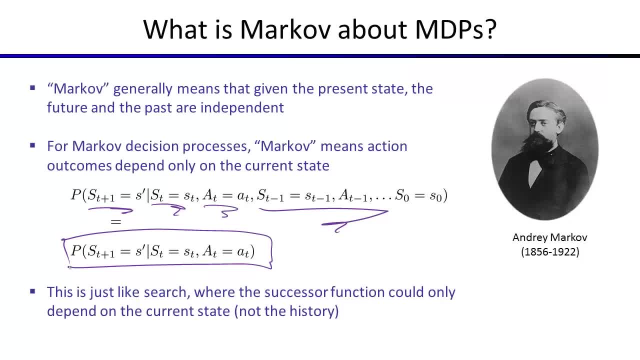 That's what Markov gives us Right. The future, which is S prime, is independent of the past, which is all these t minus ones given the present. We actually have seen this before. We saw this with search. So in search, you had a successor function and it depended on your state. 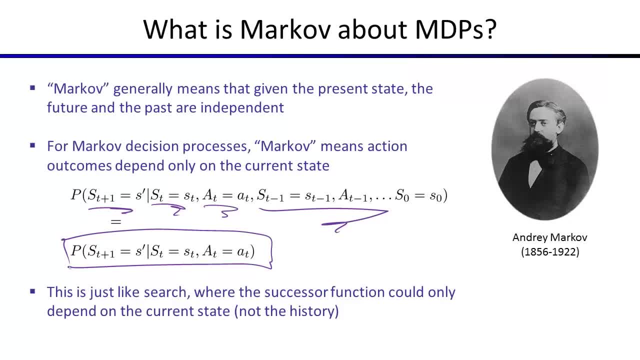 So the successors and the costs all depended on your state, But they didn't depend on your previous state. Your state somehow had to pack in all the information necessary to let the successor function do its job. And when you had problems in your homework or, as you'll see, on exams, where you formulate 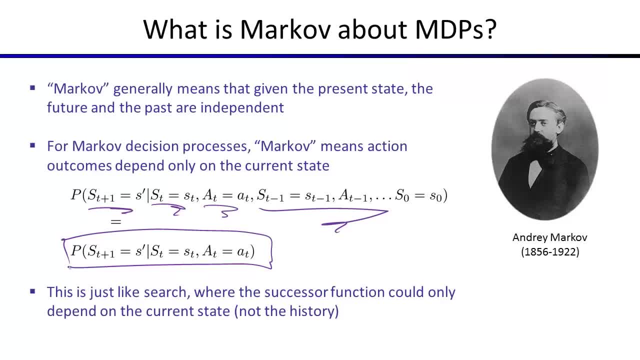 a search problem, then you need to make sure the state encodes enough information to admit the successor function, because your history is gone, Right, You don't keep your histories around. Same thing with MDPs. The state needs to support the successor function. 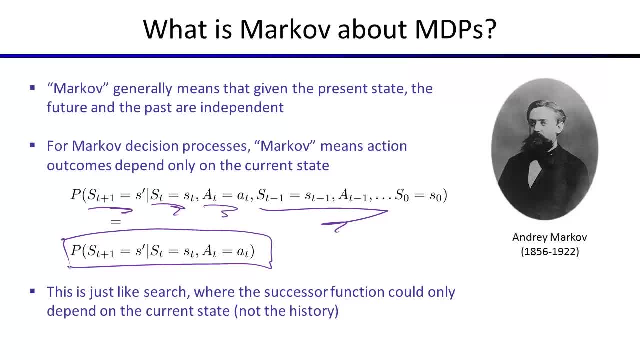 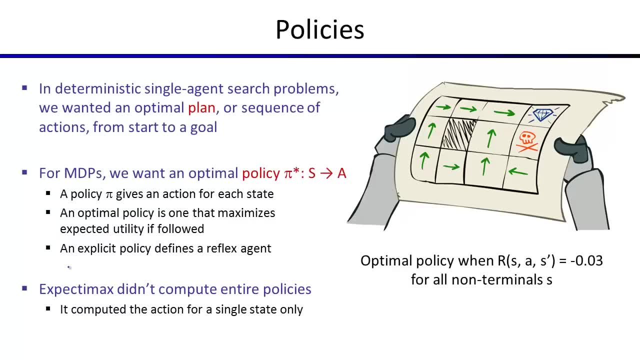 Now that means these conditional probabilities. OK, Bye-bye Markov. We'll see Markov again when we talk about hidden Markov models. OK, So in single-agent deterministic search problems, we wanted a plan That was a sequence of actions that take your start state and turn it into a goal state. 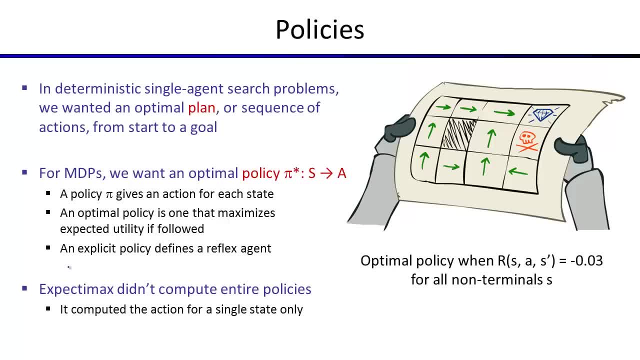 That's totally off. That's totally off for MDPs, As we saw. you can plan to go east, but who knows what's going to happen? You might go north. You might end up in the pit of death, Right. 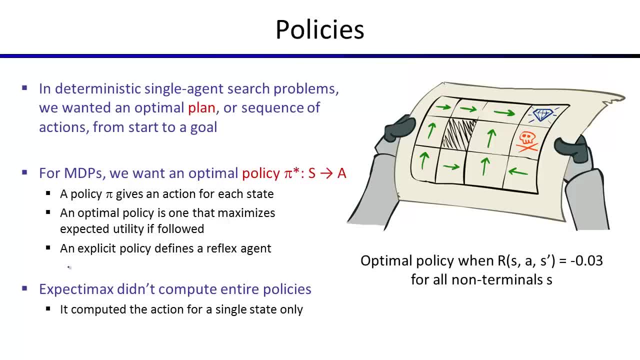 And so we can't have a plan. What we can have instead is what's called a policy, And a policy- as we saw with games- is a recommendation function. It takes your state and it tells you what to do. Right, 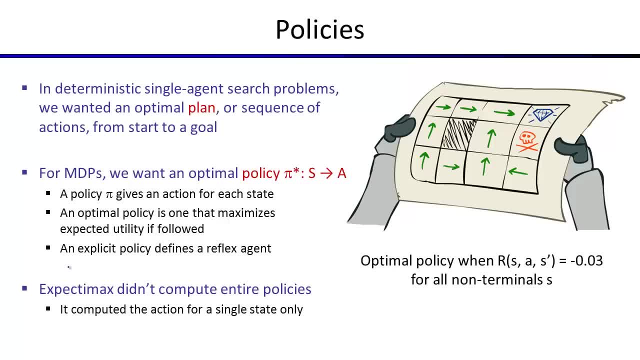 And so here you can see this treasure map that this robot agent is holding. That's a policy for this grid world we've been seeing, and it's a policy that's appropriate for a certain setting of the grid world, certain probabilities, certain living reward. 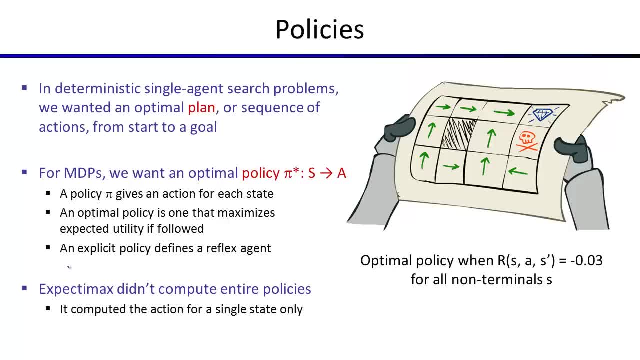 In this case, this is where every step you lose .03 of a point Right. And so it says: if you're in this square, move north, or rather, take the action north. If you're in this square, take the action east, and so on. 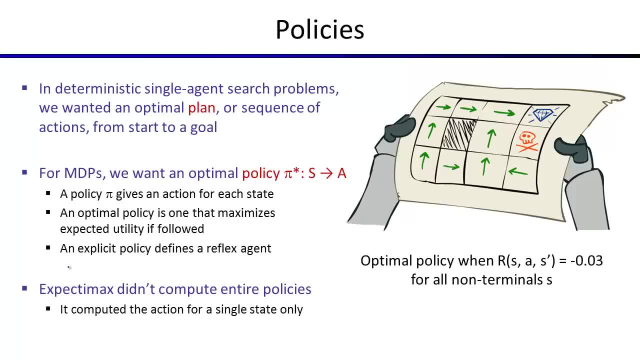 OK, So a policy gives an action for each state, which means explicitly: if you wrote down a policy, you'd have a lookup table: Right State action, state action, state action. And that, of course, would be a reflex agent if you did it. 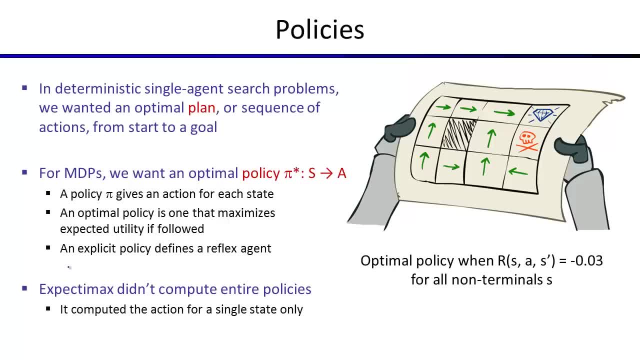 Typically you don't do that in large-scale problems because there are just so many states And so very often your policy is implicit And your policy is: when you land in a state, run, expect max and do what it tells you. 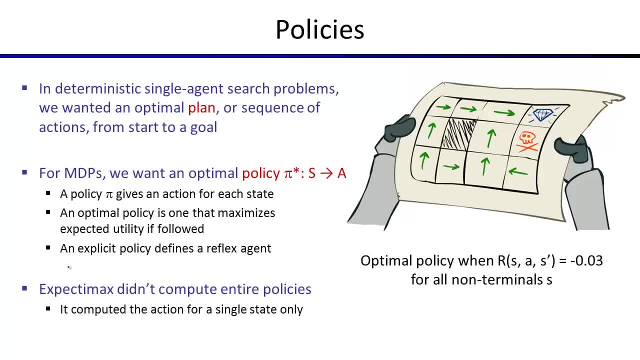 That's an implicit policy as opposed to a giant lookup table. Some policies are better than others. Obviously, a policy that always tells you to jump in the pit isn't a very good policy, And so we have a notion of not just a policy being a lookup table, but there being better. 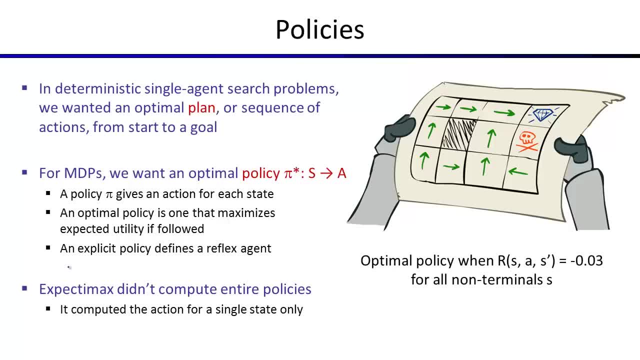 policies and worse policies. In particular, we want an optimal policy. An optimal policy is one that gives us the maximum expected utility of follow. Why does it say maximum expected utility? Why can't we just talk about the points you'll get if you follow a policy? 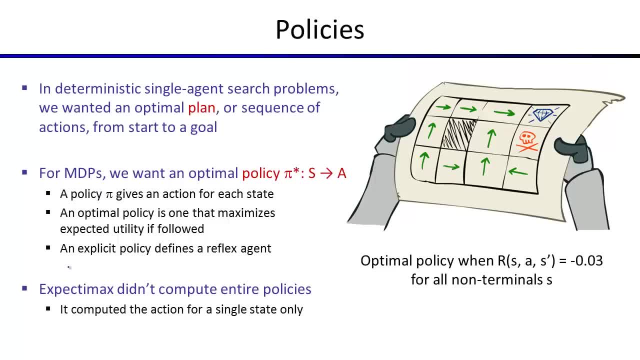 Because you can still be unlucky, Right, And you might still have terrible luck- like apparently I do with demos today, Right, And so the policy can't tell you how many points you're going to get. What you can say is: you can say: if I follow this policy on average or in expectation? 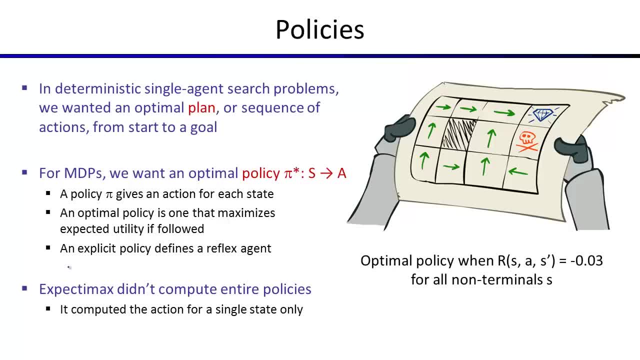 here's the expected sum of rewards that I'll get, And so we're always now talking about, not sums of costs In the world of search. it was easy: You take your plan, you add up the 12 numbers and that's your cost of your plan. 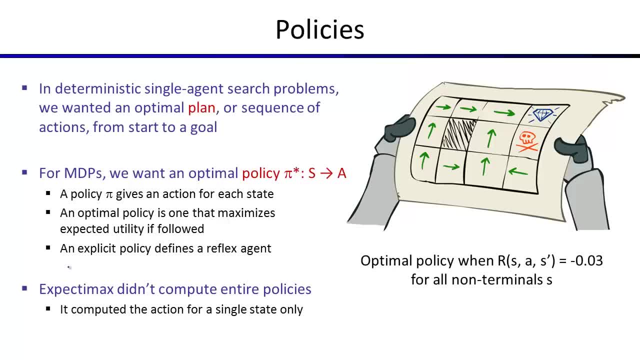 Now, with MDPs, you have a policy, And so even thinking about how much it's going to cost involves thinking about many possible outcomes and taking sums over those outcomes. So even simple things like evaluating a policy are now a little harder. 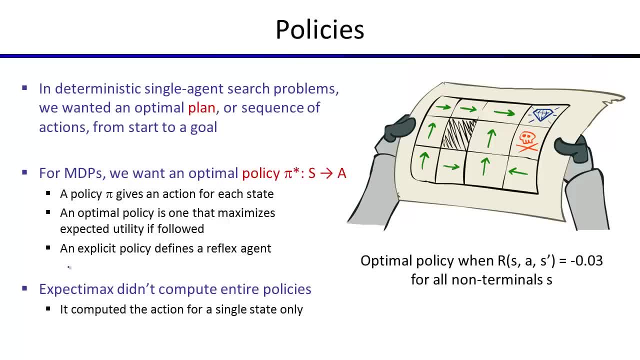 Okay. What's this have to do with Expectamax, which I've said a couple times? Expectamax did not compute policies. When I run an Expectamax search, what happens? I start doing a kind of Project 2-style search from a state. 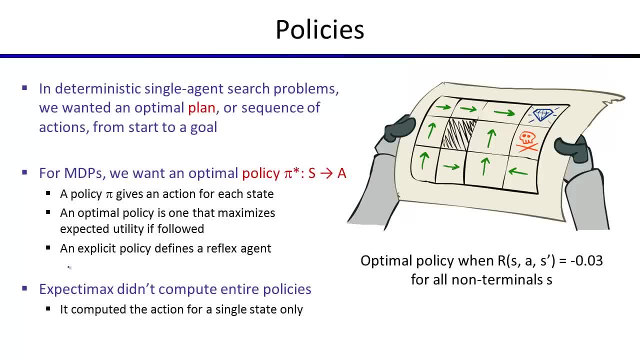 And of course I think about the future and there's an evaluation function and all that stuff. And at some point what does Expectamax return? It returns an action. It says the Expectamax value of the route is this and you should go left. 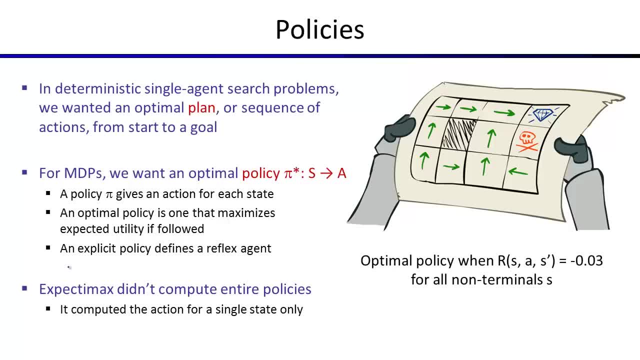 A policy would be a whole list of these things. So when you run Expectamax you're not computing a policy, You're computing one entry of a policy function. So if you wanted to compute a whole policy, you'd do a whole lot of Expectamax. 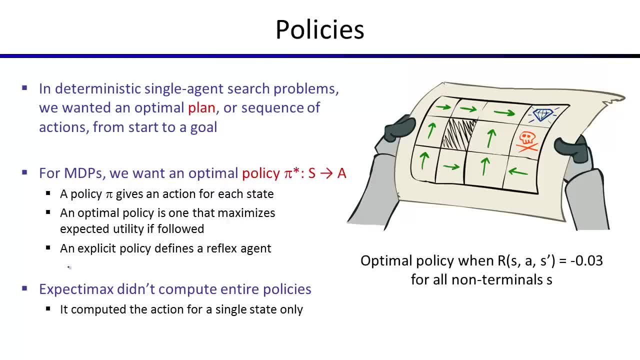 That's not going to be practical. Any questions on these basic ideas, MDPs, non-deterministic actions policies, this kind of stuff. Okay, We're going to be building on these a lot. Let's take a look at some optimal policies for GridWorld. 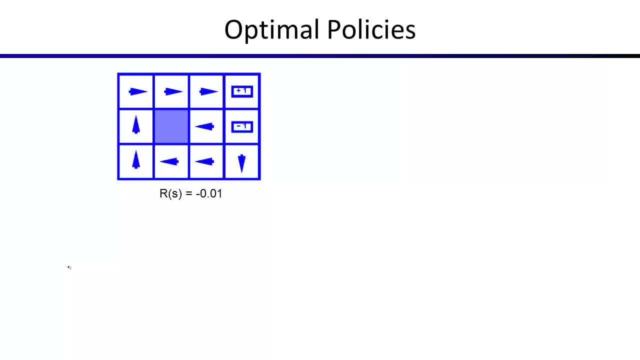 Okay. So this is a GridWorld with 80% success rate, 10% left or right, And this is a GridWorld where it's plus one and minus one at the gem and the pit of death, And also there's a living reward that's going to vary. 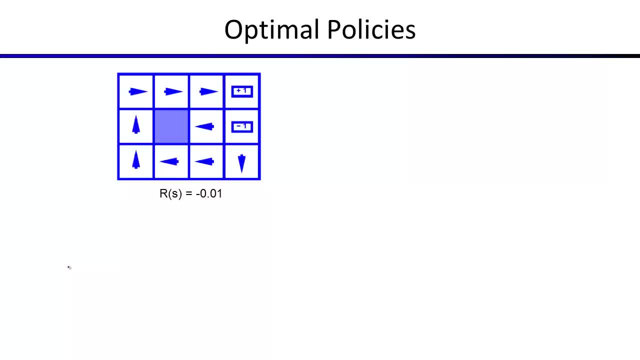 So this particular GridWorld is the one where the living reward is minus .01.. So a very small penalty each time step. Why does the time step penalty matter? Because it affects things like whether or not you're willing to take the long way around. 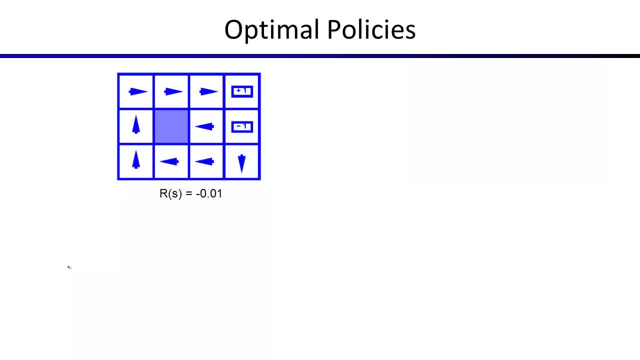 If there's heavy penalties, you might not be willing to take that step. You might not be willing to take the time because time costs you. Okay, Let's take a look at this one. So the living reward is very. The living penalty here is very small. 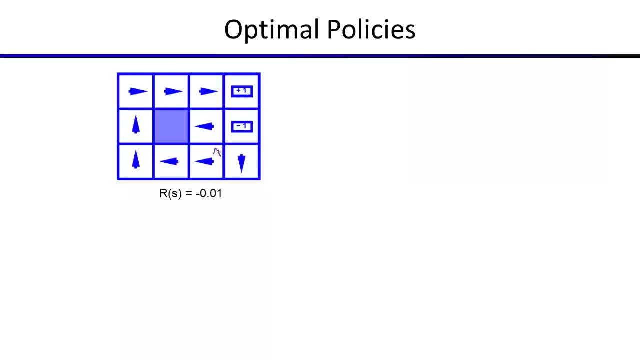 And so let's look at what this policy says. It says: if you're in square A here, what should you do? You should go west, Right, That's not the shortest path. The shortest path is kind of to go head up this way. 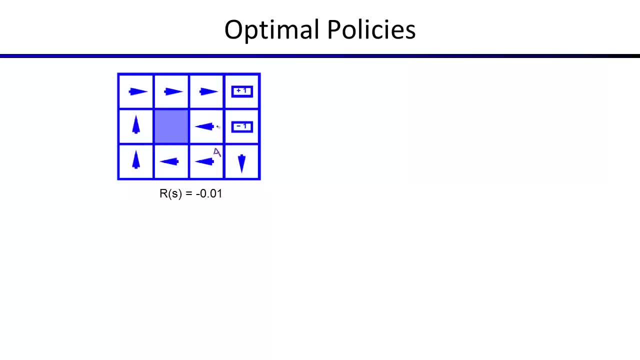 Right, Why is it saying to go all the way around clockwise in order to get to the plus one? Right, This is safe. You've got a 10% chance of falling into any pit you want, And here you just do a couple extra moves and you're kind of completely pit free. 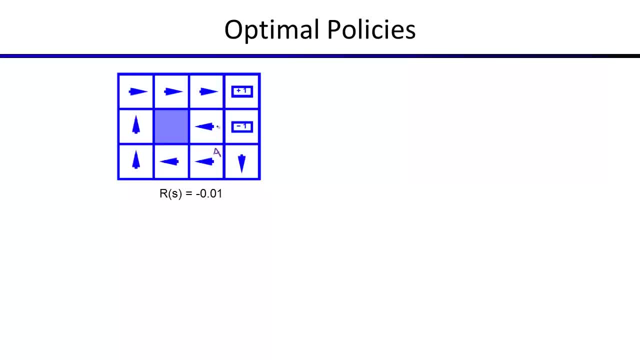 Okay, So that makes sense. A is west. Now what if you're in B? Remember, the policy has to tell you what to do from every state, And from B it says: move west. What's west of you? 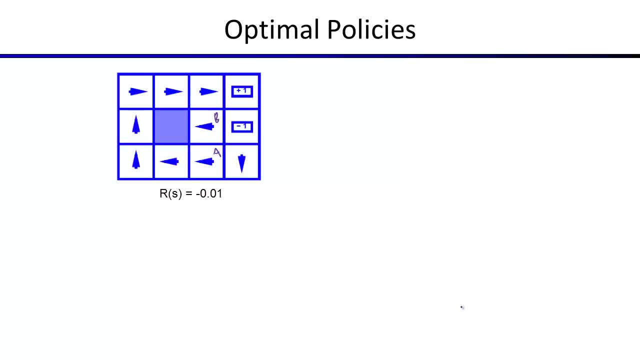 The wall. So what's going to probably happen if you move west? Nothing. So what is? Did it break? Did we compute the policy wrong? Why is the recommendation to move West? Yeah Right, If you move west, probably you'll stay put. 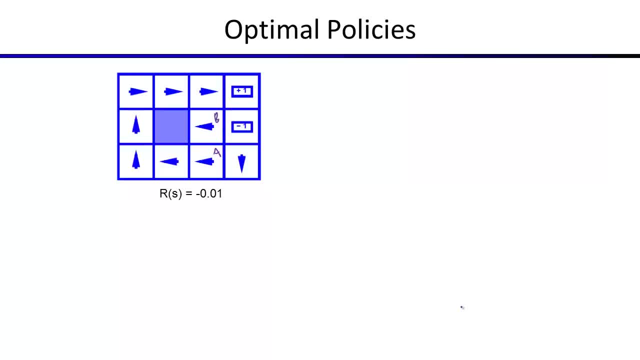 But with 10% chance you'll either move north or south And there is no risk of falling into the pit. This is like the robot pressing up against the ledge and just kind of shimmying left and right. That's what's going on with this wall. 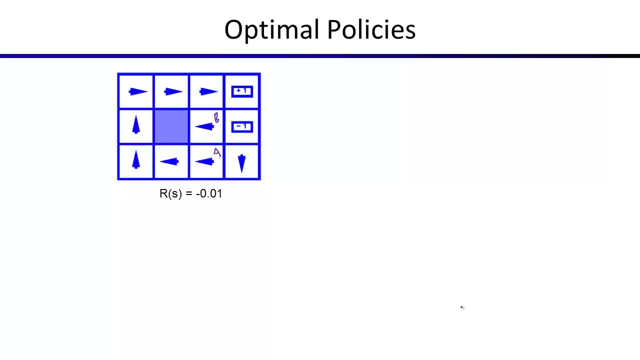 And so you're willing to, like, spend some time, probably not making progress, to get rid of the risk of falling into the pit, And whether or not you slip north or south doesn't really matter. From that point forward, you're pretty safe. 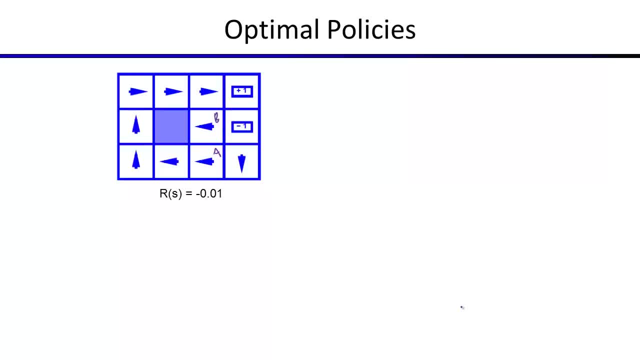 Okay, So we're going to move west, We're going to move north. We're going to move south. We're going to move north. We're going to move east. We're going to move north, We're going to move west. 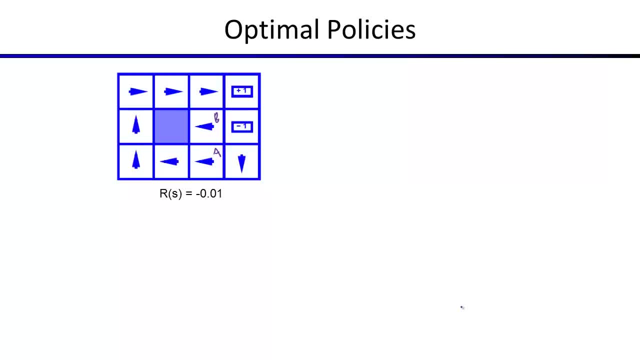 We're going to move west. We're going to move west, So we're going to move north. We're going to move west And we're going to move west, So we're going to move north, And then we have a little bit of a risk of falling into the pit. 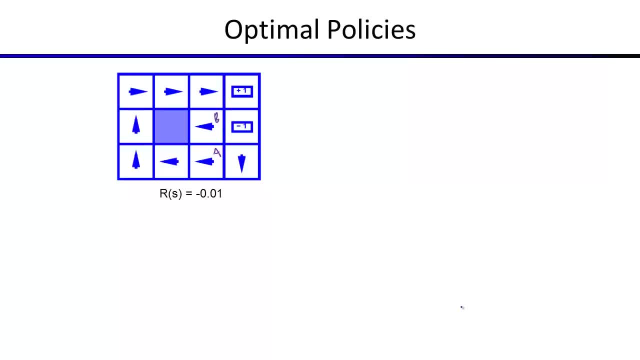 And whether or not you slip north or south doesn't really matter. From that point forward, you're pretty safe. Okay, So the reason why you're willing to go a long way and you're willing to kind of press yourself up into the wall and wiggle around until you happen to escape safely is because 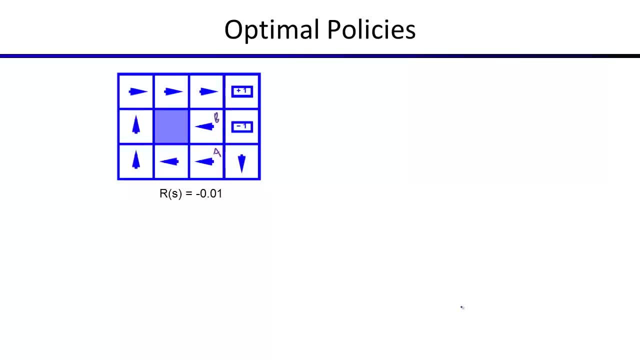 you have basically all the time in the world. The living penalty is very small. What happens if I change the reward? Well, as we know, we change the utility function and the behavior is supposed to change. The computations don't change, but the behavior should change. 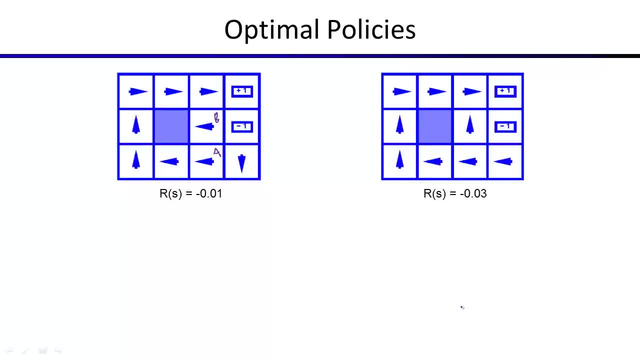 Okay, so here's a living reward that's slightly more painful. So what happens a day? Don't go the long way around. You no longer play that shimmy against the wall until you finally slip right And that kind of makes sense. It takes a long time before you actually move. That's pretty expensive. 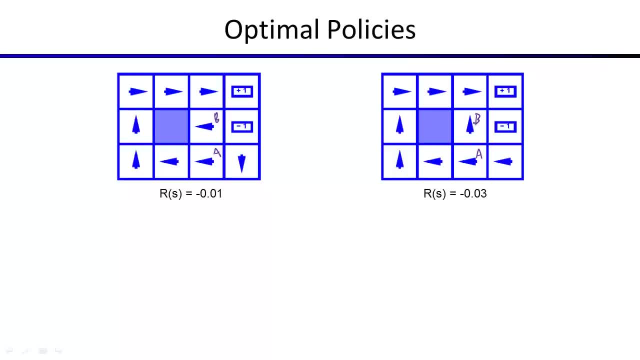 And so here you're not going to do that. Let's crank up the cost of each time step again and make the living reward even smaller. So here's minus 0.4.. Let's look at the behavior. What happens here? So at A it says: take the shortest path right, Maybe you'll fall in the pit. 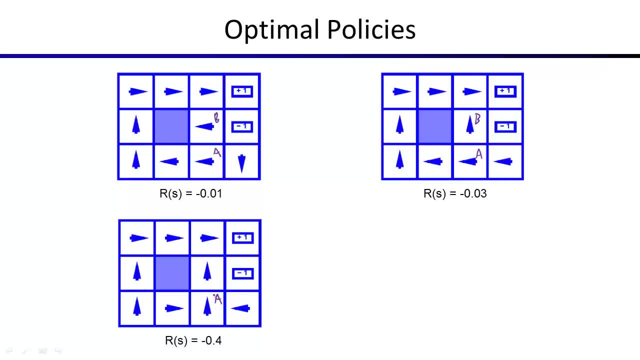 But it's just, we don't. it's too painful to go the long way around. In fact, even here at C now, you don't want to go the long way around, You just want to kind of go and as few time steps as possible, and there's some 10% risk of a minus one. 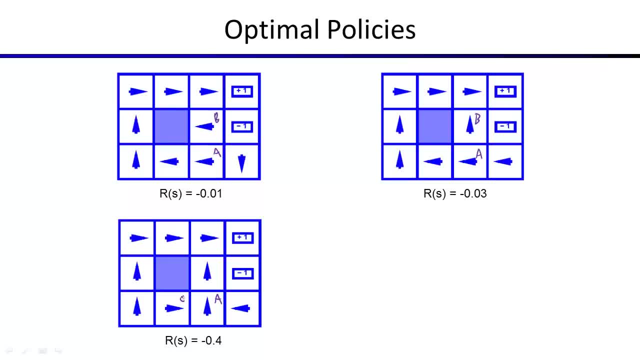 But really, 10% risk of a minus one isn't so bad when you're losing 0.4 every time step Okay, and so, of course, from B You're going to move straight north. All right, what happens if I crank up the living reward to like minus two? 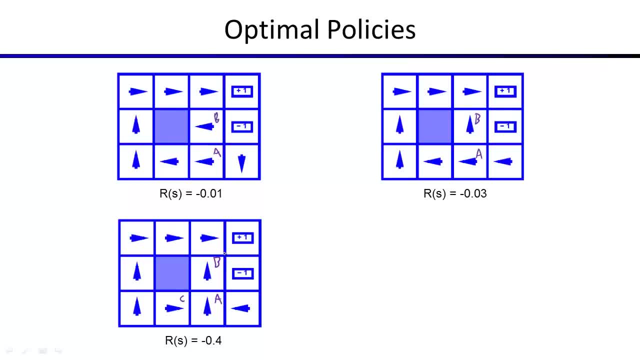 What do you think will happen? What do you think? So at minus two, right? Yeah, you want the plus one, You don't want the minus one, but really you don't want the minus two. So you just like basically run for the nearest exit, right? 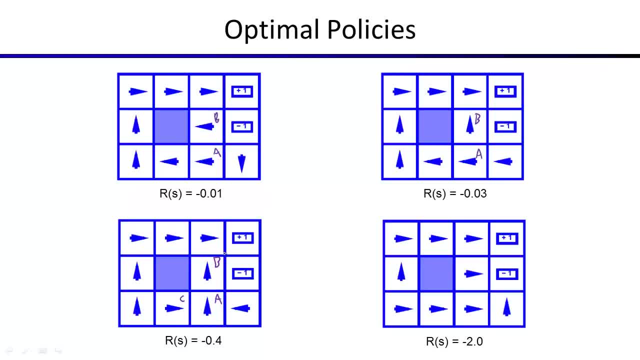 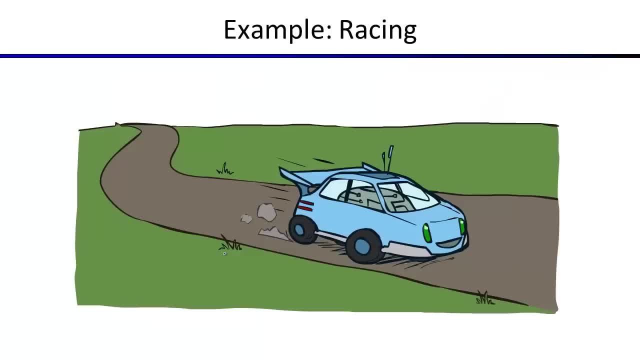 As you can see here that as we change the utilities, the same set of computations give rise to different behavior, which is pretty cool. Okay, Let's look at another MVP, which is very just like search. It's very easy, I think, that all searches about grids and mazes- 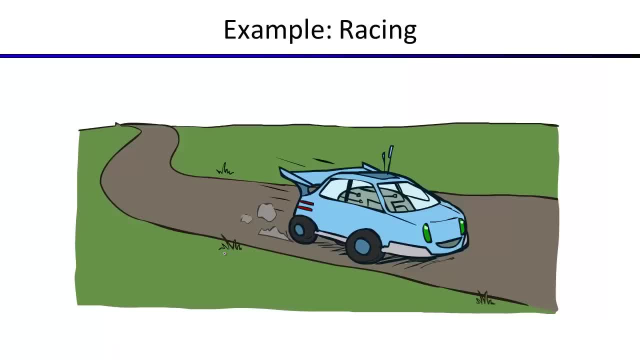 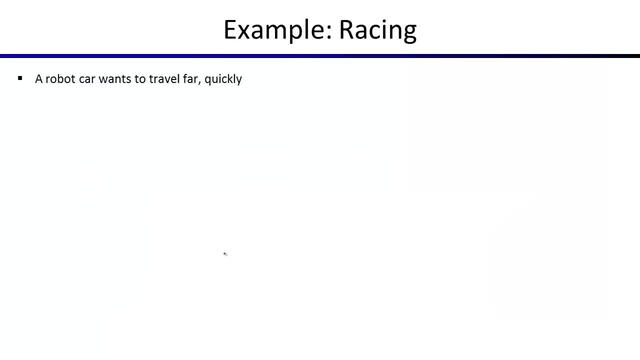 It's not, and not all MDPs are good worlds. So here's an example of a very simplified racing robot monitoring its own internal temperature. We have some robot car and what we want to do is have a far and quickly. far means you don't want to break down. 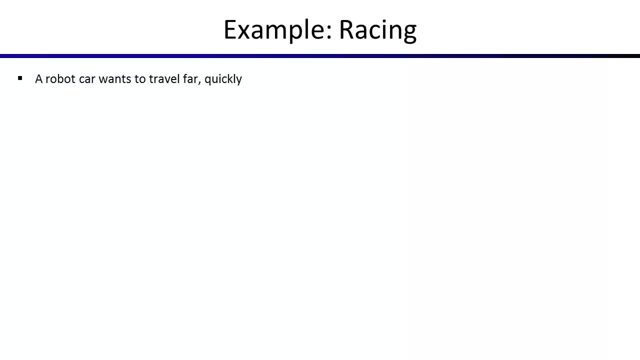 And quickly means you would like it to kind of move fast, All right. So how might might we formalize that? we could say: there's three states of the car. It can be cool. This is an engine here. Cool, It could be warm or it could be overheated, right. 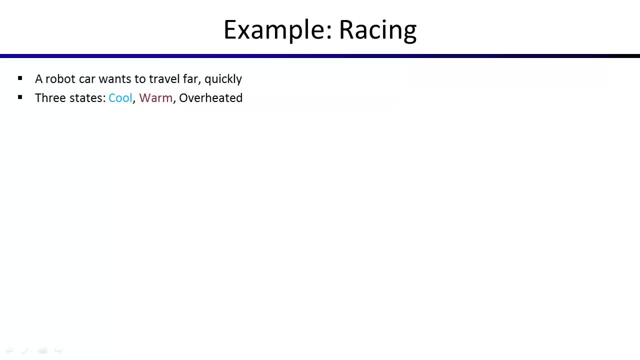 You ran, you know you ran it too hot and now the car is broken. So here's the three states. Cool, that's a happy car, Warm, kind of in a little bit of danger, and overheated means broken down And we'll imagine, from overheated There's no coming back from overheated. 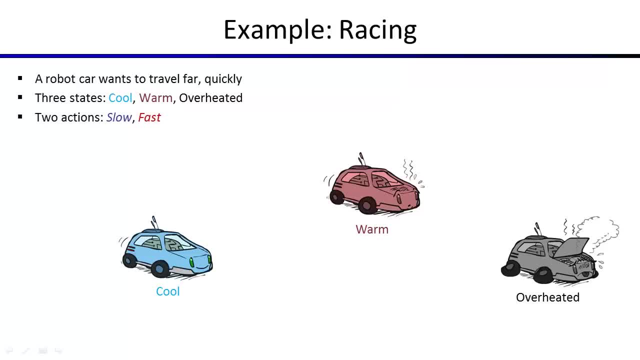 Okay, so there's two actions. You can drive slow or fast, and of course, we could formalize this with more states or with continuous Actions, but right now we're taking this formulation. All right, so they're slow and there's fast. Slow- what do these do? Well, slow, with probability one. 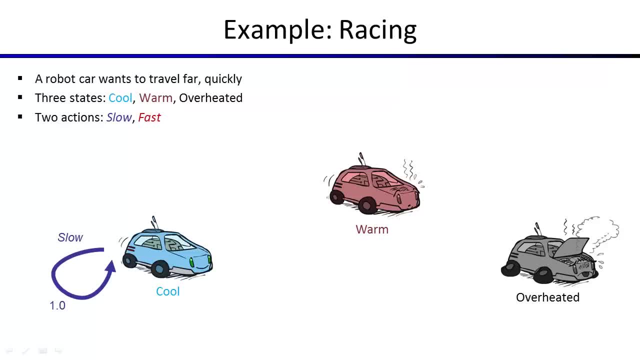 In fact it's deterministic. When you're cool and you take the slow action, you remain cool, if that makes sense. If you take the fast action when you're cool, half the time you remain cool and half the time you warm up. and now you're in the warm state. 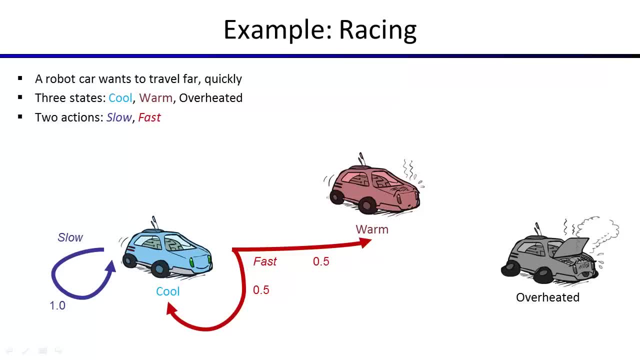 Okay, that's a non deterministic action. How about from warm? maybe slow has a percent chance of cooling you down and 50 percent chance of keeping you warm. Okay, how about what happens if you drive fast from the warm state? Well, you're guaranteed to overheat. 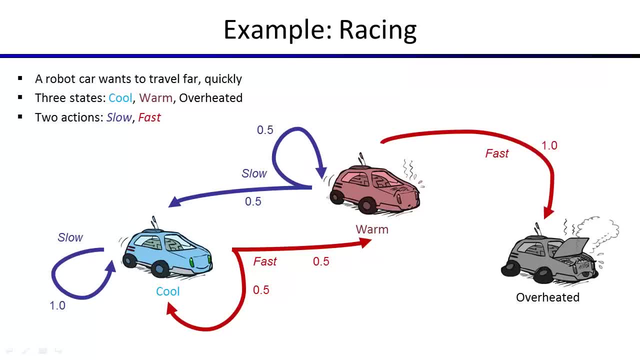 Okay, and so if we're overheated, that's kind of a terminal state. From that point forward, there are no rewards, And these are the probabilities. these are the actions that apply and what they do, and what we need to show now is not just the transition function. So these 0.5s- 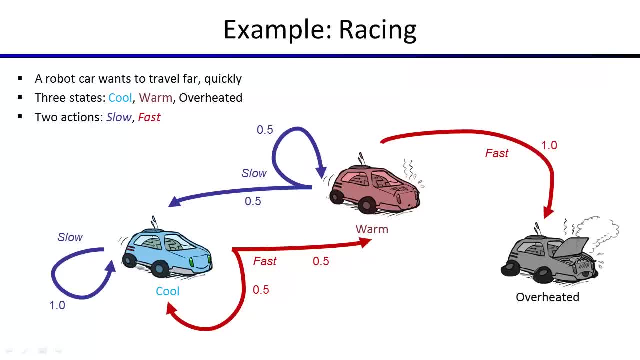 and 1s. these are the transition functions T. Okay, what are the rewards? Well, we have to, we have to kind of say precisely what they are. So maybe going faster gets you double the reward, which means on whenever you go slow you get a plus one, and whenever you go, 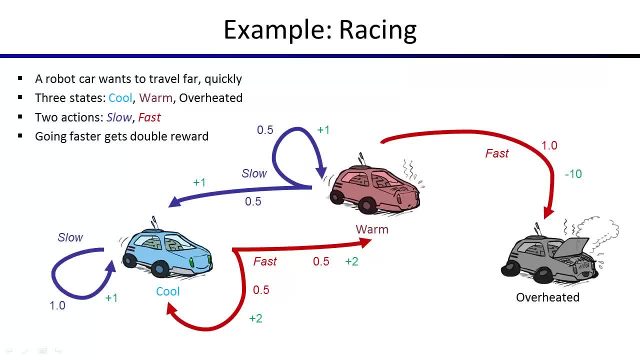 fast, you get a plus two, unless, of course, you overheat in the process, and then you'll get a minus 10 and the game will end Okay, so there's a very small MDP. This is a little bit different than the other MDP, right, There's no x, y coordinates or anything like that. 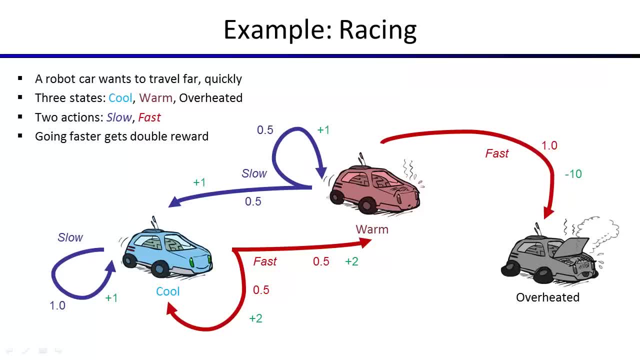 There's not that many states, But you can imagine this MDP going on forever, right, As long as you don't drive too fast, you can keep driving forever. So now we're going to have to start thinking about what happens if the MDP actually lasts forever. 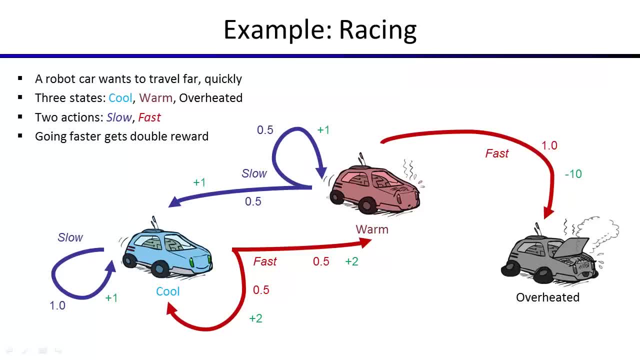 Okay, so any questions on this example? We're going to see it a lot. Okay, so let's think about a search tree. So if I said, all right, here's this MDP, the car is currently cool, what should you do? 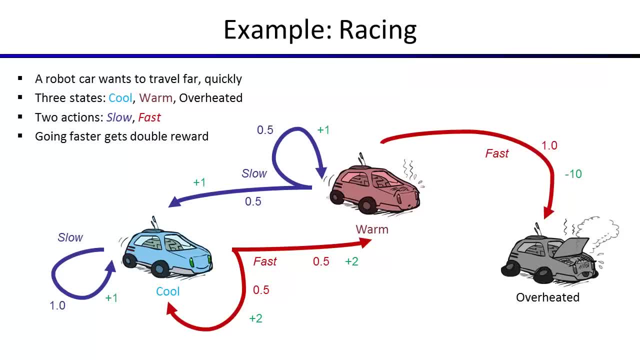 We're looking at it. what should you do? You should go fast, because you'll always be able to kind of slow down if you, if you have a need to heat up. Okay, so you should go fast. How might you determine that? 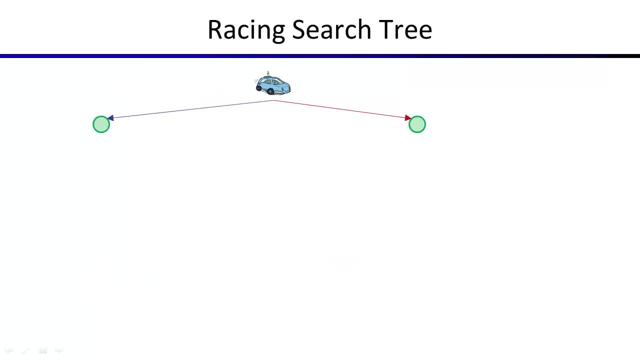 You might say: well, that's currently cool and my choices are: I can go fast or I can go slow. Here, left is blue, which is going slow. Now what happens if I go slow? Guaranteed to remain cool, All right. if I go fast, I have a 50-50 chance of either remaining cool or getting hot. 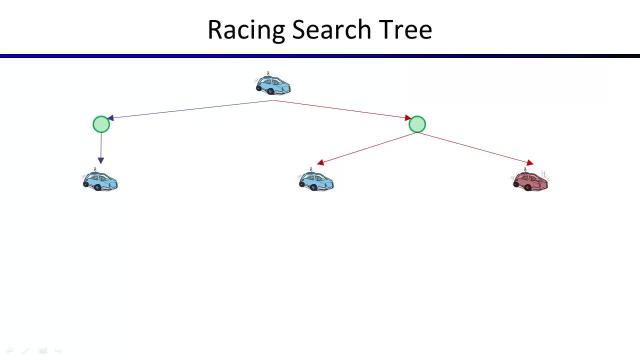 This should start to look familiar, right? Because if I think forward to the future, I'll have choices again from these points, And so again I'll have a choice between each of those possible outcomes- slow, and then some chance node will take over and determine what happens. 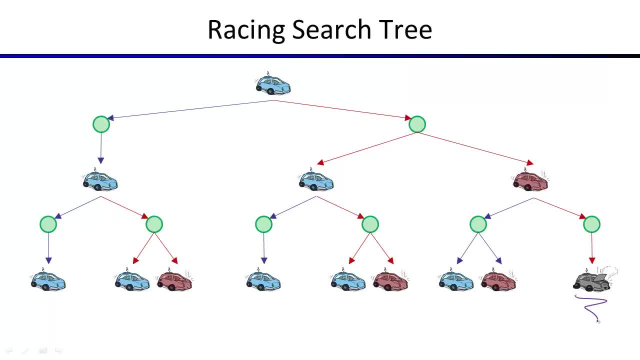 And you can see, if I go fast and I go fast and I'm unlucky, then I might overheat. Okay, so presumably, if I crunch the numbers and in this I should go fast and then at that point probably slow down, Okay, so that's a search tree. What does this look like? 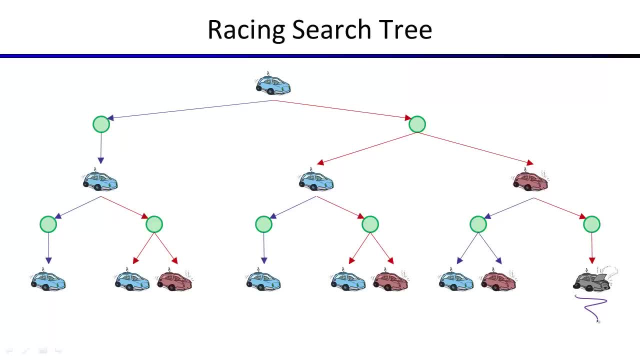 This is an expect to max tree. There's max nodes, except they're shaped like cars and there's chance nodes and they even look like circles. Okay, there's only one difference between an expect to max, as we learned in the last lecture, and this tree right, And that is: where are the 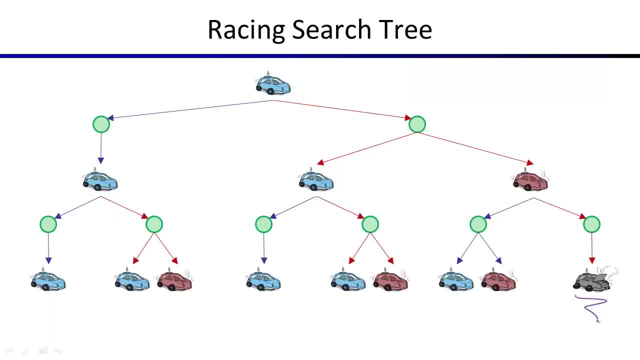 rewards in an expect to max tree for a game. They're all at the end. When the game ends you have some score, or you win or you lose, and everything in between is kind of propagated up from the bottom. Here there are actually, you know, rewards as you go. So when I choose to go, 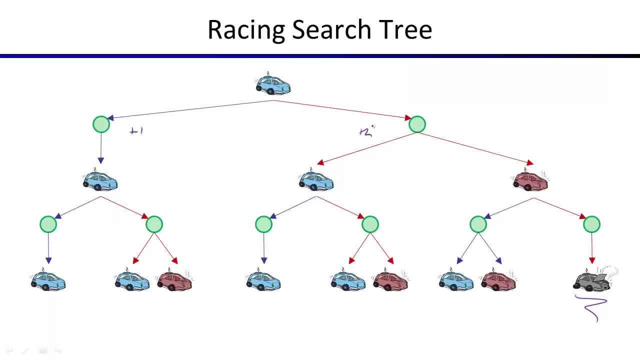 slow, I get a plus one. If I choose to go fast, I get a plus two, And the rewards are kind of spread throughout the tree. So there'll have to be some minor bookkeeping to deal with the fact that the rewards come in step by step. Beyond that, it's expect to max. 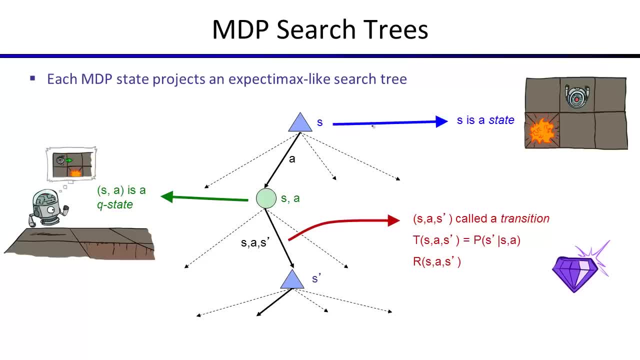 You can think in your head that from any state the futures you might experience in an MDP. they look like expect to max And every algorithm- even though in general we're not going to be using expect to max to solve these- every algorithm at its core is expect to max or kind of is derived. 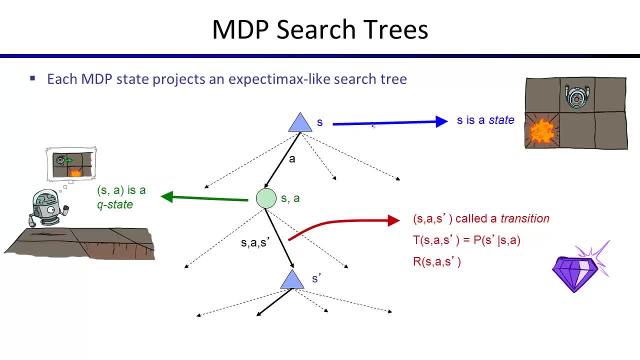 from the same kinds of thinking. that gives rise to expect to max. So I hope you like expect to max, A lot of expect to max. Each MDP state is going to project a kind of a search tree. We know what states are, So a state here is the current situation of the world and that's. 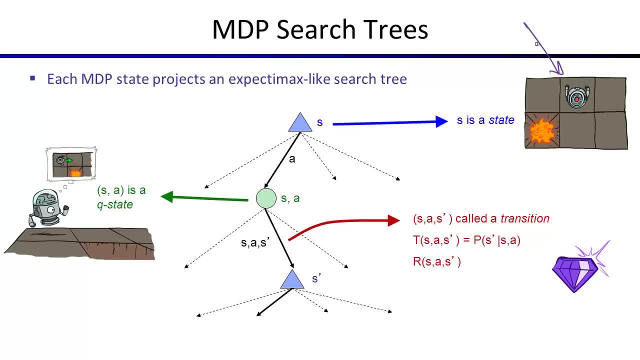 something like: I'm in this square. So states, we know them and we love them. What happens in a state? when you take an action? You control the action. So if you take the action, in some sense you've like you've pushed the button on going north. You don't know whether you're. 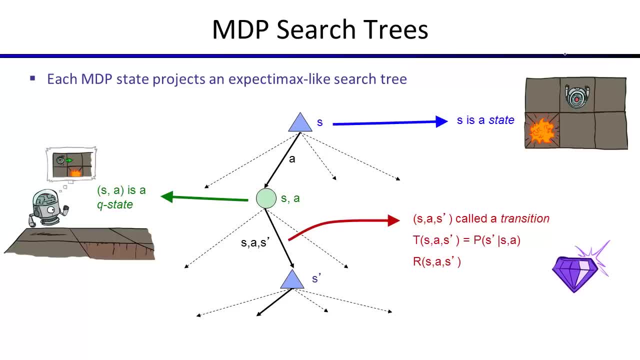 going to fall into the pit or not, Or you're going to state flood, or you're going to slip or whatever. But you were in a state and you've committed to an action. You're waiting to see how it results And, in essence, you've made your move and the world's going to make its move next and tell: 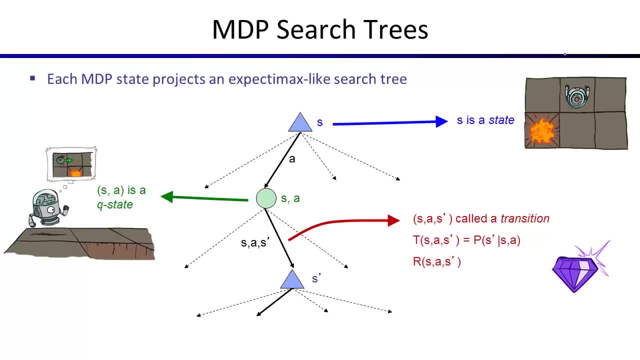 you what happens? That state of having been in a state S and committing to an action A, but being uncertain what's going to happen. this is called a Q state. This is probably like. this is probably the single most important and confusing piece of notation we're going to see today- And a Q state. 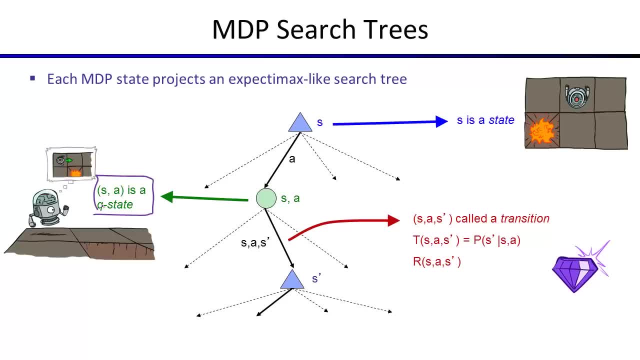 of a state in an action, And you can see in the illustration. here you're in a state. you've committed to moving, in this case to the east, but you don't know what's going to happen. Okay, so you move from a state to a Q state, S A, using a max node right. You pick an action. 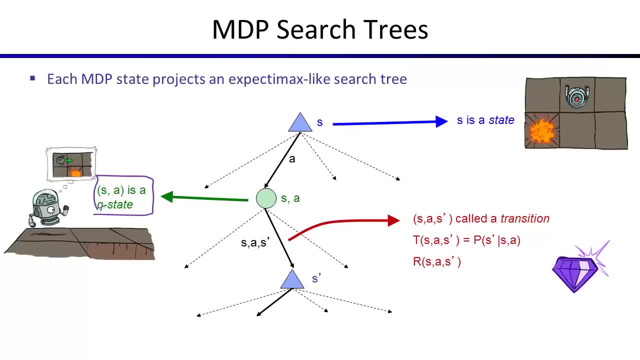 Then you move from a Q state S A to a result state S prime. That's the world, It's telling you what's going to happen. So we've got some terminology down here. So you pick an S, The environment picks an S prime, This pair- sorry, this S A, along with the result S prime. So this: 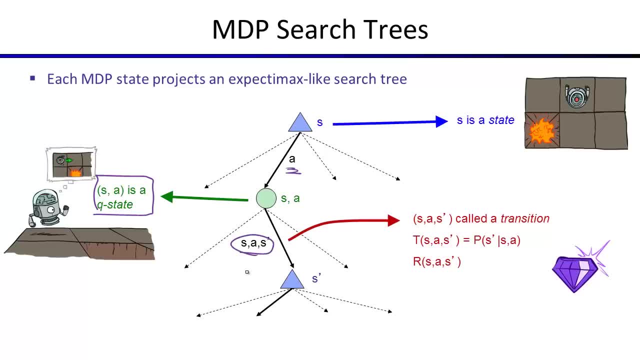 this triple here S A, S prime. This thing is called a transition, right, It's a state, It's an action that you chose and it's a response from the world. That's called a transition. The probability of the transition comes from T and the reward associated with the transition, which could be zero. 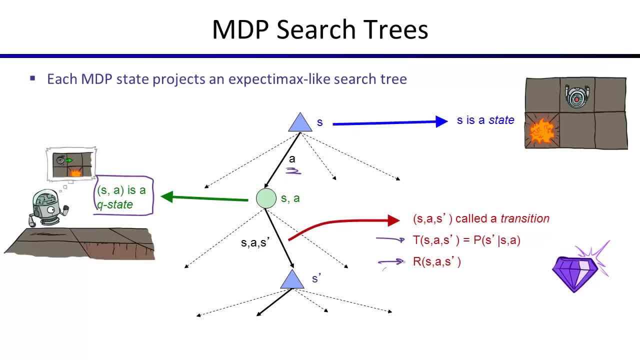 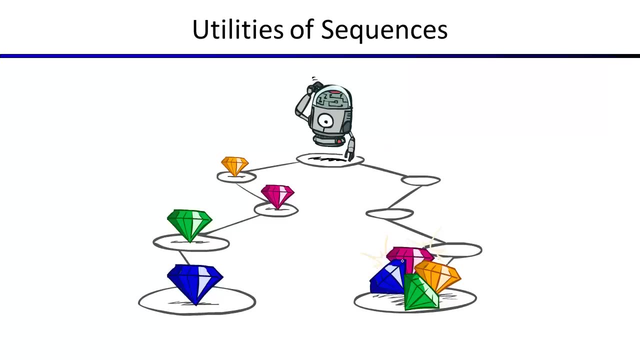 comes from the function R. Any questions on that? All the algorithms are going to manipulate these to kind of compute various sums and maxes. Okay, before we start solving these, let's actually think a little bit about something that I've been sweeping under the rug so far, And that is 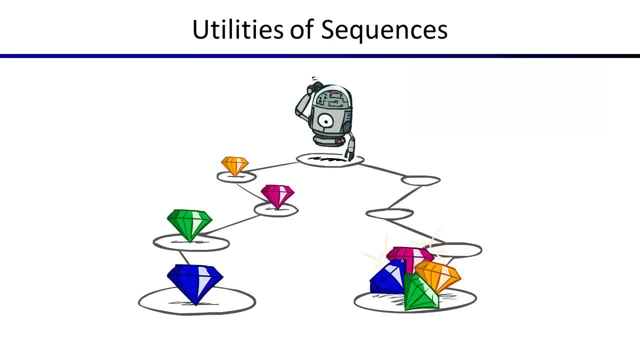 the MDP defines rewards, So this, this transition, gives you a plus one. this one gives you a minus one, Which means, when you have a sequence of actions and you experience a whole grid world or a racing robot, you get plus ones and minus ones and plus point threes and whatever it is. 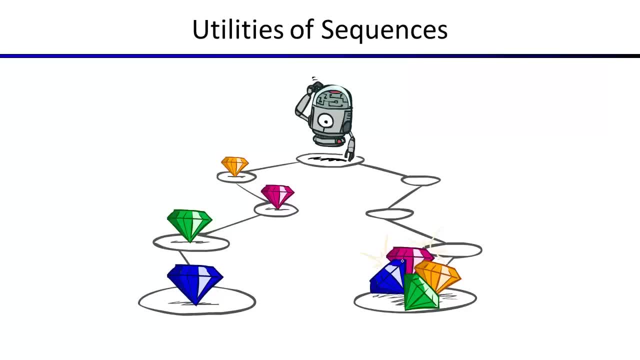 we've been adding them up. Who says that you should add up your rewards? Okay, so now we need to think a little bit about. we know we're going to get a sequence of utilities. what should our preferences be over, say, for example, getting you getting the rewards sooner rather than later? 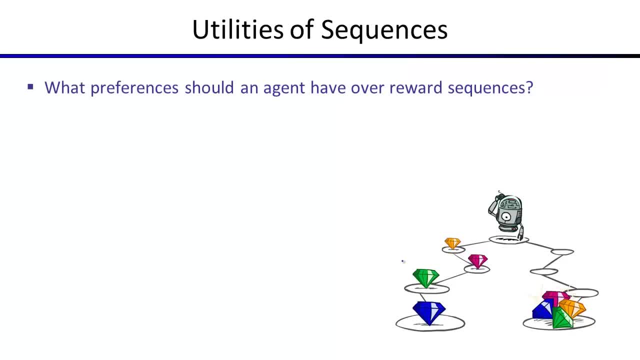 Okay. so what preferences should our agent have over sequences of rewards? Well, let's start with an easy question: Would you like more rewards or less rewards? It's reasonable the agent would like more rewards, Otherwise there's no reason for that. we got our signs wrong. So, for example, if my choice were between the reward sequence 1,, 2,, 2,. 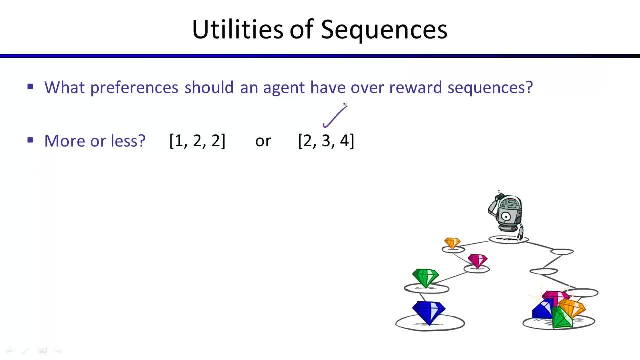 or 2,, 3,, 4, what should I prefer? Right, I should prefer the one that has bigger numbers. Okay, that's easy. Adding them up satisfies this right. If you add them up, then you prefer things that. 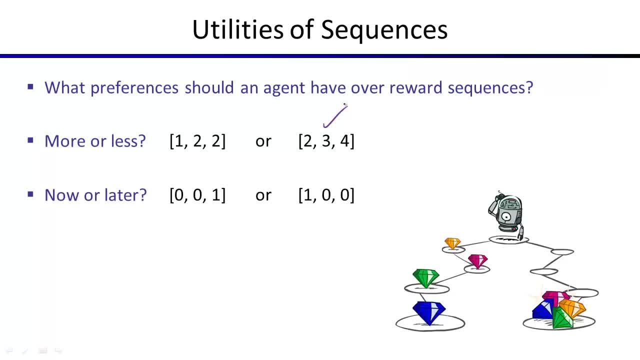 are more. However, how about now versus later? So what would you rather have if you were an agent? Would you rather have the reward sequence 0, 0, 1, or the reward sequence 1, 0, 0?? Or maybe you're. 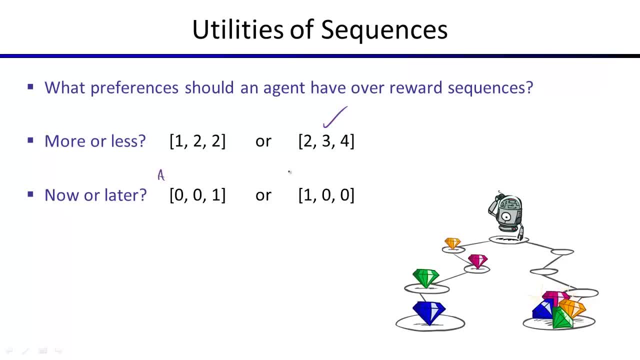 indifferent. A, B, Who prefers A? Who prefers B? Who's indifferent? Okay, By the way, totally reasonable to be indifferent, and it's also reasonable to prefer for B, right? Somebody says: what would you rather have? Would you rather have $1,000 right now or in six years? Well, 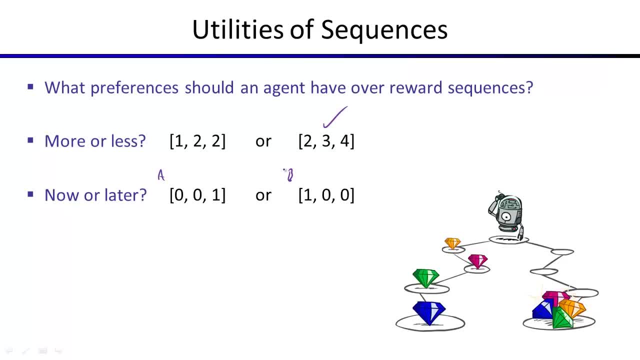 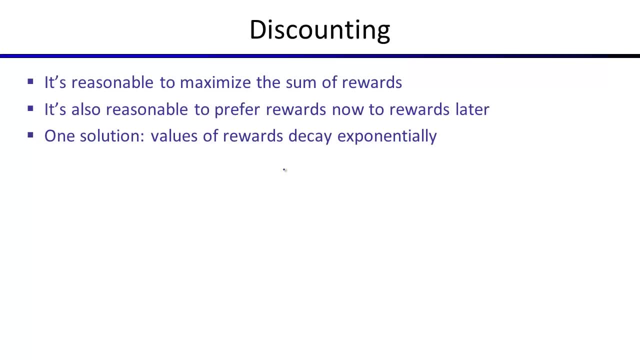 like it seems reasonable to prefer it now, right, So it's totally fine to maximize the sum of rewards. Sometimes that's an appropriate formulation of your utilities. It's also reasonable to prefer things now rather than later. But if you do that, there's now a trade-off. Maybe you'd rather have $900 now than $900 later. 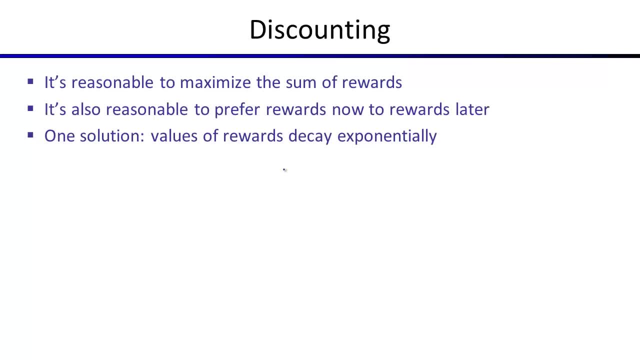 but would you rather have $900 now than $1,000 later? Who knows? This depends on the details of your preference function. So one solution that captures this idea that rewards are worth more now than later is when you consider their value in terms of utilities. you take the reward itself. 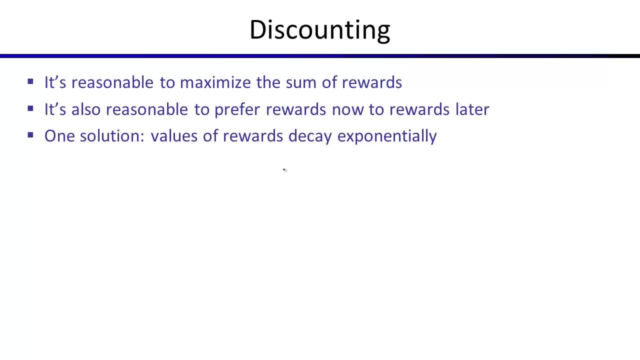 and somehow discount it for being in the future. And so you can do this by an exponential decay. This is the standard method. You say, if I get to that gem it's worth one, if it happens in this time step, But if it happens in the next time? 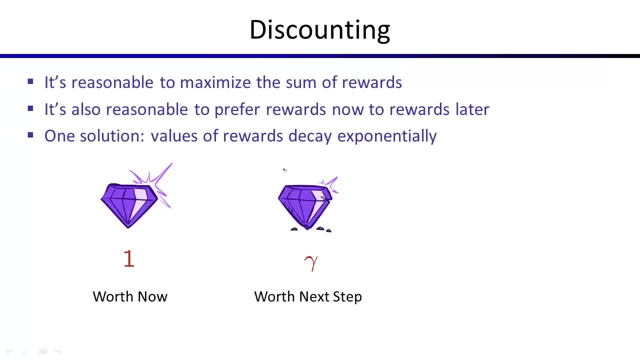 step, it's worth less. How much less? Let's say gamma. Gamma will be some number which is called a discount, and it'll be something between zero and one. What happens if I don't get this gem for two time steps? Well, I'll get my discount twice. so it'll be worth gamma squared. And if I get it, 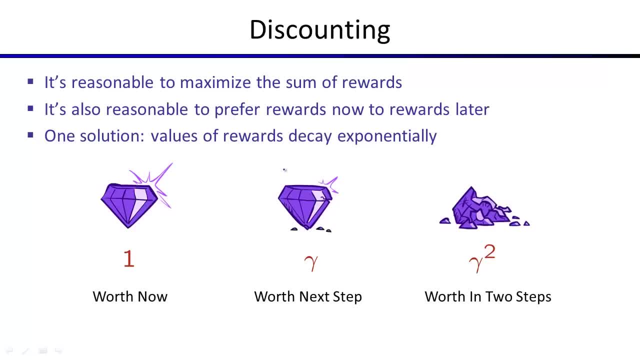 kind of infinitely far in the future, its value will kind of will tend towards zero, right, And that seems reasonable too. So this is called discounting, Okay. so first of all let's talk about how you might deal with discounting, and then we'll talk. 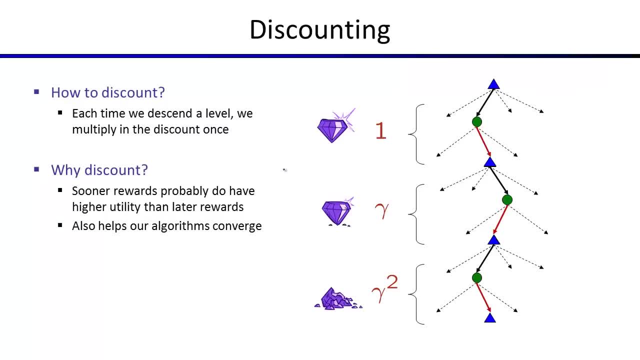 about why we do it and kind of think about it a little more formally, So mechanically. if you think about this tree of possible futures, remember you can get rewards at every level. Now in grid world, all the big ones are at the end for small values of the living reward. 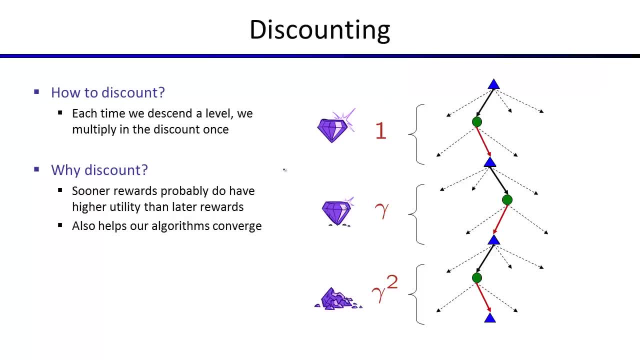 but in the car racing you kind of get plus ones and minus ones as you go right. So there's rewards at every level And we are going to add them up. But what we do is to the extent that you think about this as a kind of recursive search, every time we move down a level into 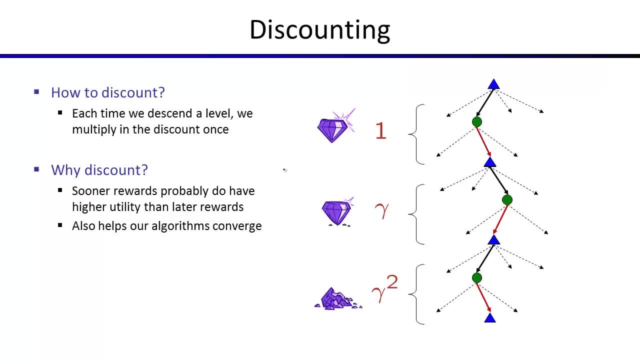 the tree, you get a factor of gamma which is less than one. that makes your rewards worth less and less, And once you pick up too many factors of gamma, the rewards- whether they were good or bad- they've been kind of pushed towards zero. So why should we do this? 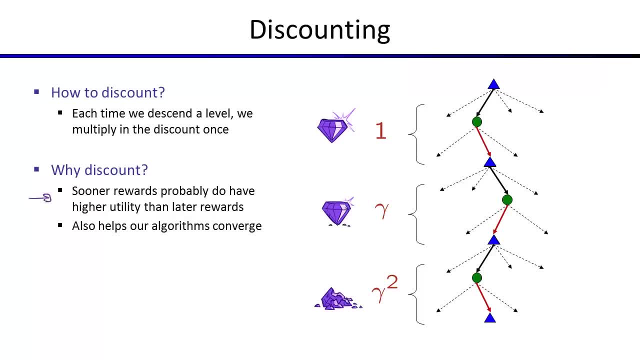 Well, one reason to do this is it probably is the case that rewards sooner should have higher utility. So you all said most of you would prefer to have the rewards sooner rather than later in the example, And this gives you that When gamma is like 0.9999, you kind. 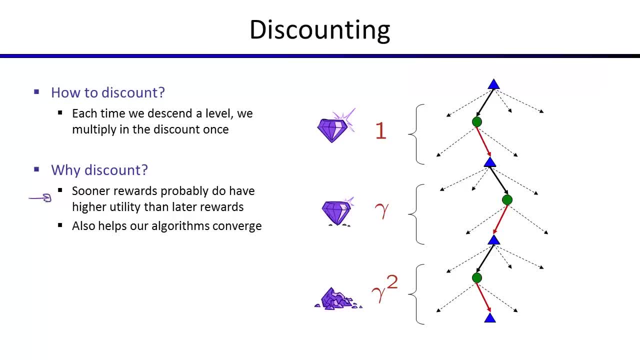 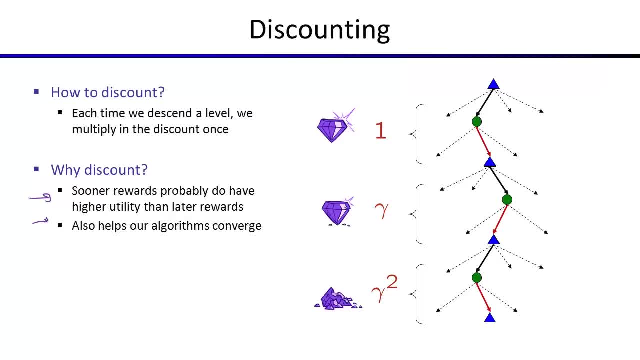 set gamma to 0.001, you get 0.001.. And if you set gamma to 0.001, you get 0.001. And it's just kind of converge better if the distant future doesn't matter, When the distant 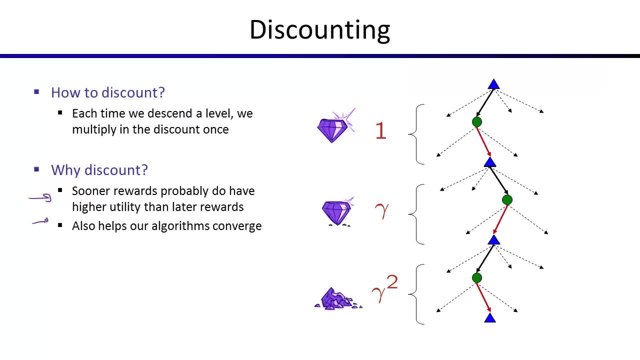 future matters. you're kind of forced to think about it And that has a computational cost. Okay, Well, let's do an example. Let's say your discount is 0.5.. Every time step in the future that your reward comes, it's worth half as much to you. So if I think about the 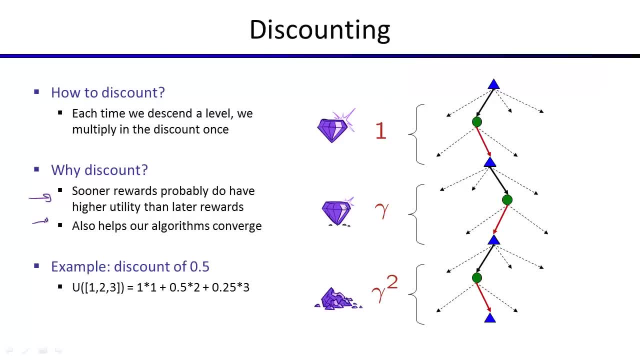 utility sequence 1 to 3, the sum of utilities is 6.. But the sum of discounted utilities is 1 for the first reward, because it gets full value. The second reward is a 2, which, but it's only worth half as much because it's coming one step in the future. 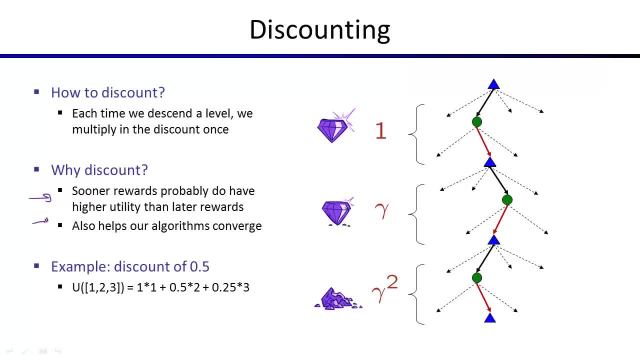 And the third reward is coming two steps in the future, so it's only worth a quarter as much. So you add all of those up and what you get is you get that now the utility of 1,, 2, 3 is less than the utility of 3, 2, 1.. 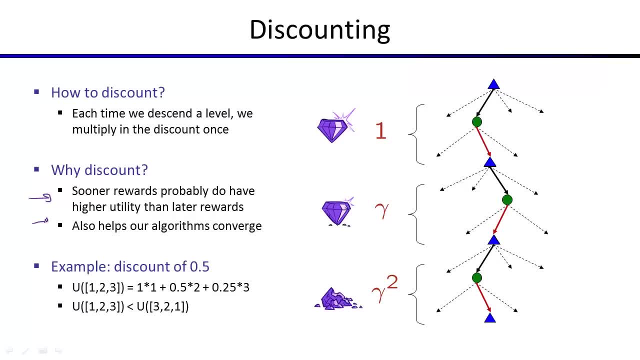 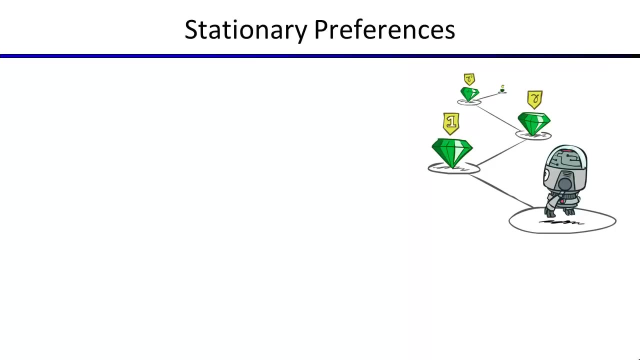 Their sum is the same, but their discounted sum is going to be different. So now we've got two techniques for turning sequences of rewards into utilities. You might then wonder. you know, adding them up, that was intuitive Discounting. that's a little weird. Why was it exponential? 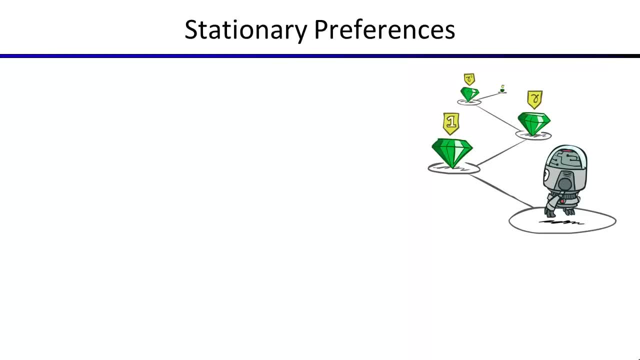 Maybe there's 17 other things that are all reasonable, And actually there are a lot of preference functions that would count as rational, but there's a kind of preference function that we call stationary. What is a stationary preference function? A stationary preference function says essentially: 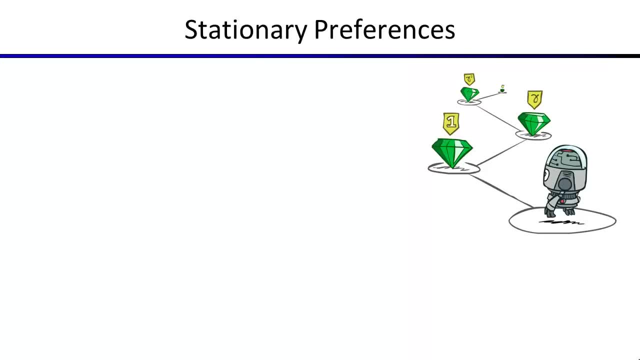 that whatever I prefer today, I prefer tomorrow. Okay, so what's a stationary preference function? So we assume stationary preferences, which formally mean if I prefer one sequence- A1, A2, A3, and so on- to another sequence B1, B2.. 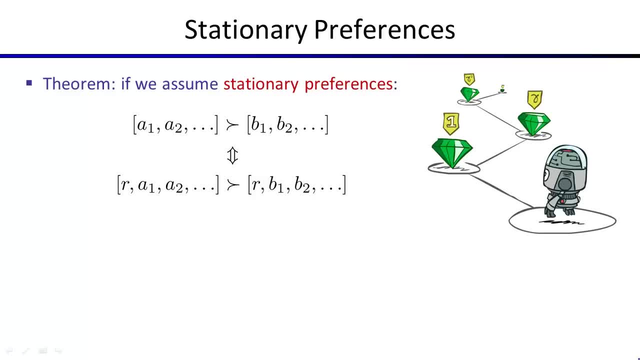 So I like the A sequence better than the B sequence. If I take those same sequences, I push them one step in the future and I give them R in the first step, so the same. These are two sequences that are the same in the first step. 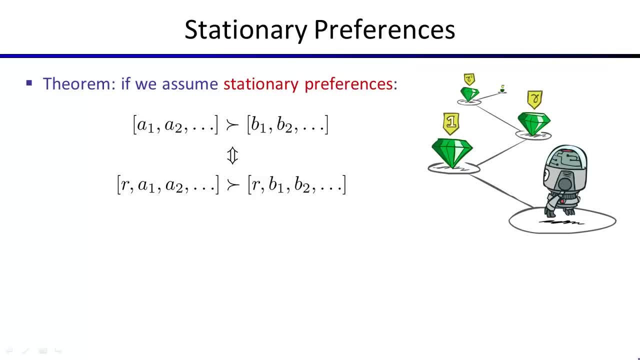 and then I like A better than B. I should preserve my preferences Right, shifting things into the future, but otherwise keeping them identical shouldn't be a problem. I should change my orderings If that's true. we say your preferences are stationary. 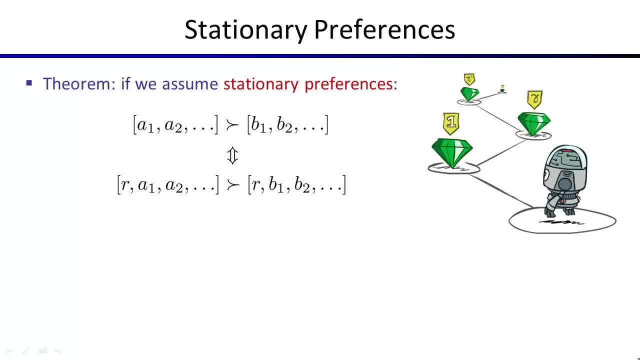 Is it possible to have non-static stationary preferences? Absolutely, But if you have stationary preferences, then you have a theorem that tells you there's only two ways to define utilities that work out. One is additive utilities and the other is adding discounted utilities. 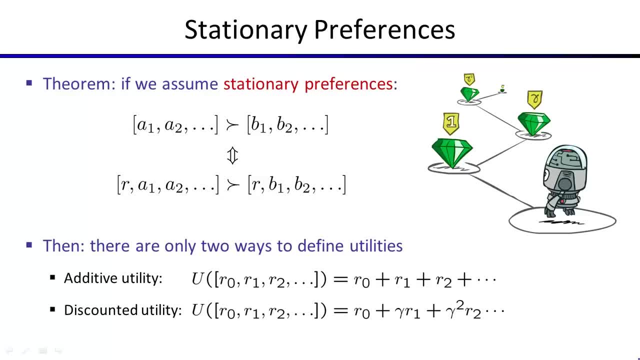 And in fact, if you like gamma B1, you get additive utilities. So there's really only one thing you can do. Because of this, all of the solutions that we do from this point forward is going to be in terms of discounted utilities. 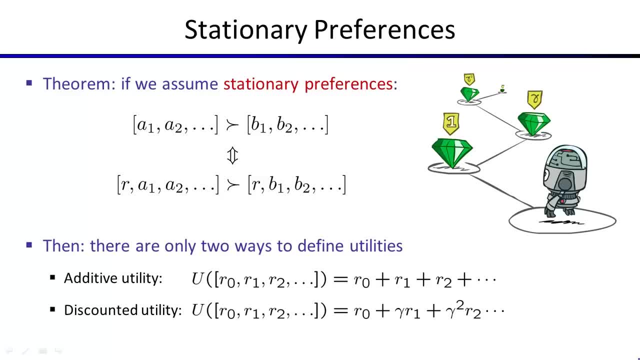 and you can always set gamma equal to one if you just want to add them up. That means that in all our equations going forward, there's going to be these gammas floating around, And that's what they mean. It means, every time I take a time, step into the future. 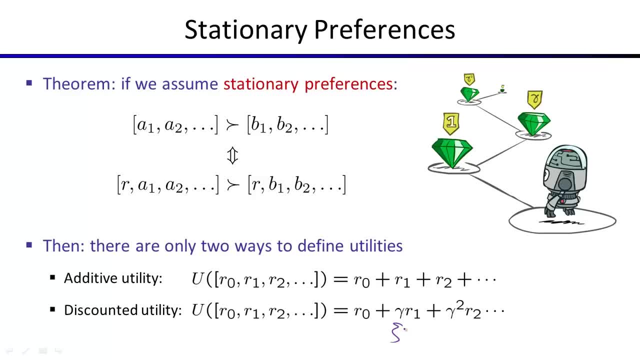 whatever happens, gets deflated by a factor of gamma. Any questions on this? Yes, Good question. If you assume your preferences are stationary, then you essentially can derive that your utility function- remember, utilities are numbers that express preferences- you can prove that you have to have one of these utility formulations. 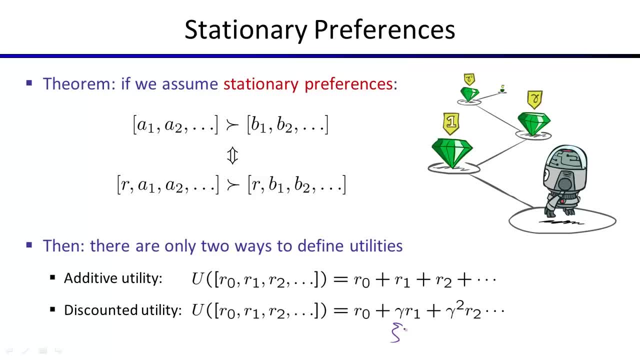 It doesn't mean your preferences have to be stationary. So there are cases, for example, say, if you're playing a game that ends at a certain time, like life, Life ends at a certain time. We don't always know when, but it doesn't go on forever. 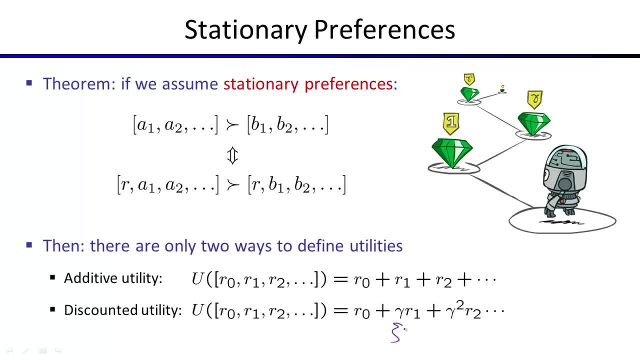 And so your utilities in life aren't stationary. The things you want today may not be the same preference functions you want, And that's because you can't just shift things in the future, because they kind of scroll out the end, And because of that there are very reasonable cases. 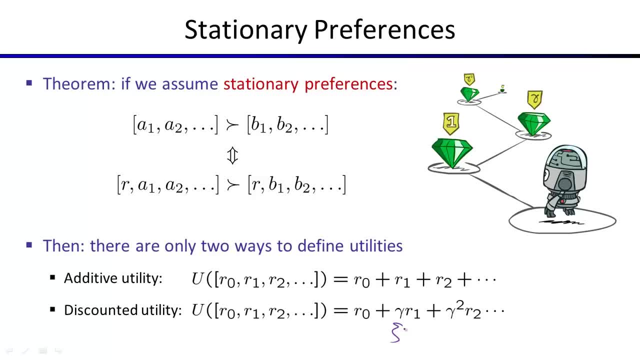 where stationary preferences is not a reasonable assumption, But when they're stationary you kind of can derive that they have to be some sort of discounted. Any other questions? Oh yeah, sorry, Can you talk a little bit about preferences, Sure. 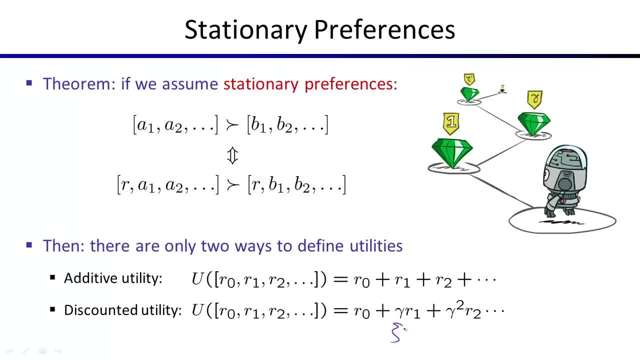 Preferences are called stationary preferences. and they're called stationary preferences because they have to be some sort of discounted. So if you're playing a game that ends at a certain time, preferences are called stationary if they obey the following thing. So I say: 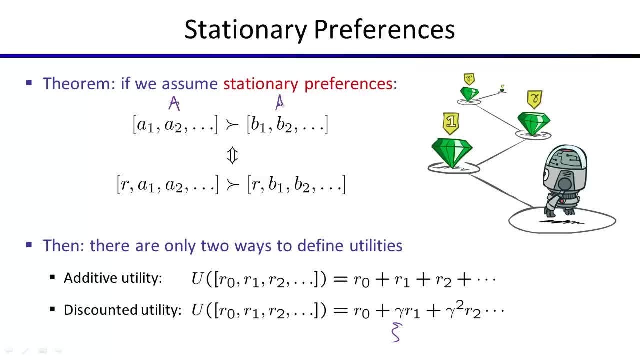 here's one sequence. we can call it capital A, and here's another sequence, capital B, If I prefer. Wow, that piece looks a lot like an A, doesn't it? Capital A and capital B, If I prefer capital A to capital B, which is fine. 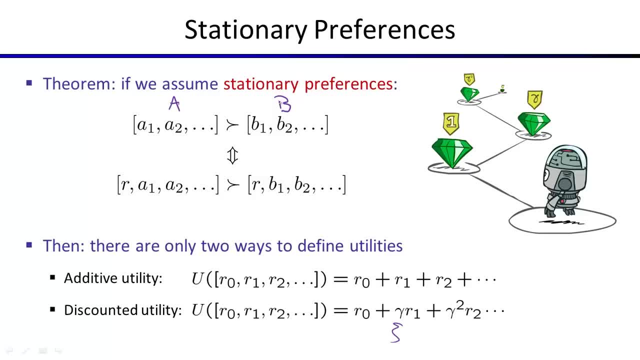 they're different sequences. what should happen if I take those sequences and I create new sequences which are essentially R, some fixed number, followed by A, And this one's R, followed by B? So it seems like if A is better than B. 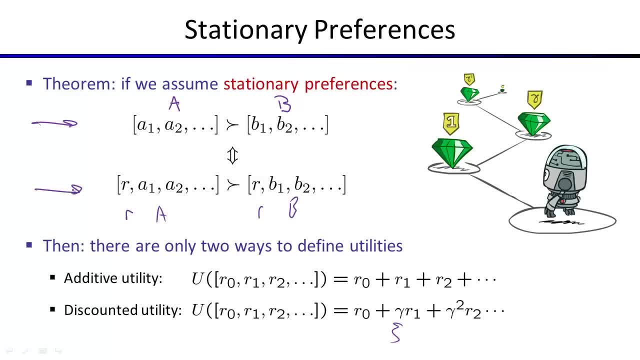 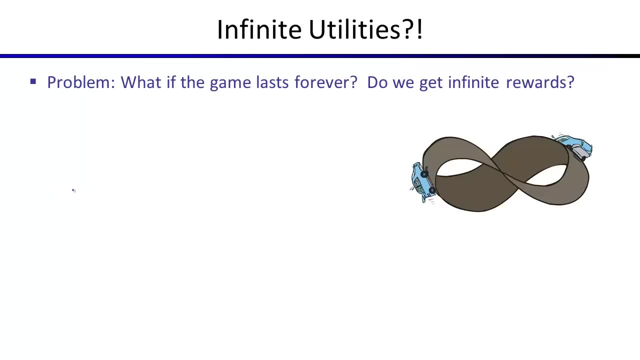 now, which is up here, A should be better than B one step in the future, assuming that first step is identical. If that holds, you say your preferences are stationary, But your preferences may not be stationary. Okay, So now we have a problem. we alluded to it. 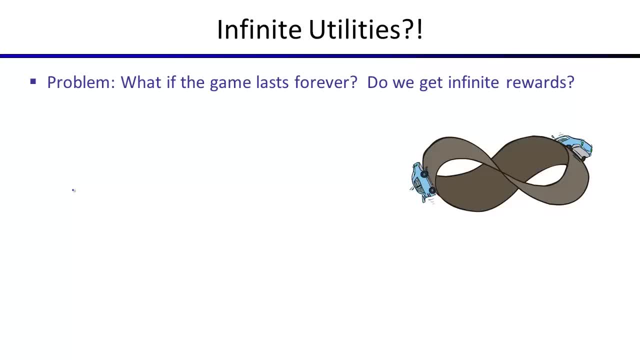 but we're going to talk about it now. which is what happens if your game lasts forever? Life may not last forever, because mathematical games can, And does that mean you get infinite rewards If that car drives forever? does that mean it's just kind of fast-slow? 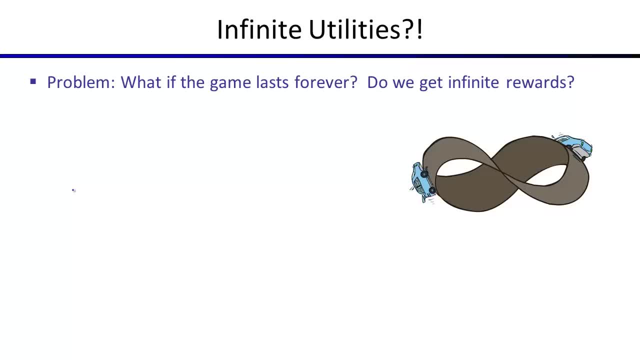 it doesn't matter, you're going to get infinity eventually. You can see how there might be a problem for infinite games if good and bad policies all give rise to infinity eventually. And now who cares what you do in the short term? So we need something to deal with these things. 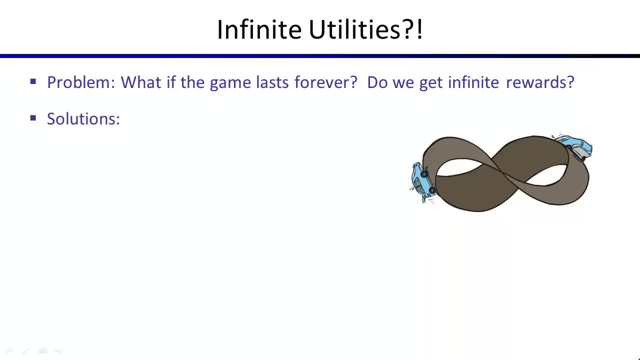 that last forever. And there's really two solutions, two major solutions, but there's a couple ways these can fall out. One is finite horizon. This is a case where the game is in fact finite. So if the game ends after a limited number of time, steps 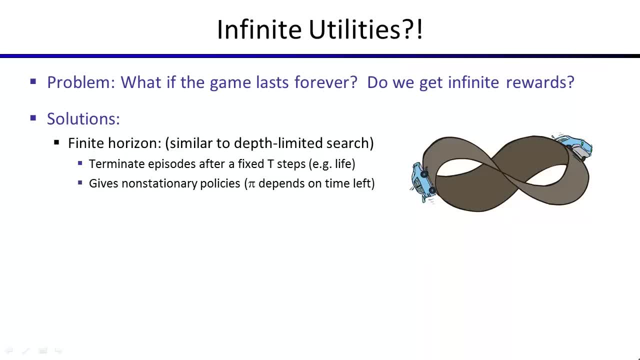 it's kind of like depth-limited search. The game goes and goes and goes. after 20 time steps, it's just done. This is like grid world with a countdown to the end of the world. In that case it's finite. 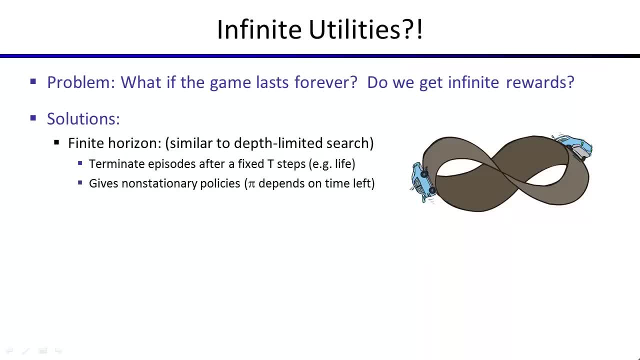 And in fact, you won't get stationary policies. The action you take is going to depend on the amount of time that's left, And that means the things are going to end after some fixed time, and life is like this. There's another solution. 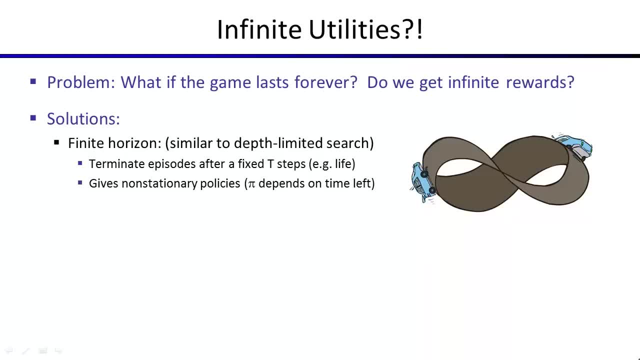 which is, your game could be finite. then you don't have to worry about infinity. or your game could be infinite, And when it's infinite, there's really two ways that things can work out okay. One is discount. Luckily, we already have the major solution. 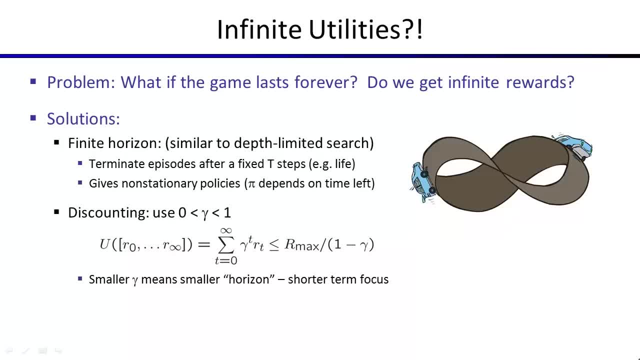 If you set your discount between 0 and 1, then even if your utility sequence of r's- the rewards of the time- steps, even if you get an infinite number of rewards, their sum is going to be bounded, assuming that the rewards themselves are bounded. 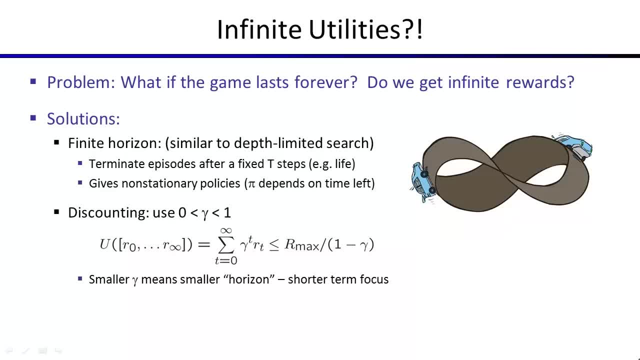 And essentially now, this is just about the math of infinite series. If you have this exponential decay, then when you add everything up, you're fine, at least if the rewards themselves are bounded above and below. What does gamma mean here? If gamma is 0,? 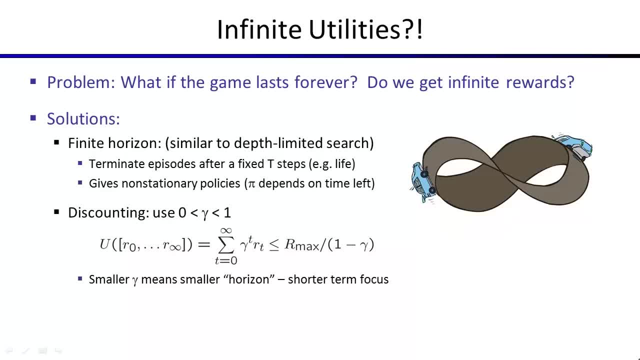 only the next time step matters, because after that everything is worthless. If gamma is 1, then you have infinite horizon, And so gamma in between is going to determine how far into the future the rewards matter, and in a kind of a soft way. 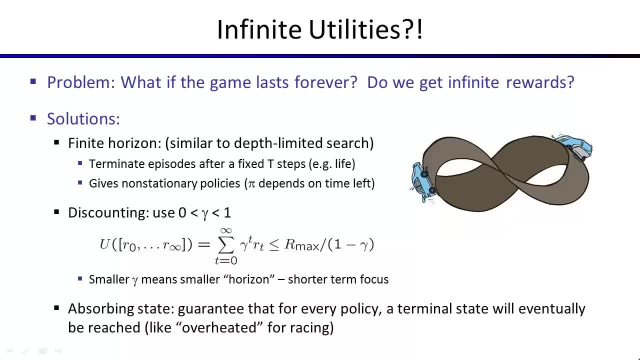 There's actually another way to do it, which is to have a guarantee that, no matter what your policy is, a terminal state will eventually be reached with probability 1.. So, for example, in the racing case, if there was always some chance to overheat. 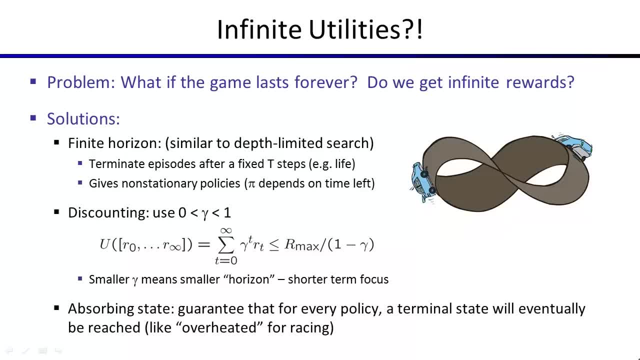 even though in principle you could have an infinite run of not overheating, with probability 1, you will eventually overheat And that means that when you average things together it'll kind of work out. It's something actually like having your game be finite. 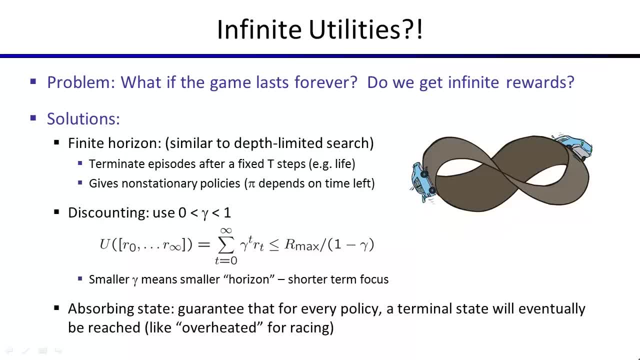 in a soft way And then, a year later, the odds are going to go against you and the game is going to end. Even if there are infinite sequences, they have infinitely small weights, Not because of the discounting, but because their probability goes to 0.. 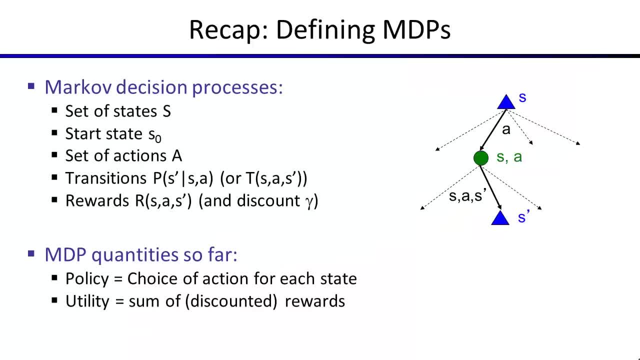 So that's what we do about infinite utilities. Any questions about that? Okay, so let's see where we are Actually. let's take a break right now and then we'll talk about algorithms for solving MVPs that have properties that are very complex. 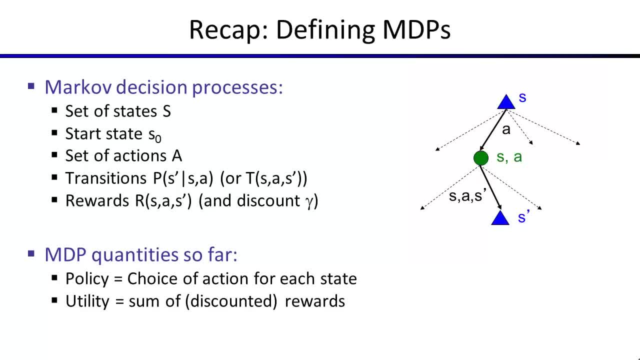 We'll take a couple minute break now. Okay, let's get started again. Okay, so all of that. everything we just did was about defining markup, decision processes and seeing examples of them and starting to talk about some of the notation for transition, probabilities, rewards. 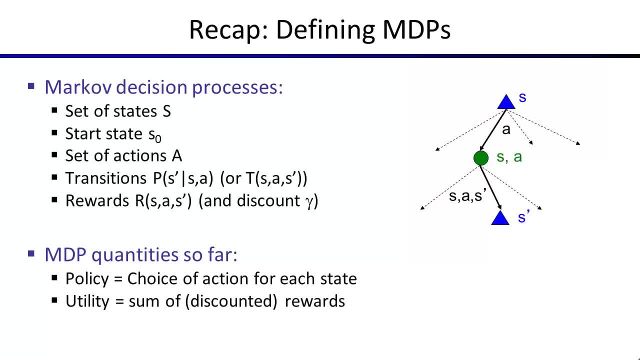 and things like that. Now that we have some intuition about what an MDP is, let's talk about algorithms for solving them. Okay, so let's recap What's an MDP? It's like a search problem, so it's got a set of states. 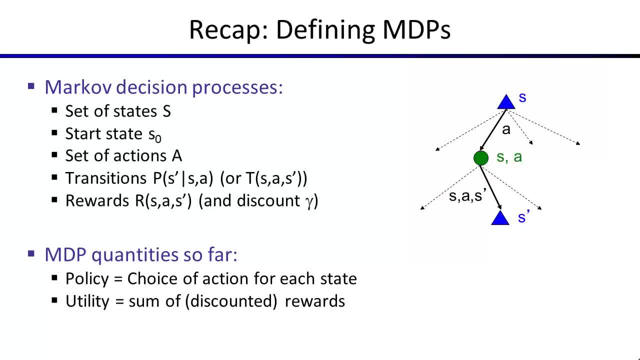 including a start state. It's got a set of actions and then it's got a successor function, and the successor function is composed of a transition function which tells you from each state how likely each outcome is, and a reward function which tells you for each state action. 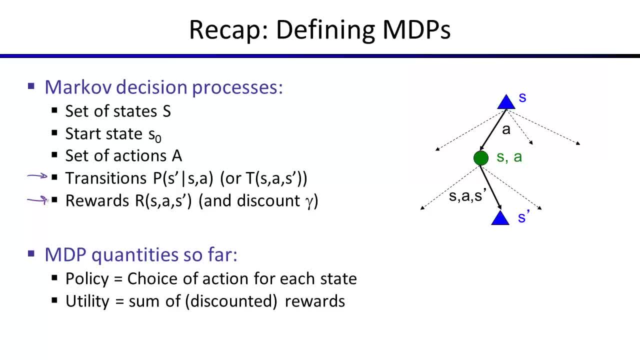 what the cost or what the reward is. In addition, an MDP has a discount which tells you something about how long your horizon is as far as the rewards go. So what are the quantities we've talked about? We've talked about a policy. 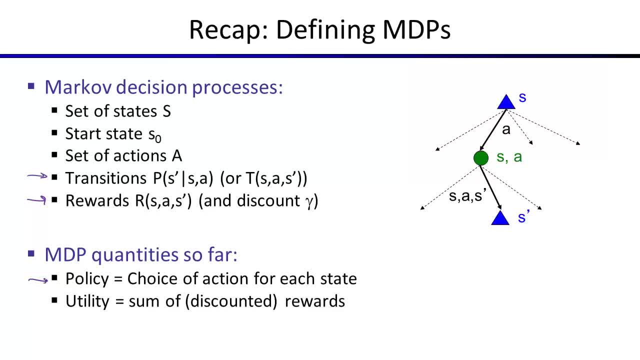 which, mathematically, is a map from states to actions, and we've been talking about utilities and we haven't been totally precise about what computations we're going to do with these utilities, but we know that, for a single sequence of rewards, the utility we're associating 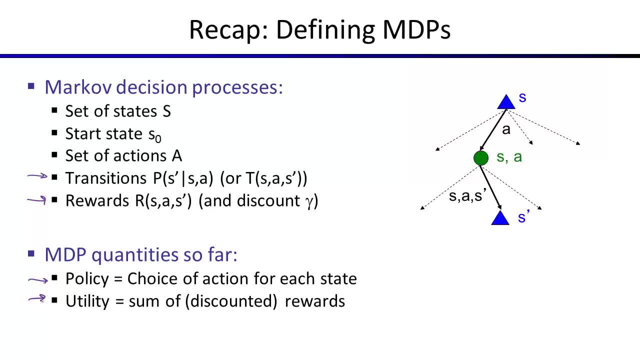 with. it is going to be the sum of discounted rewards, and that comes from a stationarity assumption. Okay, so we know the utility for a sequence of actions and we know what a policy is, but there's a lot of other things we need to compute. 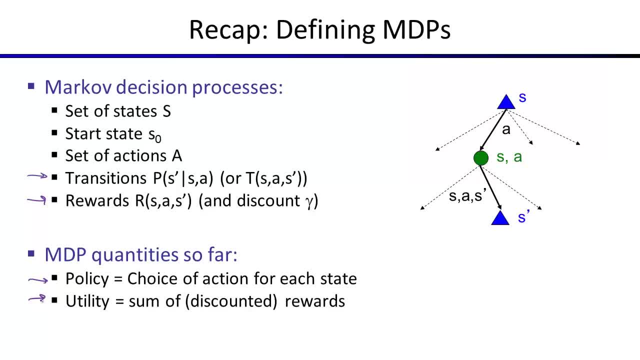 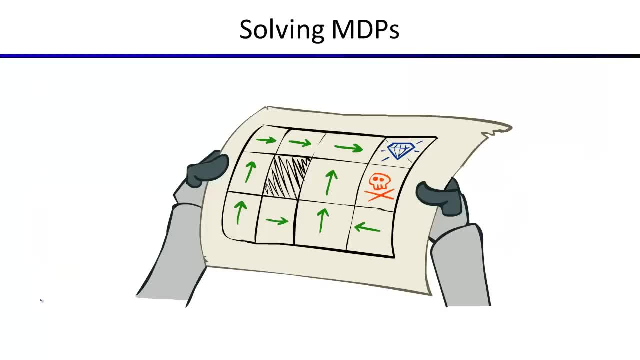 and computing things like what is the best policy or how good is this state. that's going to be the subject for the algorithms we're going to be looking at for the next lecture and a half. So first let's talk about what it means to solve. 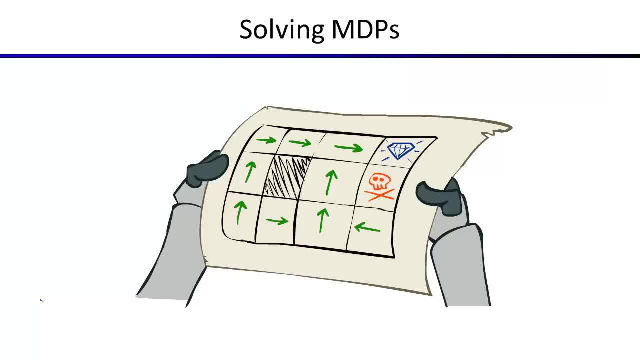 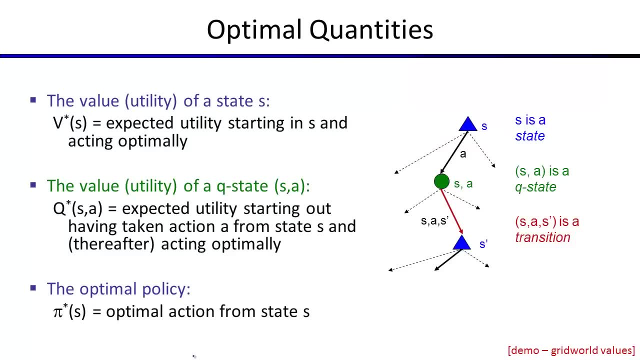 and then some new algorithms that effectively are going to take the ideas of expectamax and how to solve them. So let's talk about some quantities beyond policies and returns. One important kind of the central thing that you compute with MDP algorithms is what's called the value of a state. 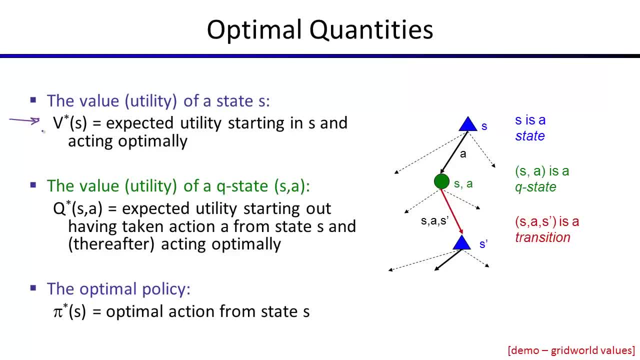 or the value of a multiple state. So the value of a state, V stands for value. here the star indicates optimality, And so the value function is: it takes a state and it returns a utility. But what utility? It's an expected utility. if you start in S, 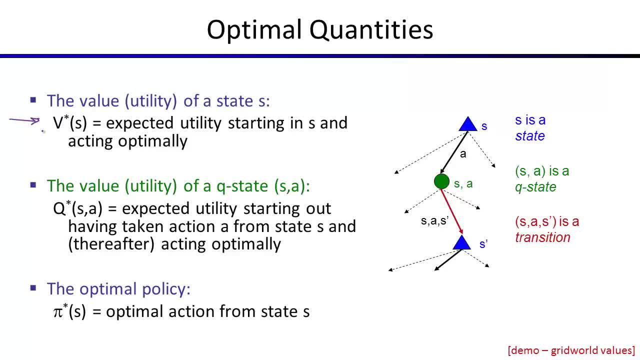 and act optimally. The reason why there has to be that optimally in there is because from a state you could do dumb things. If you're next to the pit of death, you could jump into the pit of death. That's a bad policy, and so the values. 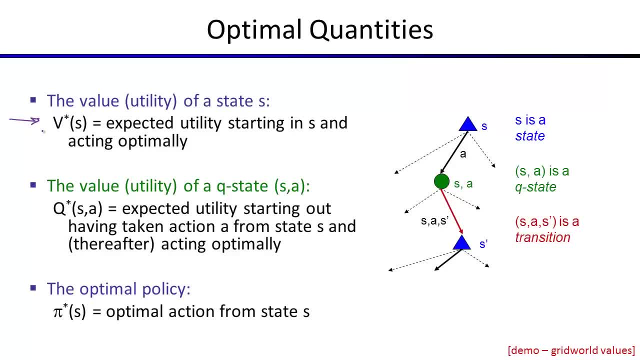 would be very low. A good policy might have very high values, And so when we talk about the value of a state, we either need to say what policy we're talking about- and we'll come to that later- or we need to say: this is the value under optimal play. 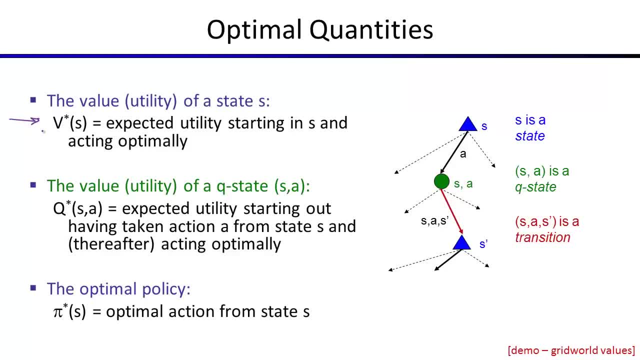 which then implicitly we're talking about an optimal policy. So the value of S is the expected utility, starting in S and acting optimally. Similarly, when we talk about a Q state, which is a state-action pair, we say the value is the expected utility. 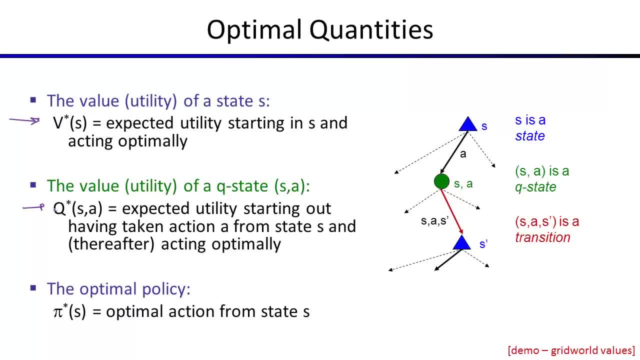 starting in that Q state, which means you were in action S, you committed to action A, which might have been a bad idea, but that's irrelevant, and from that point forward you act optimally. So we have values of states and values of Q states. 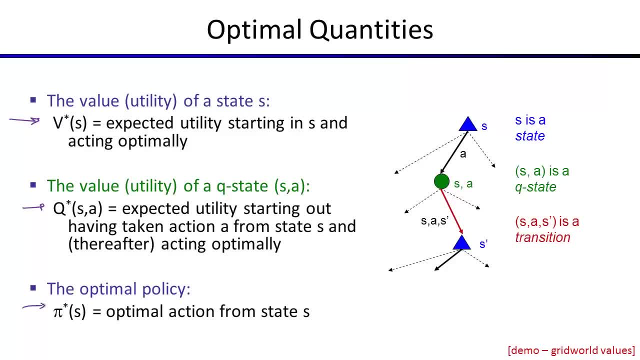 and we also have this notion of an optimal policy. So if we look at this on as expectum acts, we would say, if I'm in a state here and I think about the whole expectum acts tree and it would be inefficient to compute. 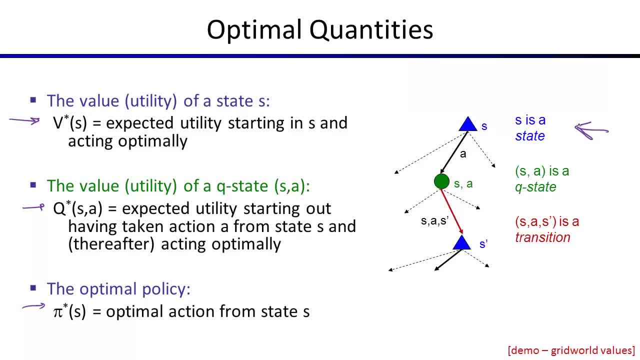 but let's just conceptually imagine if I computed the expectum acts value of this state, then what I would get is I would get V. So if we start an expectum acts computation from a state, the answer is the value of that state. 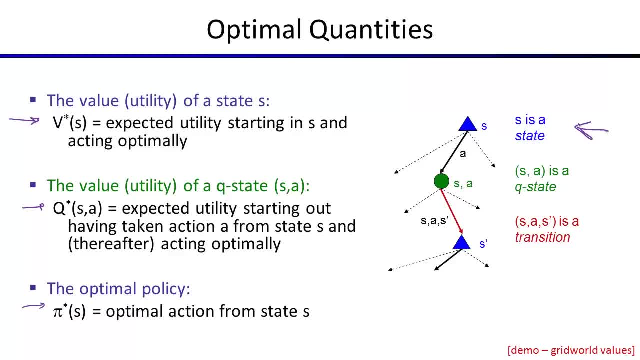 which takes into account averages by averaging over the chance node. that's the expectation part and it also takes into account optimality, which is the best action at every max node. So if we start, If we start an expectum acts at a chance node. 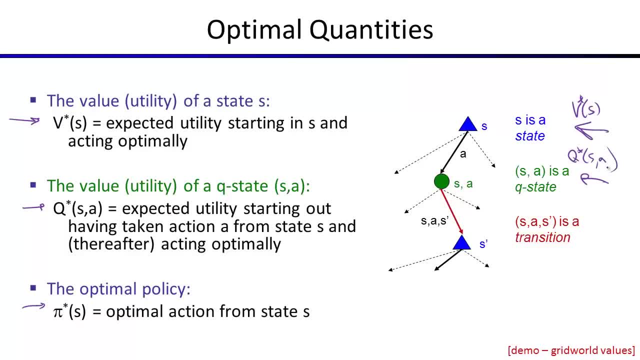 we'll get another value. So, even though it's kind of hard to get intuition about what a Q state is and you might forget it, the key thing is, when you do expectum acts for a state and for chance nodes, the value of a chance node with expectum acts. 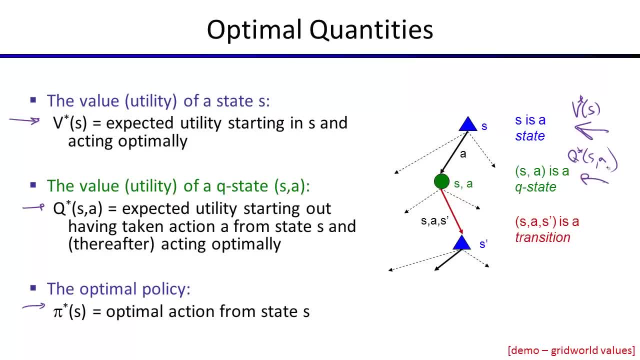 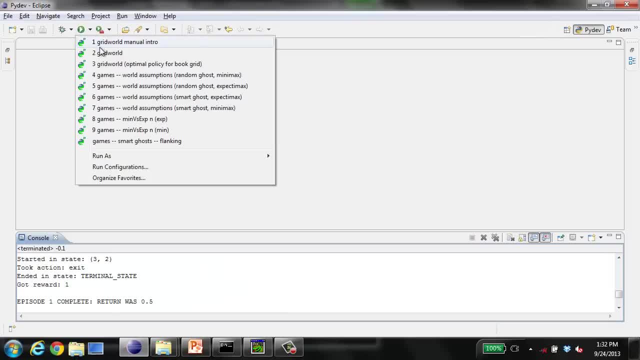 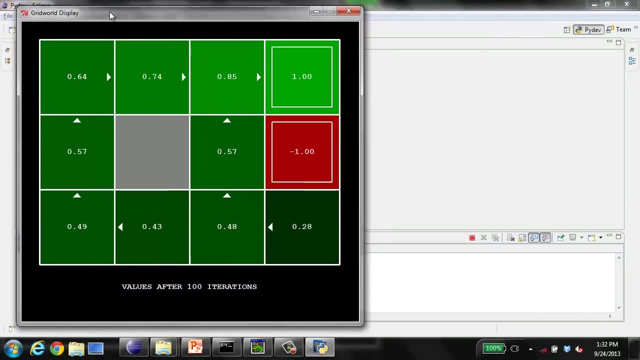 is the Q value. Okay, so let's see some examples of these. Okay, so this, by the way, these grids with numbers in them. this is the first half of your project: trees. Okay, so this grid world. what am I looking at? 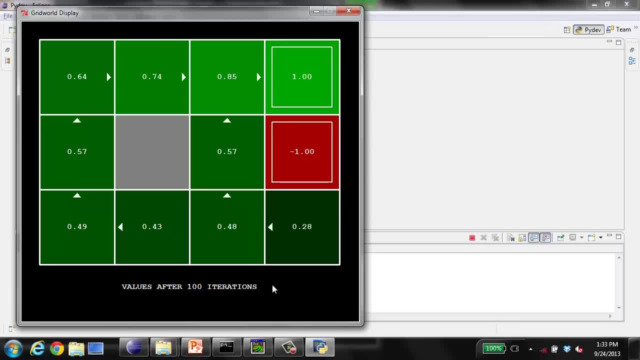 This is a grid world that has the standard grid world movement. you know rules: 10% noise in each direction, that kind of thing. It's also got some discount and it's also got some living reward for each time step. 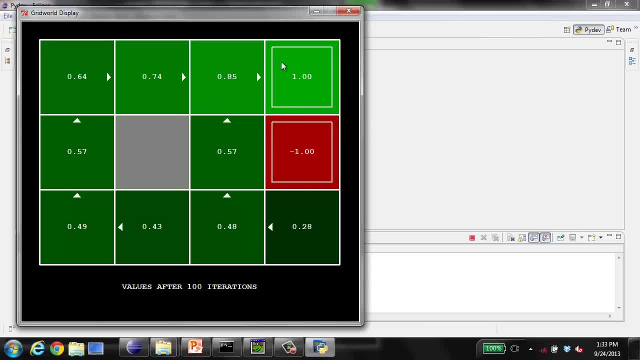 So what are these numbers we see? Well, some of the numbers are pretty interpretable. So, for example, in this square here we see a 1. What does that mean? In that square, if you act optimally, which involves choosing the action, exit? 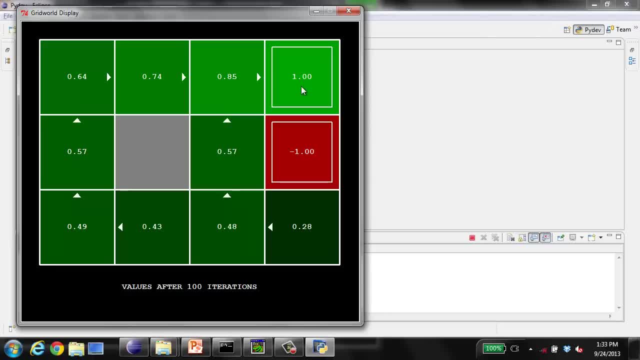 there's nothing else you can do. you're going to get a 1 every time, And that is the expected utility from starting in that state. How about, right here, If you're in the pit of death, the only thing you can choose is the action exit. 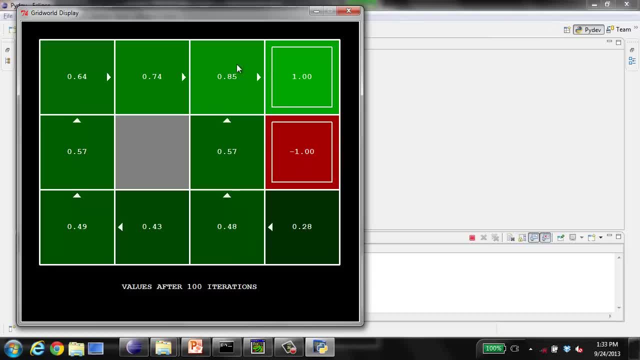 and you get a minus 1.. But what's this 0.85?? This 0.85 here is the average score you're going to get if you act optimally, Which, in this case, you can see. you can guess that. 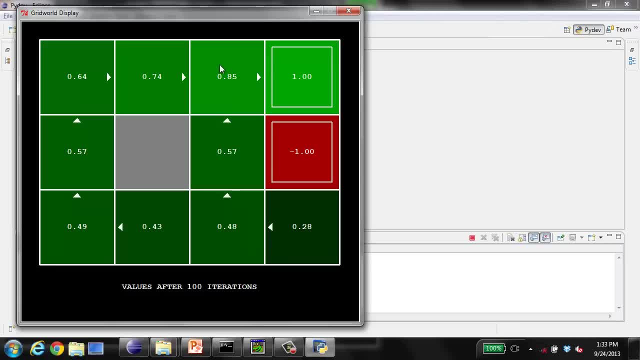 these arrows are the optimal policy means trying to go east. Well, maybe you'll go east and then you'll exit, Or maybe you'll slip and you'll go to the south, And at that point you'll then try to go north. 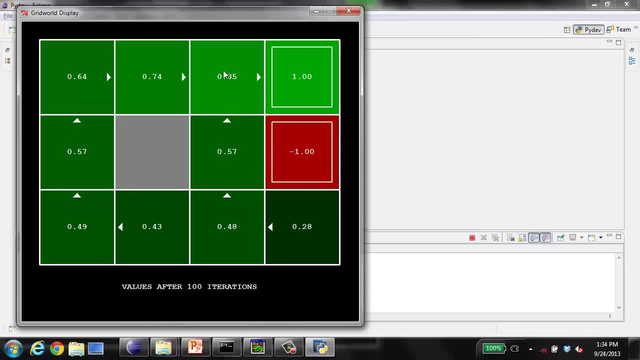 Which maybe your order is ongoing north, or maybe you'll fall into the pit and so on. So this 0.85 rolls all of that up. You could think of this 0.85 as being the expect-a-max value. 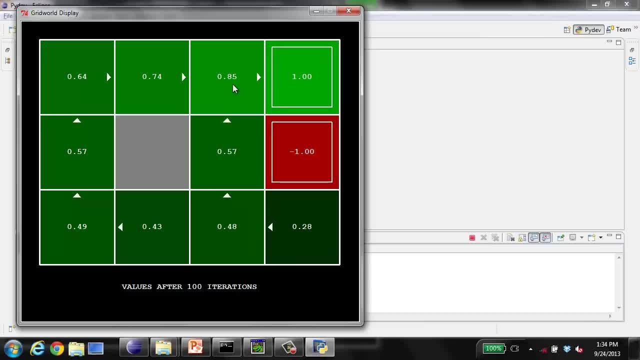 like if you run expect-a-max from the state. You could also think about it as somebody handed you the optimal policy and said what will happen on average if I follow this policy. Of course, there's exponentially many things that might happen, but if you added them up, weighted by their probabilities, 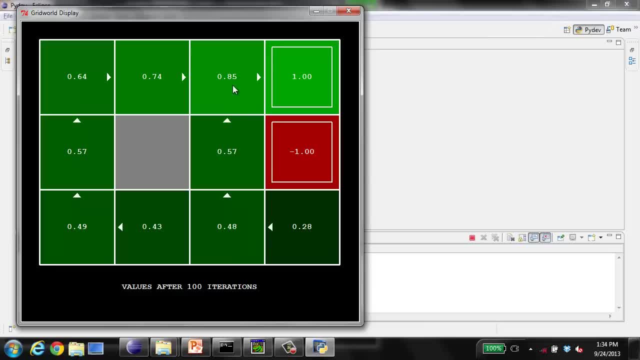 you would get 0.85.. Both of those computations are equivalent. Okay, let's see what else we can see here. Down here, 0.28, this is the worst square in terms of value. Why, Why is this so bad? 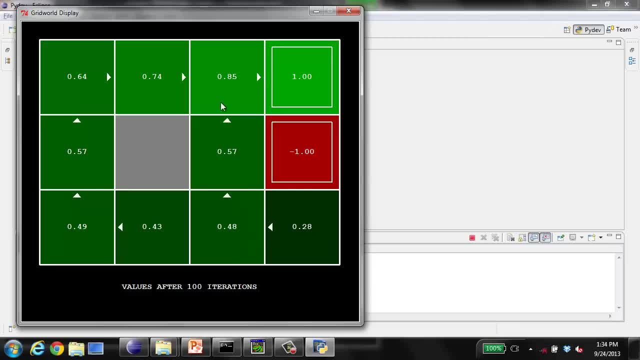 Well, one, you might fall straight into the pit. Two, even if you've got to make it to the good reward, it's going to take a while. So it's both the fact that you've got kind of some short-term bad outcomes under this policy. 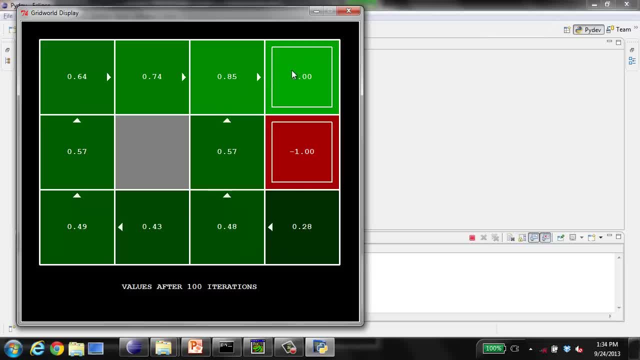 and the fact that that living reward is slowly chipping away at your value. this is not a good square to be in Now. of course, even bad squares to be in have optimal actions to take. The value doesn't tell you what to do. 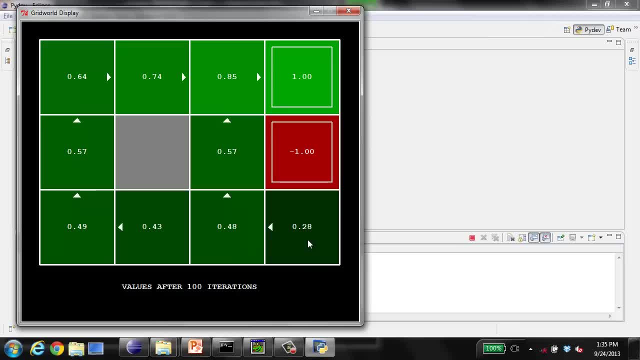 it just tells you what your average score is going to be if you start there. So if somebody gave you the choice, you wouldn't want to start here. If you're there, what does the value do? Well, it doesn't really do anything. 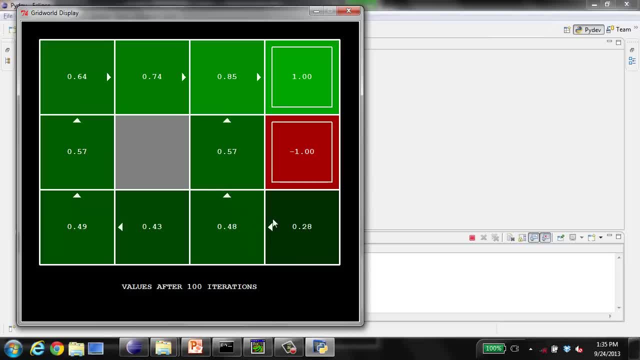 It's a quantity that you compute along the way when trying to figure out what you should do, so it's just like a minimax value. If the minimax value is high or low, you know, that's kind of how good the world is. 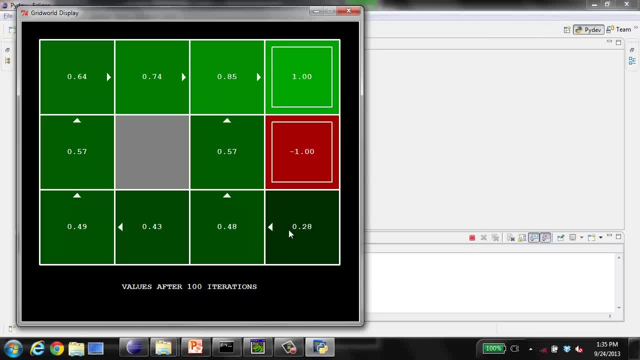 It doesn't tell you how to act. So these are the values, and we'll talk about how to compute them. What does a Q value look like? Well, let's take a specific example so we can see: Okay, how about here? This is a good example. 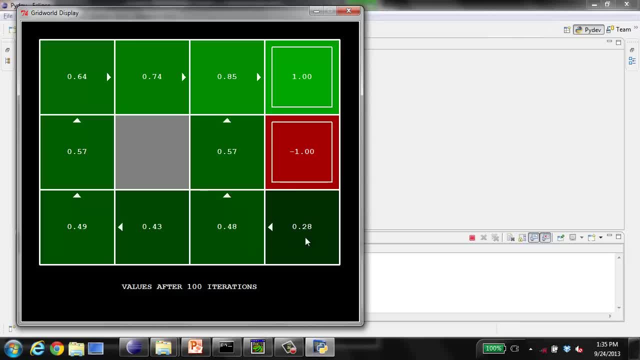 It's .28.. Its value is .28.. If you think about the expectamax, we're in the state. what can we do? We could go east, we could go west, we could go north, we could go south. We could kind of chug all the computations. 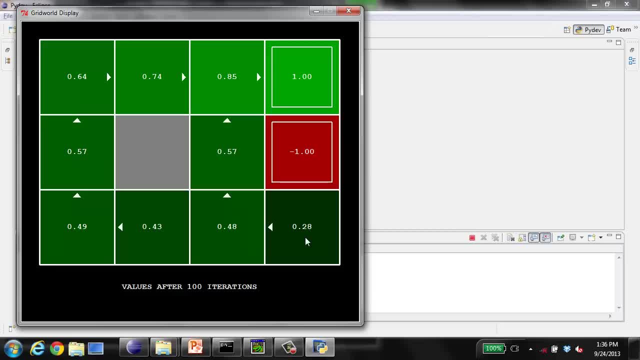 Going west is the right thing to do, What's probably the worst thing to do. North is probably the worst action. So going up is a bad idea, and you're probably going to end up with something like negative one if you go up. 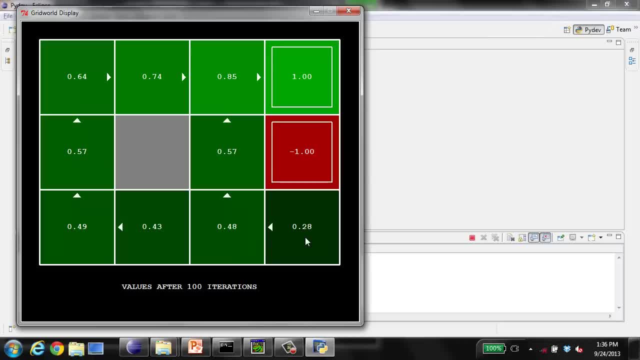 If you go west, then you're going to end up apparently with .28.. If we break out not just the value of the state, which is the value of acting optimally from the state best action, and we fix the action, then suddenly this state now has. 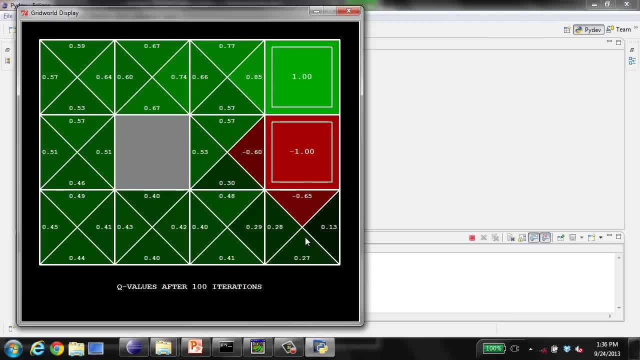 four different numbers. These four numbers are the values- remember expectamax value- if you commit to that action but thereafter act optimally. So you can see, for example, if you commit to north but then act optimally. well, what are you going to do? 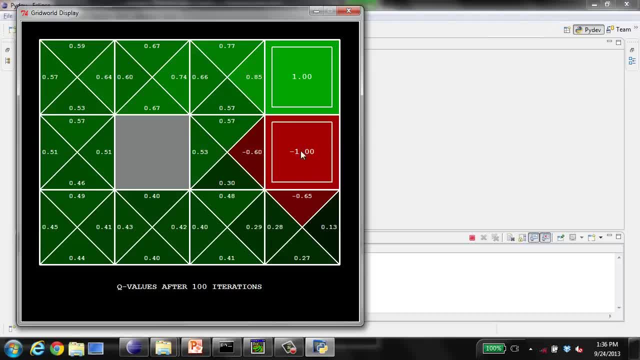 You're going to lose a living reward. there's going to be some discount, then you're going to end the game. So the Q value for this Q state is low. but the Q value for this Q state is reasonable: it's .28.. 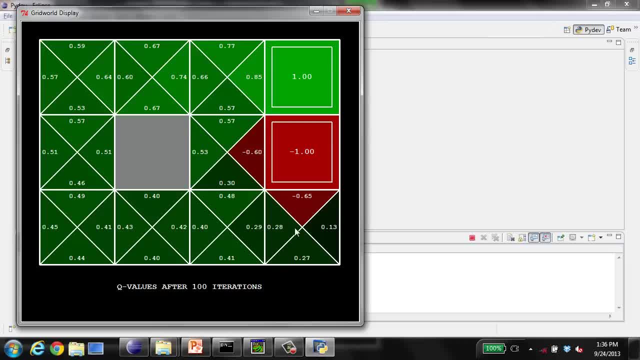 It's not a coincidence that one of these Q values equals the value, because the value is just a max over all of the actions you can take, meaning the value is going to be the maximum of one of the Q values. Any questions on that? 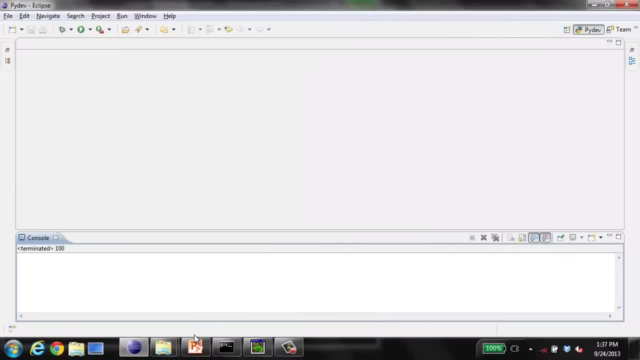 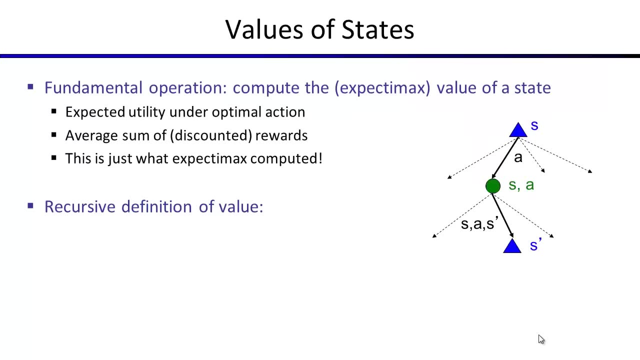 Just kind of visualizing some of these values. we'll see some other values later. So values of states. This is a fundamental operation we need now to work for. This algorithm is going to compute the expected max value of a state. That's the expected utility under optimal action. 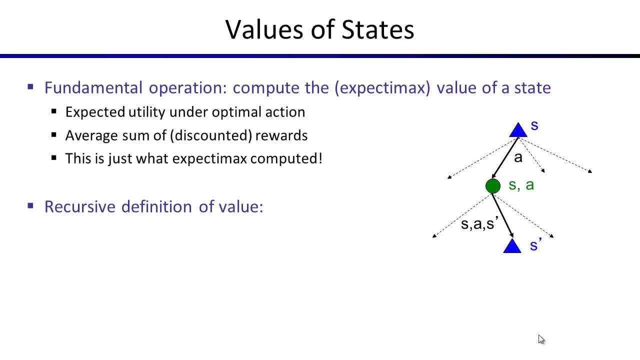 That means it's going to be an average sum of discounted rewards with kind of the appropriate actions taken at every place, And it's what expected max computed. So if I say here's an MDP, go compute me the values. what you could do is 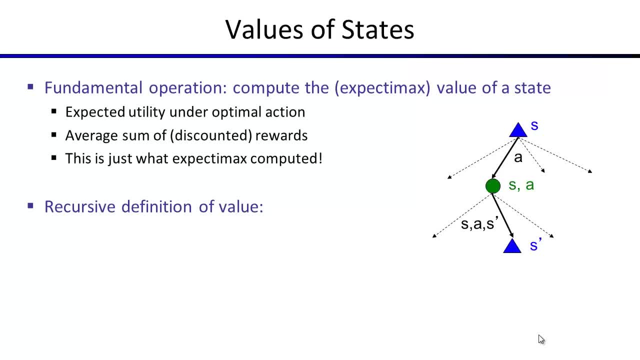 you could say: okay, wait a minute. you could go state by state and for each one you could launch a little expected max and use it to compute the value. This would work. There's actually two problems with it. Why would you not compute the values? 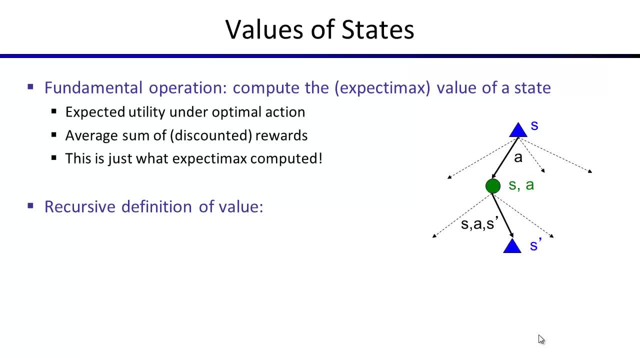 of all the states by running lots of expected max. One problem is there might be a lot of states You're going to have to run expected max over and over, and surely there's going to be some redundant work. Secondly is if you'll remember these games. 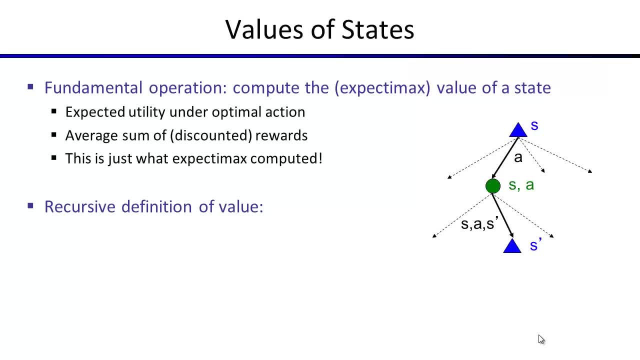 can last forever. Expected max is exponential in its depth, And so what happens if you set the depth to infinite? Bad news: Even a single expected max won't work in an infinite game, and even if you somehow had a way to do that, there would be a lot of wasted work. 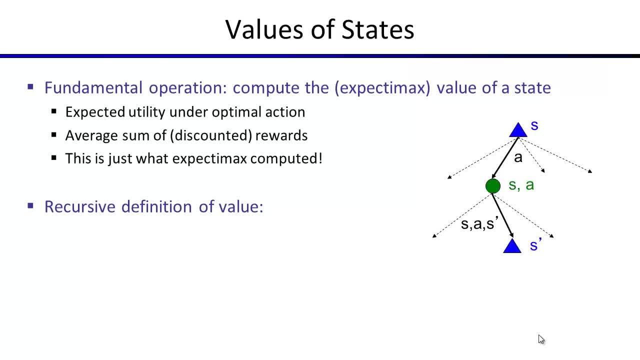 between the different states, because they share a lot of structure. So instead, what we're going to do is we're going to write down our cursive definition that captures what expected max does, But then we're going to reorganize the computation in a bottom-up way so that we don't waste. 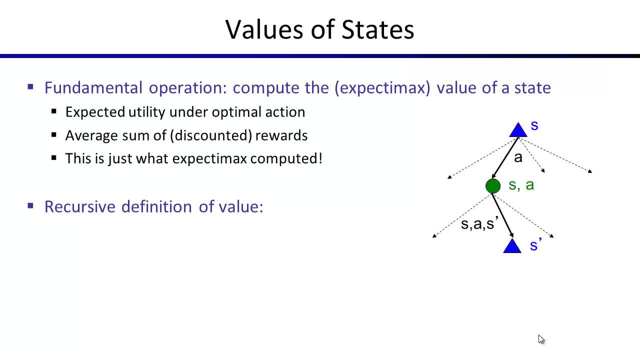 work Okay. so what's the definition of value? Let's actually write this out. Let's talk about a state. So if I want to say what is the value of a state, So that's v star of some state s. 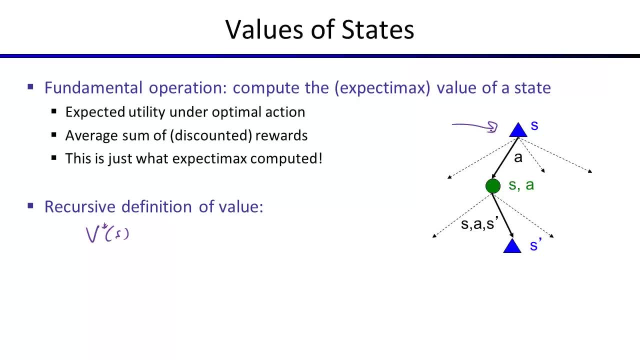 Well, we think back to what would expected max do on this tree. Expected max would say: well, the score you're going to get from that state depends on which action you take, And you should take the action that gives you the biggest score. 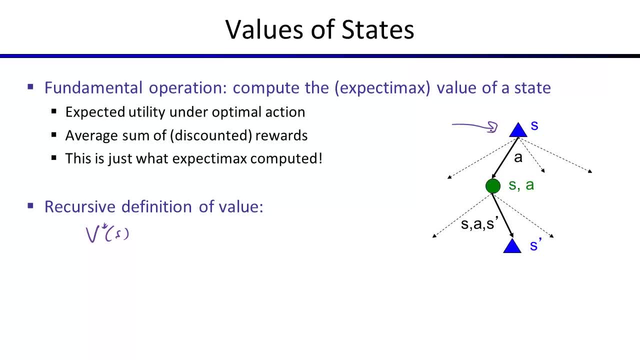 How would you do this if you actually implement your project 2?? How do you implement this? Well, you loop over the children and for each one you recurse Right. So how do we write that in an equation? We say the value of a state. 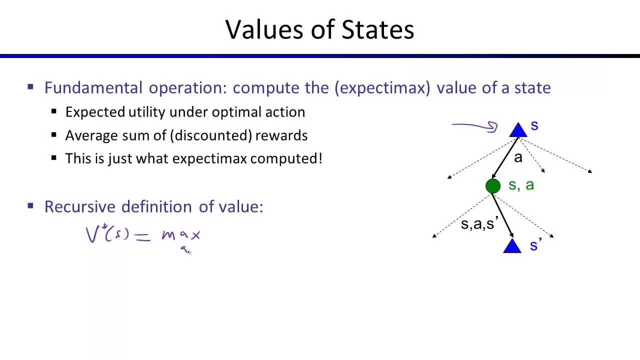 is looping over the children and taking the max. We write with a max And then we recurse. Well, we recurse in the code to a chance node, And that here is the q value. So it's the maximum of all of the chance nodes. 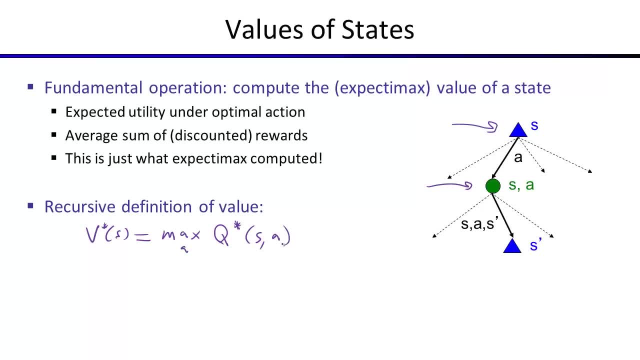 which are q states s a, It's the best one. So this equation here, even though it's got this q that you're still building intuitions for, this just says it's the maximum of the children. Easy Max nodes are simple. 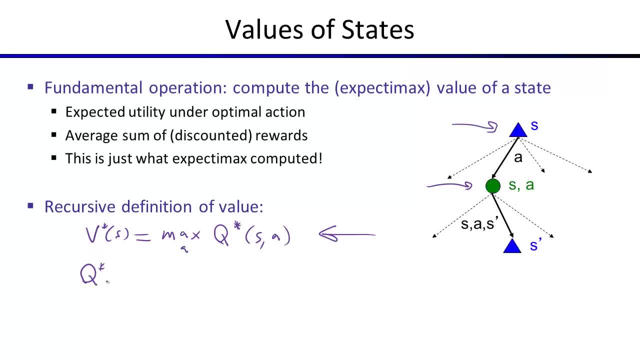 What is the expectamax value? What would expectamax return from a q state, from a chance node? Well, you can think about that. You're at this green node here and you're doing expectamax. So what does expectamax do? 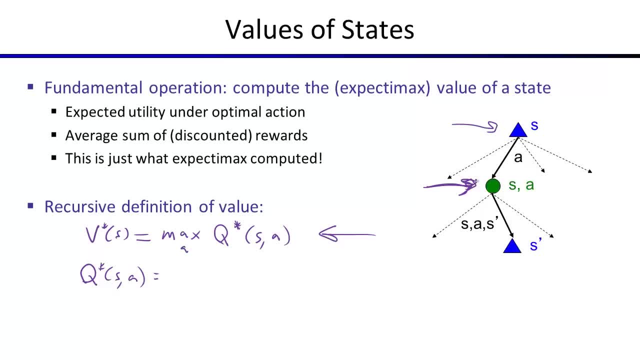 It visits all of the children. it recurses to that child to see how good that child is, and then it averages them together. So how would we write that? Well, we have to visit all of the children, So we're going to go to each one of these. 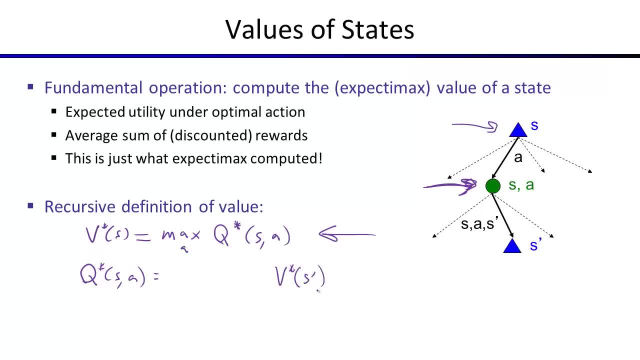 children s prime and we're going to compute its value. So that's some function. call to v star of s prime. Okay, so we compute all the children's values and then we average them. Well, what does that mean now? 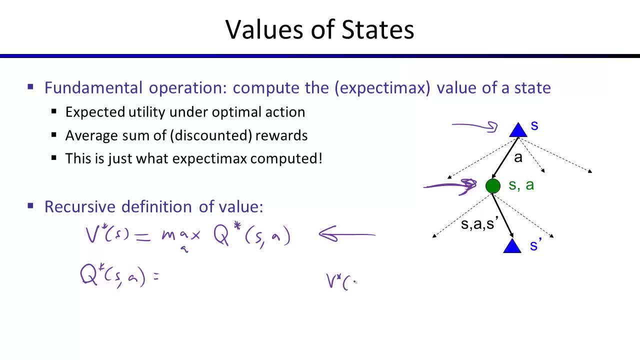 Let me move this over here. What is the probability that this particular s prime is going to happen? Right, it's given by the problem, And what is it? It's the transition function. Good, Okay, so what we're going to do is we're going to do an average. 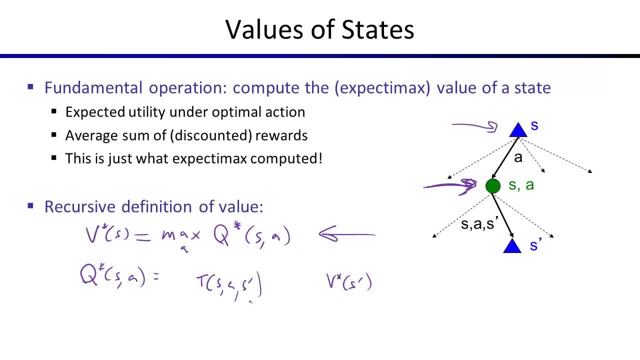 for each s prime. We're going to look at how likely it is according to the transition function and we're going to add those up. So we're going to add up over all s primes: transition function, times, value of the child. If it were like this, it would be: 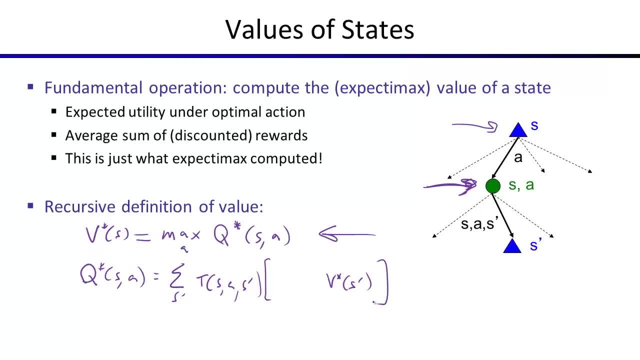 just like expectamax, This is max would be a max over the children and q would be an average over the children. But remember there's one more change between expectamax and an mdp, And that is you get rewards at every step. 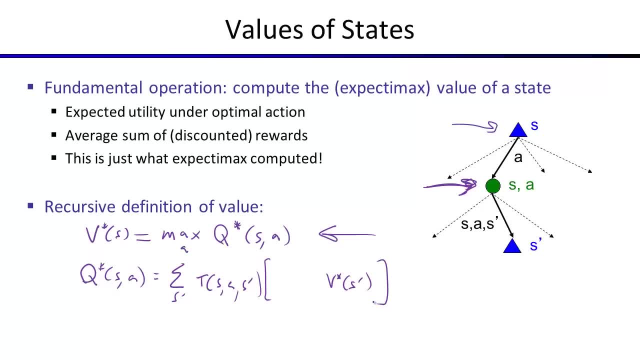 And so, when you go from s to a to s prime, in addition to having a probability of this outcome and in addition to having a future value of v star, you have an instantaneous reward. So, at that very instant you get the reward: r s a s prime. 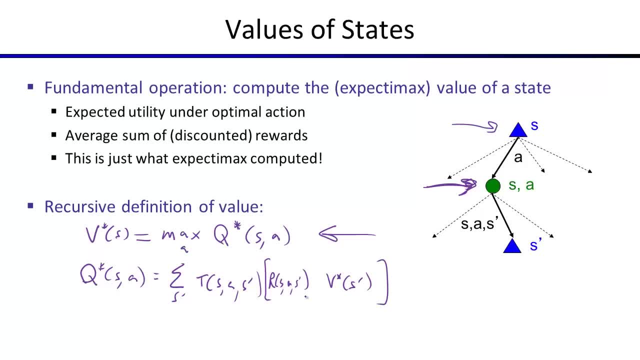 Okay, so you have to average over the possible s primes. For each one, you look at the instantaneous reward plus the future reward, where the future reward comes from this recursion, And if you remember, there's one more thing, which is that there's a gamma that discounts the 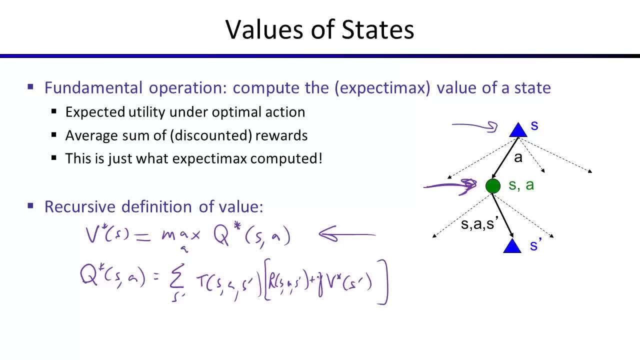 future by a factor of gamma. every time step into the future, And because s prime is one time step into the future, I get one gamma. So this is it, Okay. here's your occurrence for max, here's your occurrence for the average. 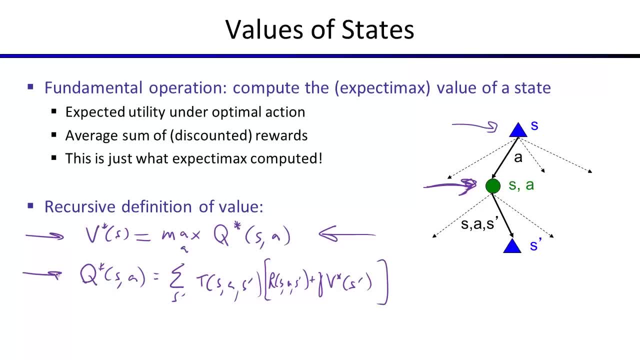 and it's a little bit complicated by this fact that there's instantaneous rewards along the way. Yes, If you're going to average over s prime, why not divide it by s prime? s prime's not a number. You mean divide it by the number. 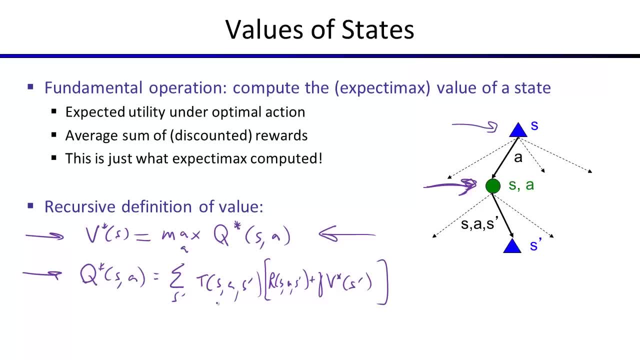 of s primes. Yeah, so that's already in t. So if there are two s primes that are possible, each one will be 0.5 if they're equally likely. So t already is a normalized probability distribution. Okay, so I'm going to. 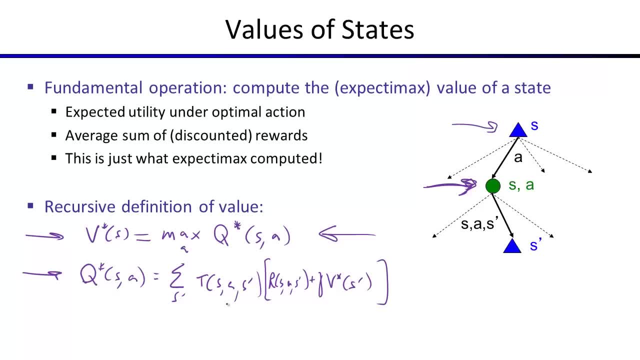 any questions on this before I replace it with nice pretty latex instead of my handwriting? Okay, Okay, so the value is a max node. It's defined in terms of a chance node. The chance node is defined in terms of the max nodes with an expectation. 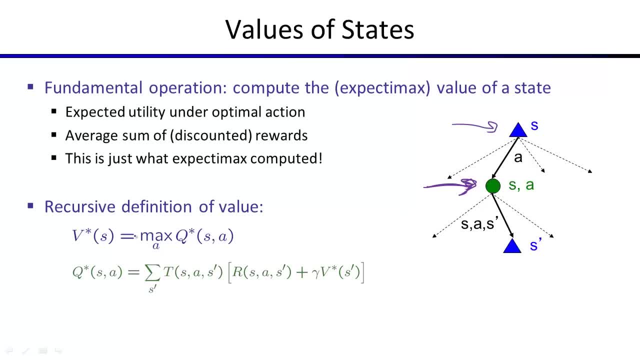 just like expect a max and reward plus discount in future. Okay, that's breaking your future up into what happens in the next time step and then a recursive call. You can kind of inline this and you can write this without any views. 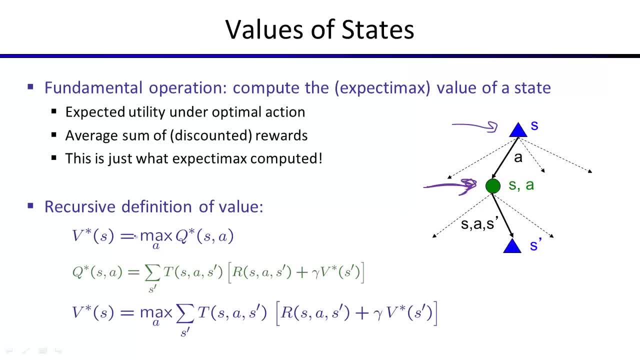 So if the views offend you, you can write this equation that says: v star of s is a function of other v stars of s. Okay, Now this equation is actually the standard form. This is something called a Bellman equation. We'll talk about this later. 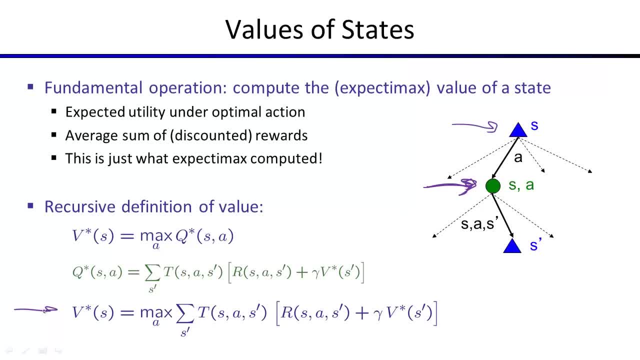 But it's kind of an eye fool. So if you look at this, your chance of symbol shock is high. So what you want to do whenever you think about this is you want to think, when I see a max, that's this for loop here. 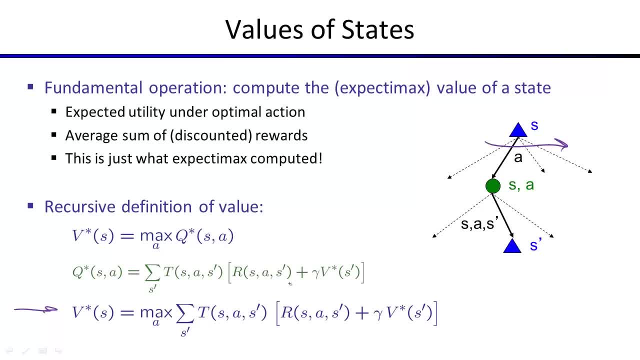 The for loop that loops over all the children, And when I see a sum of that's weighted by t, that's looping over the possible outcomes of the chance node, And so if I want to go from a state to another state, I need to consider. 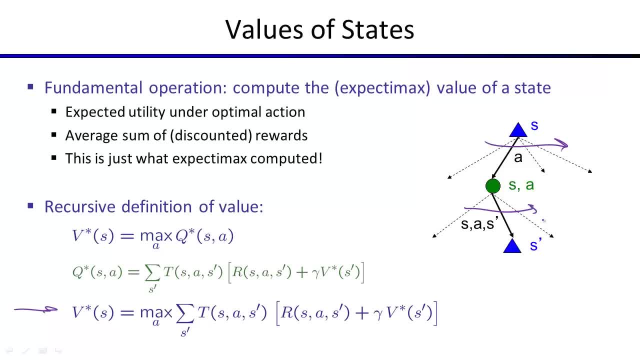 my action, which is the max over actions, and the outcome s prime, which is an expectation. Okay, So we're going to see a bunch of variants of these things. They're unfortunately going to look a little similar, but the reason they look similar 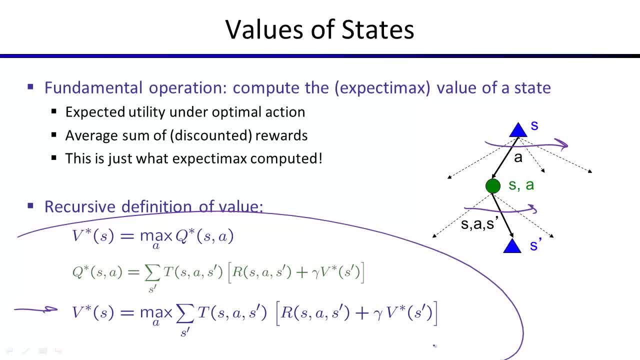 is because it's that same expectamax calculation over and over again And in some sense, it's often easier to be able to reconstruct these from expectamax than to memorize them, because, again, they're pretty similar. Okay, Let's look at the search. 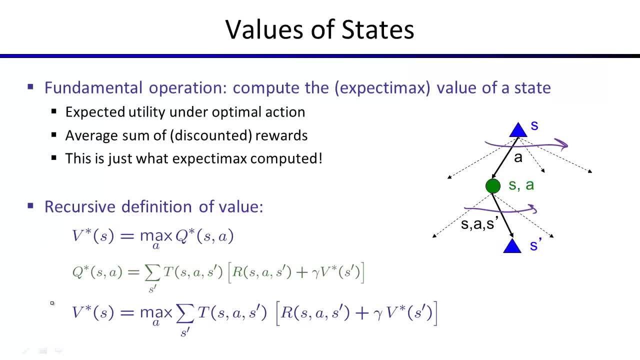 tree. So what I just wrote here, these equations, these are definitions. This is not an algorithm, Right, Because they're the same variables on the left-hand side and right-hand side, and that means, if I executed this as a recurrence, there's. 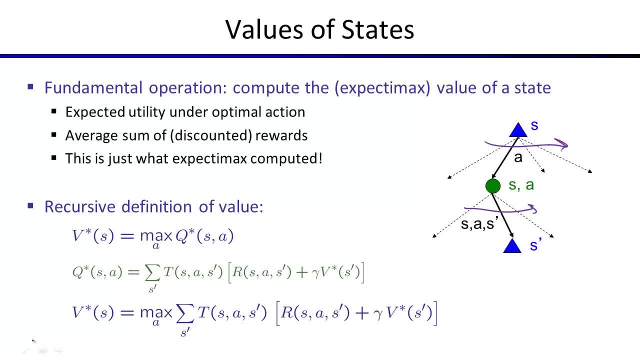 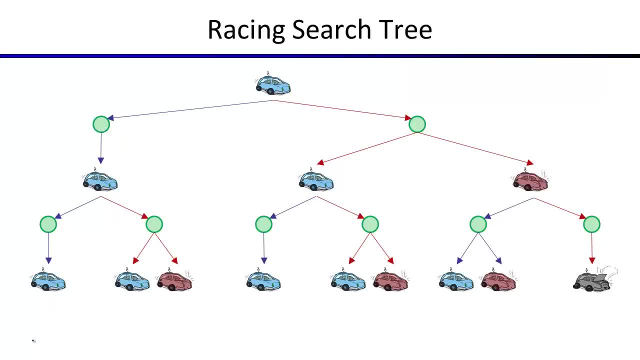 no guarantee it would ever terminate And in fact, for the car problem it wouldn't terminate. So this isn't an algorithm, but let's think about what the racing search tree actually looks like. Okay, So at the root we've got the current. 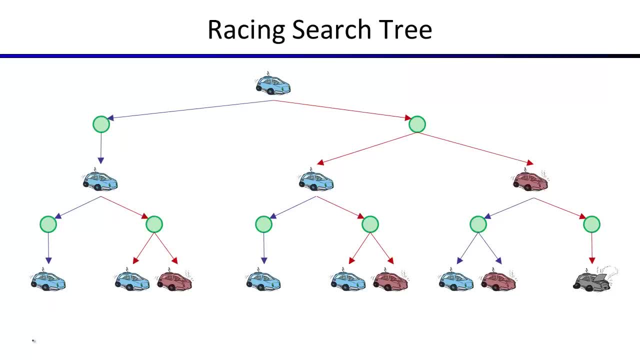 state. Right Underneath that we've got two Q states that correspond to the two actions we could commit to, and those states have kind of one or more resolutions, and then we're back to states. So here's the racing search tree. We could run expectamax on it. 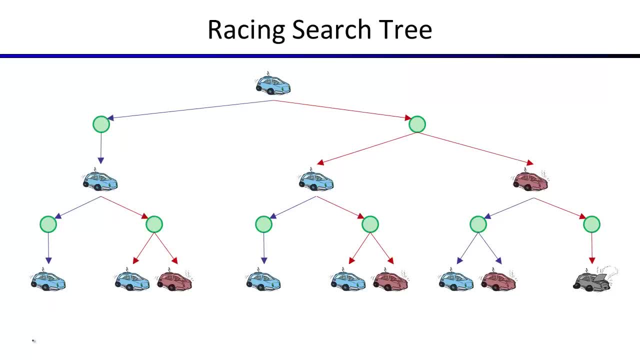 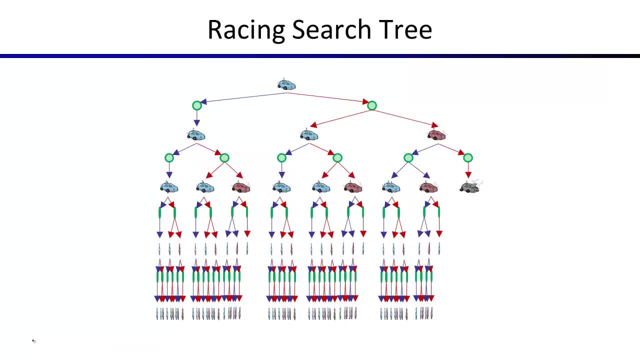 We couldn't run it to infinite depth, because this game goes on forever. but there you go. Let's go down a couple more levels. The search tree is starting to get kind of. you know, the branching factor is not that great, but if you go down deep enough there, 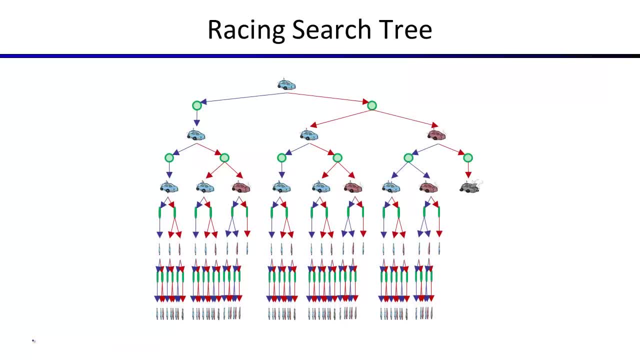 start to be a lot of states. Okay, But how many states are there in this problem? There's three. In some sense, it's crazy that we've got a search tree that's getting exponentially large when we've only got three states in. 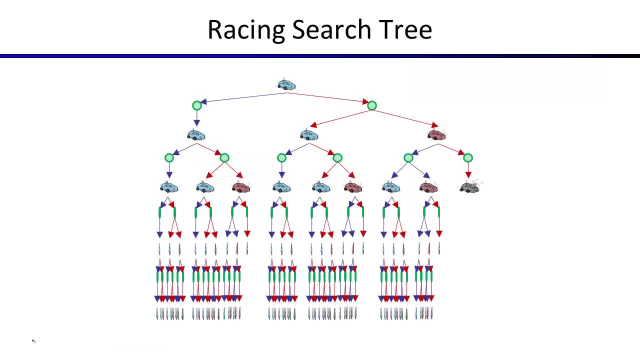 our problem, And so there's a lot of repeated work. Right, If you think about executing expectamax from here. right versus from here, it's the same expectamax computation. So one thing that's wrong about computing expectamax from a tree like 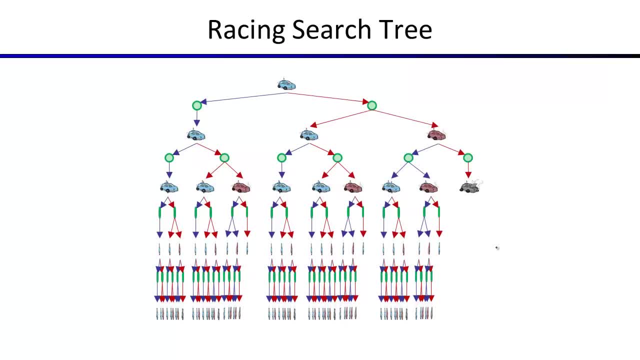 this is because if the states repeat, you end up redoing their expectamax computation. So at one level you could say: we can just fix this. We could just kind of hack a fix into this, We could put in, we could do some memoization and say, if you ever ask, 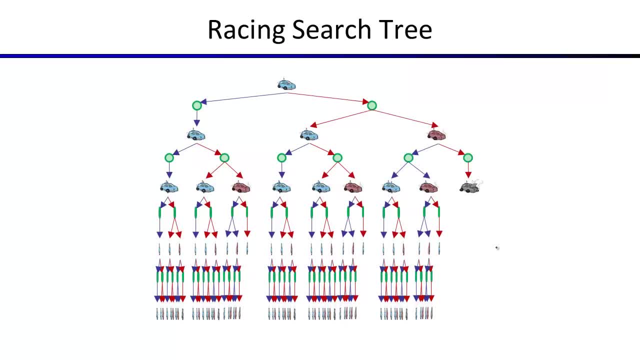 me a question I've computed before. I'm just going to return the answer, And actually that would be fine. That's 90% of the algorithm that we're going to do. We're going to do expectamax, but we're going to avoid doing. 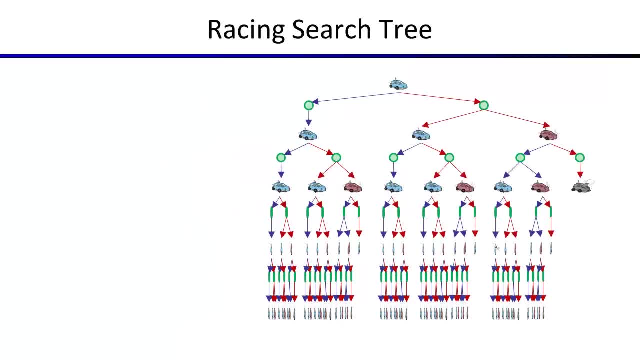 computation, except we're going to organize it differently. Okay, Let's look at the search tree. We're doing way too much work with expectamax because the same states are reappearing, And so instead, what we're going to do is we're going to compute the quantities we need one. 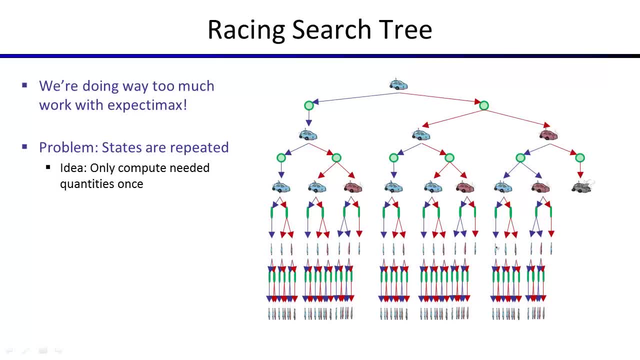 But rather than just let kind of memoization starts us out on the fly, we're going to write down all the quantities that we're ever going to need, and then we're going to compute them one by one. In essence, what we're going to do is, rather than starting at the 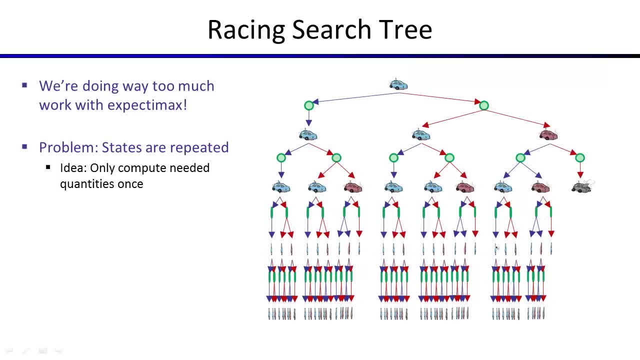 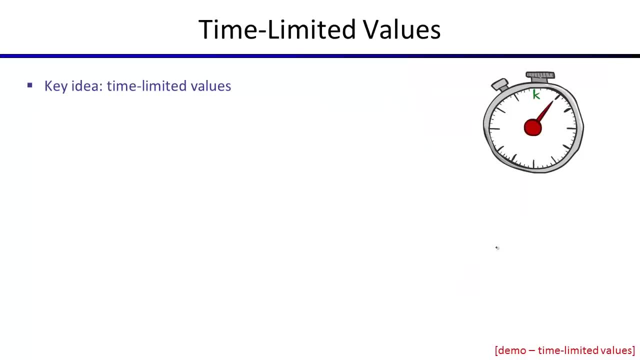 top and working downward. we're going to start at the bottom and work up in a dynamic program. Okay, So yeah, and the tree might be infinite and that would be bad. So we'll talk about how we fix that later, But first let's 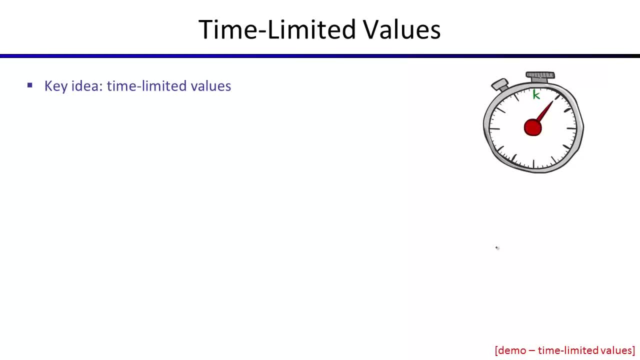 just deal with this repeated work issue. The key idea behind this algorithm we're going to see- and the algorithm we're going to see is going to be called value iteration. The key idea is called time-limited values, So you can think you have a. 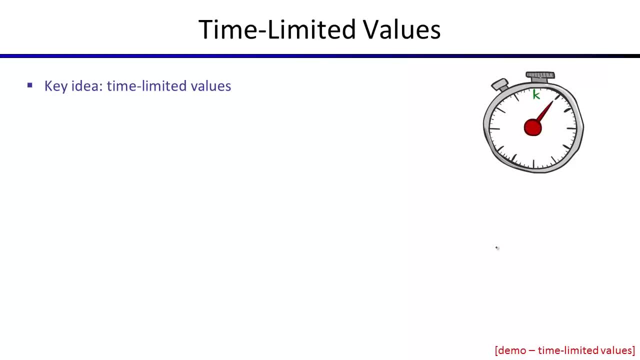 stopwatch that has k more time steps, and then the world's going to end. Okay. So why is this good? Well, if there's only one time step, computing values is easy. You don't have to think about the future at all When there's. 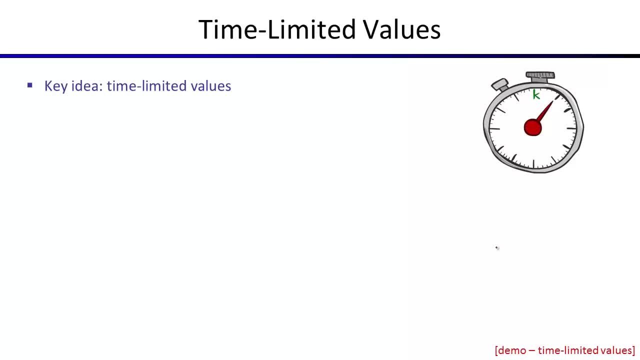 two time steps. it's not that hard, Right, And so what you can do is you can imagine just doing kind of deeper and deeper computation. We're going to define v sub k of the state. So remember v is the value under optimal play. 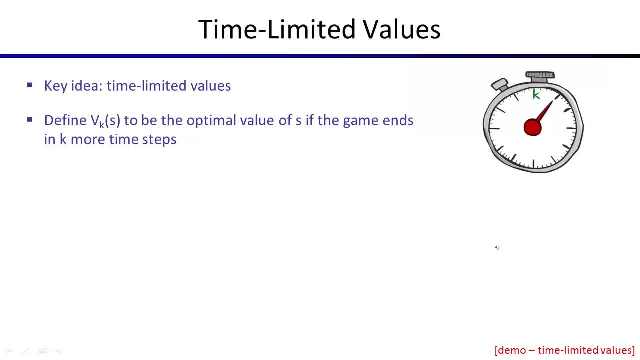 s is a state and we're going to define v sub k to be the optimal value if the game is going to end in k steps. Okay, Equivalently, it's what depth k expecta max would give, Because in expecta max 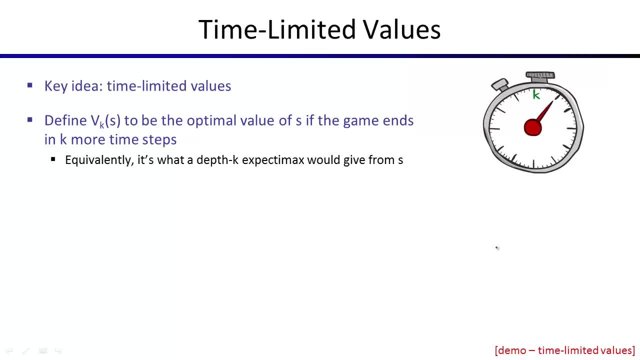 you consider kind of k layers and then silence right. So if we computed this right, the step search tree, if we computed this, this is a depth to expecta max and we would say the result of that computation is v2. 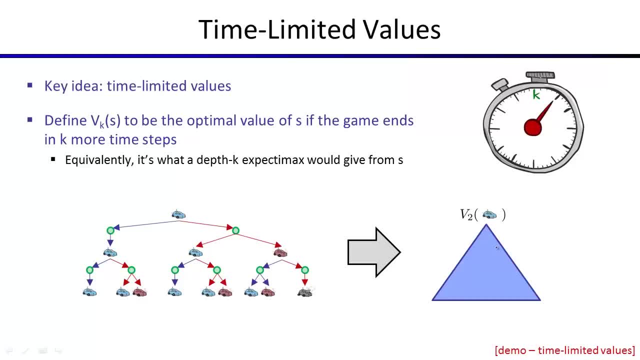 of the root state, which, in this case, is cool. Okay, So what we're going to do is we're basically going to compute all the v1s and all the v2s and so on, so that we don't have to repeat any of those computations. 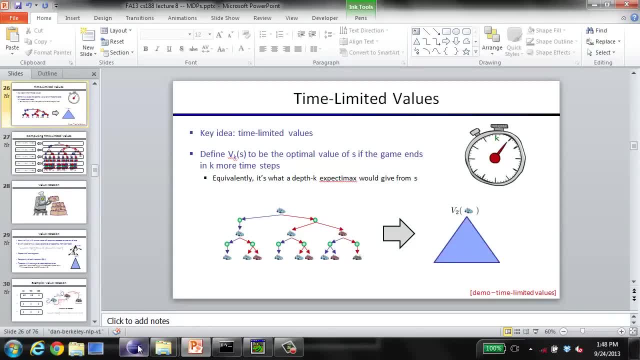 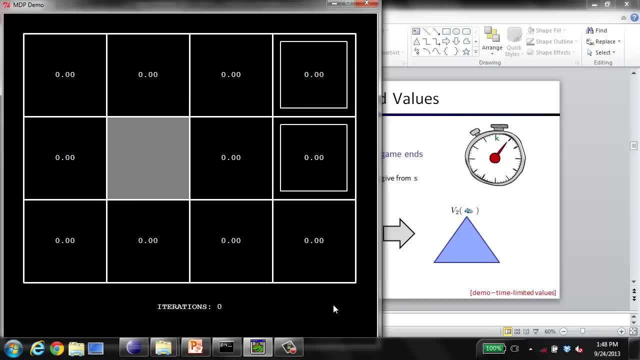 Let's actually look at what we're computing before we see how to compute them. So here are depth limited values for the grid Right, remember, some of them are green, some of them are red. Now they're all black, they're all zero. So what depth. 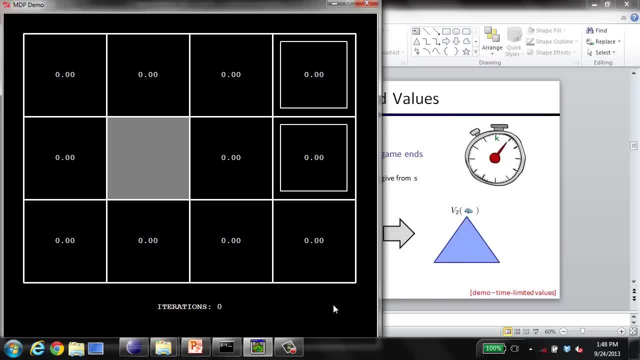 is this: This is zero. This is the value you're going to get. that is the expecta max score under optimal play. if you have exactly zero time steps left, meaning nothing will happen. What if we have one time step left? 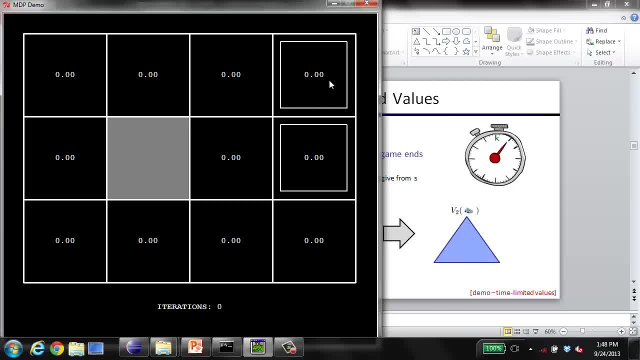 Well, if we're in the good exit up here in the upper right, how? what will our average score be in one time step? It'll be plus one, and it will always be plus one, because there's only one thing that can happen. Similarly, if you're in the 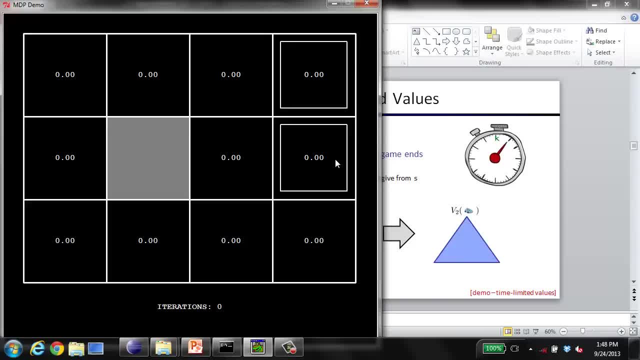 pit of death, then your average reward or your expecta max value will be plus one. How about? if you're right here, You're right next. you're one step west of the good reward. What can happen to you in one step? 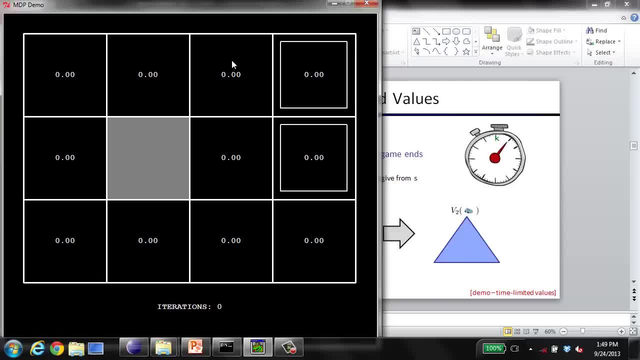 Well, you can get to the good square, but you can't exit. So you'll still have zero if there's zero living reward. So in this case, I set the living reward to zero In one time step. you can see the. 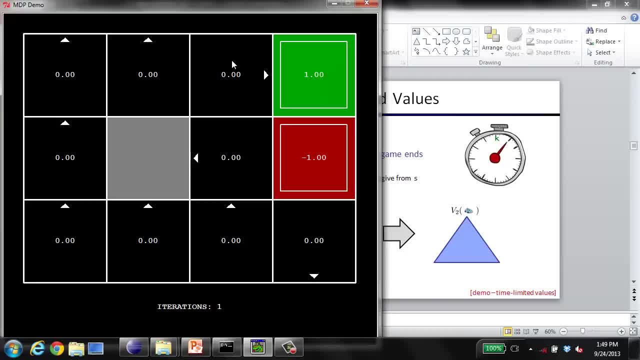 only squares in which you'll see a reward are the squares that are one step. exit away In two steps. where can I see a reward? Well, if I'm right, here, next to the good exit in two time steps, I can move to the east. 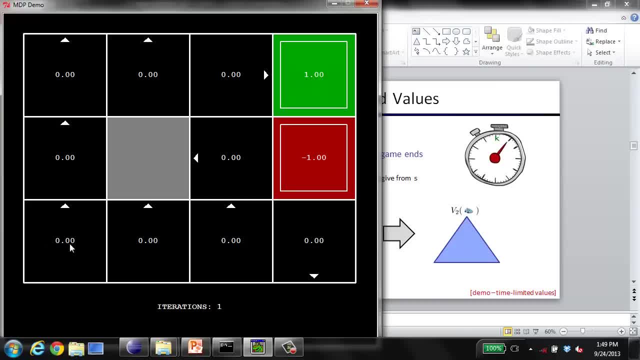 and then I can exit. But if I'm over here at the start in two time steps, I still can't get to any non-zero reward. So if I go to values v2, these are the optimal values in two time steps Now. 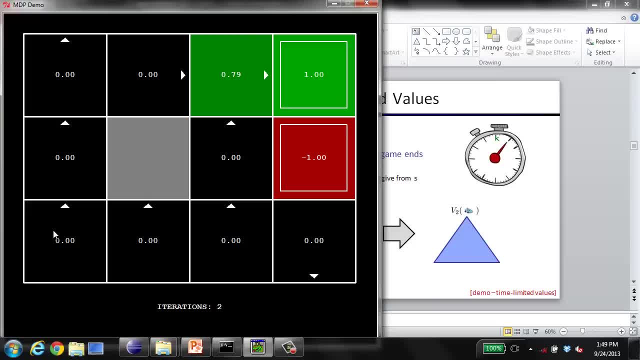 0.79 there. that actually has two components. There's two reasons why it's less than one. One is any living reward that might be in play- although here the living reward is zero. A discount, if a discount is in play, and also 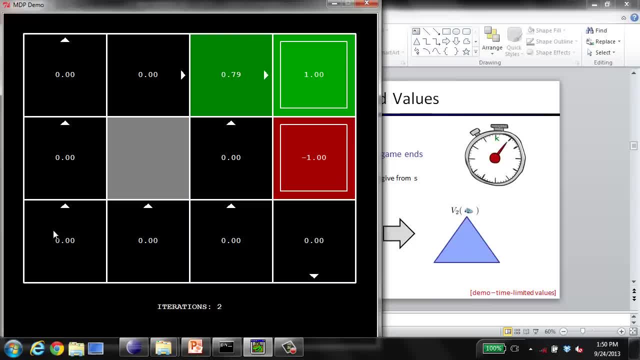 the fact that, even though you can get a plus one in two time steps, you might not because you might slip. Okay, so if I go three time steps, you can see that 0.79 has gone up to 0.87, and you can see if I go. 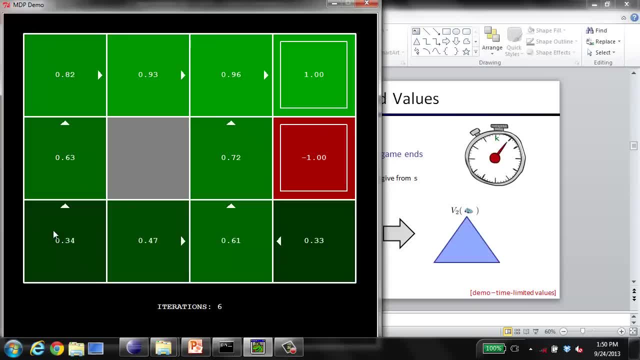 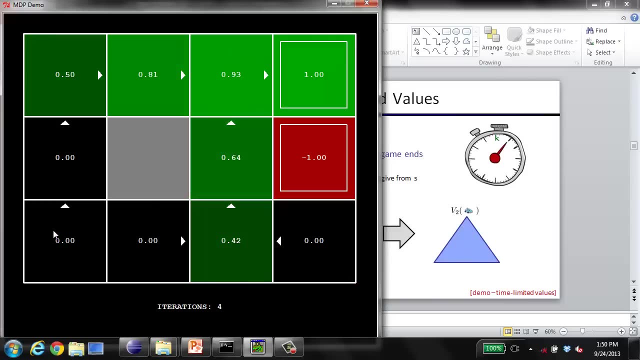 to four time steps, then five time steps, then six. the longer my horizon is in my search, meaning v, sub k for larger k, the far away from the end state I can start to see rewards. Yes, Why do the lower? 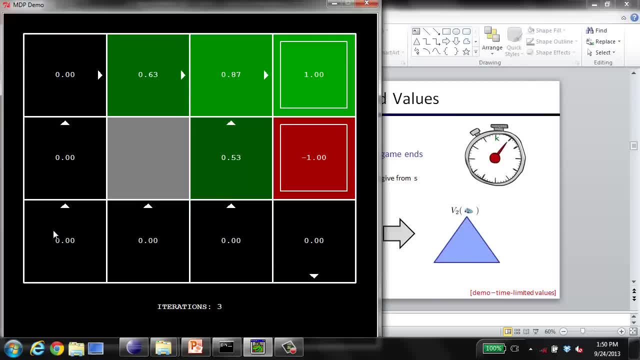 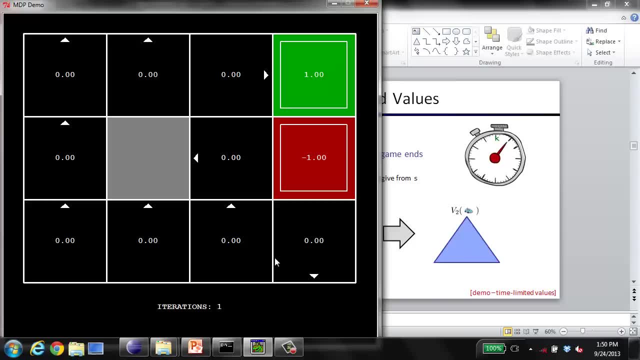 Okay. so right now, if we're talking about the lower right in one time step, what's the best you can do? Zero In two time steps. the best you can do is zero. In three time steps. the best you can do is zero. 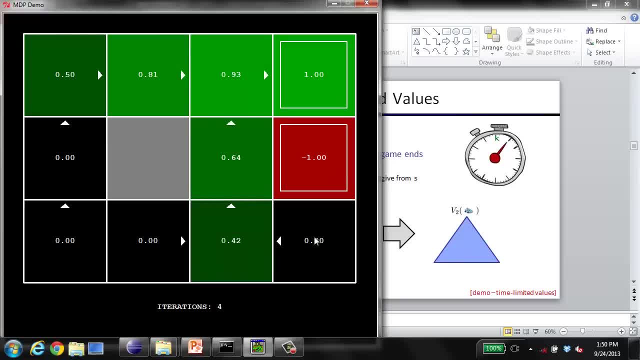 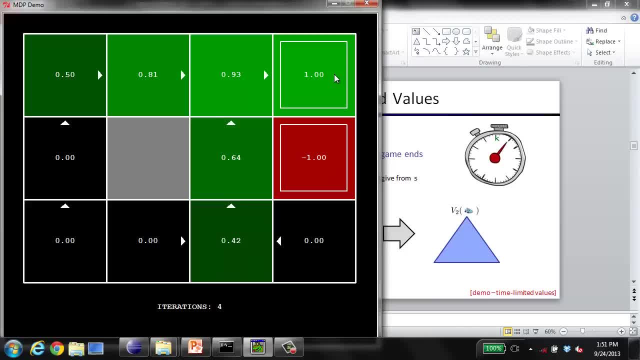 plus one, It does have a score and it scores zero. That's right. If I re-ran this with a living reward, there'd be kind of minus .4s everywhere. You can see how the information propagates out as the depth increases, and here's what it will. 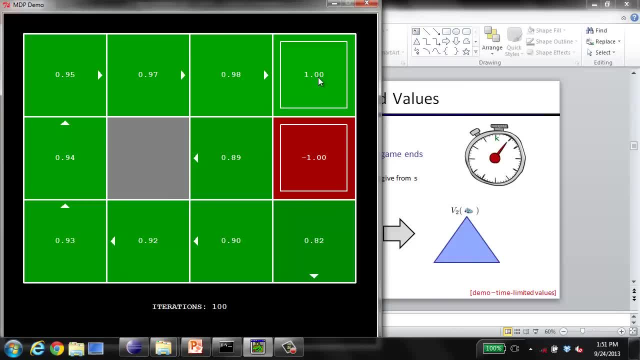 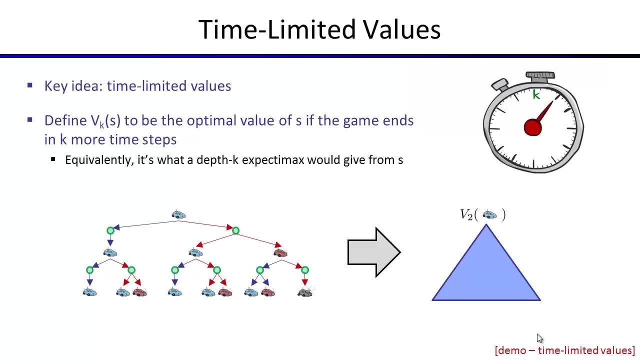 converge to. If you look at this, you can actually see what's going on. You can see that there is a discount, and it's a very small, sorry. the discount is very near one. Okay, So let's think about how to compute those Well. 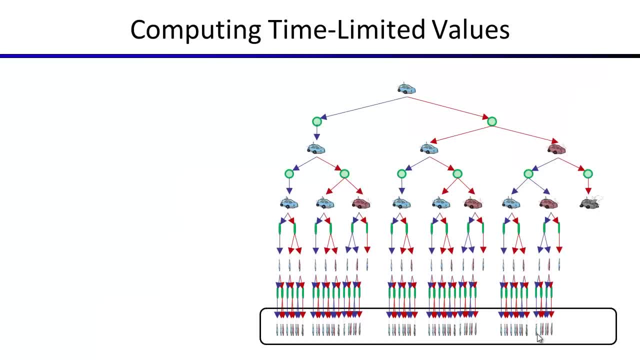 computing them actually turns out to be pretty easy, at least for v0.. Because in v0, you're at the bottom of the tree. You have zero rewards left to come. Zero time steps means zero rewards. to sum up, So v0. 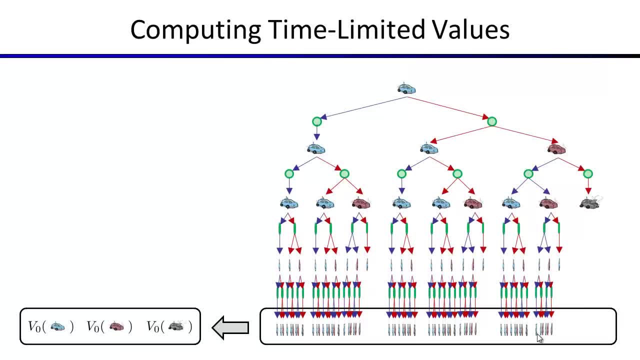 is easy. it's all zeros and we can compute v0 for each of our three states. There aren't that many states, so it's easy to do. How about v1?? Well, if you think about this, this tree may be very large. 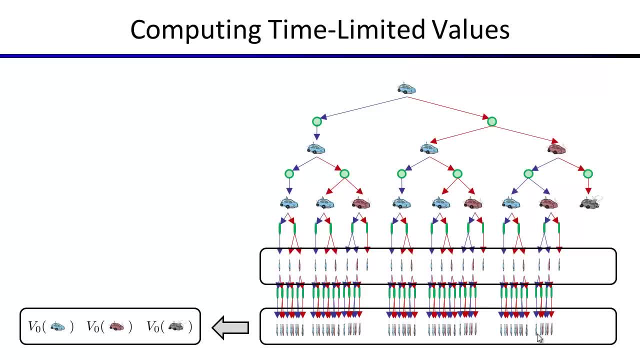 but there's only three, and so the vectors of values that I can get at this level of the tree. there's only three numbers, They just reoccurring. Similarly, if I go up here I can compute v2.. Those are expected. max searches of depth: 2,. 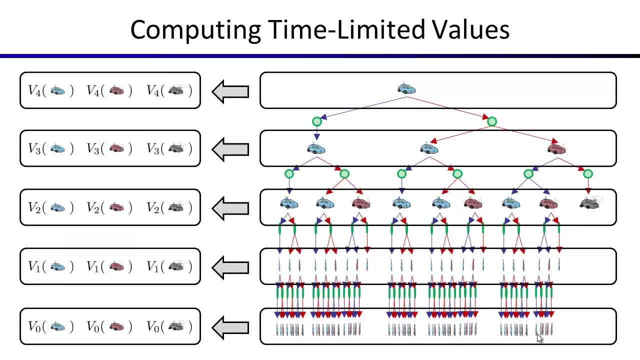 and again, there's only three to compute. There's only three to compute at this layer and there's three to compute at the root. Okay, There's actually more work at the root, but this way I'll get the answer for all states. 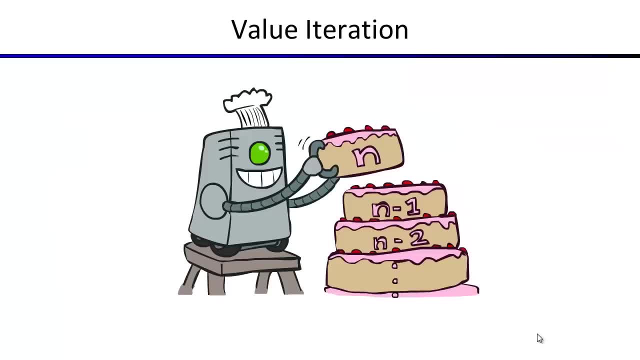 So how do I compute these? Well, it can be like building a cake: You start at the bottom, And so you start at the bottom with v0,, and presumably that's not good enough for you, so you compute v1.. Presumably that's not. 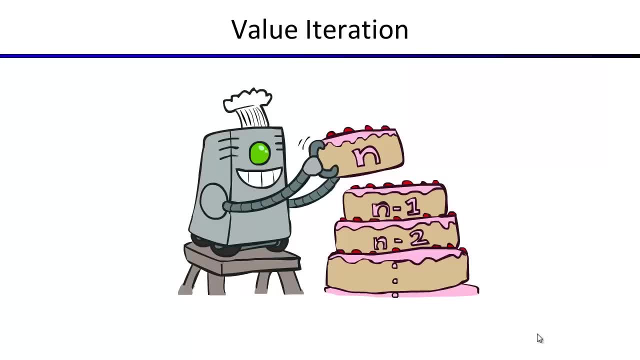 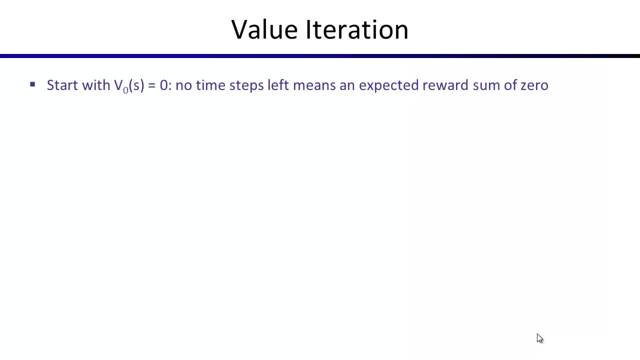 good. you compute v2.. And at some point around v100, you say: these are good enough, I'm gonna stop, Let's see how that works, how it goes. Now I'll go ahead and call value iteration. You start with v0,. 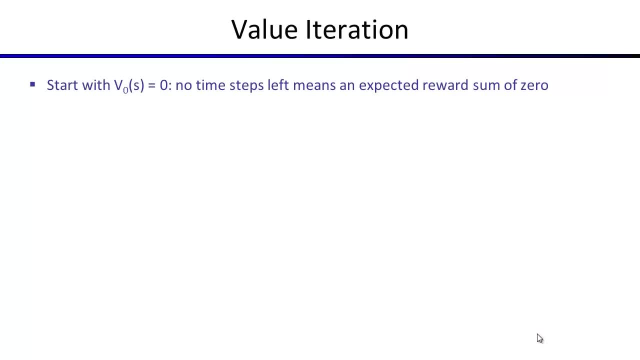 which is always zero. Okay, Unlike expected max, where at the bottom there are all the good numbers. right in a game the bottom is zeros. When the game ends, it's done, There's no more rewards. You were kind of handed your rewards step by step. 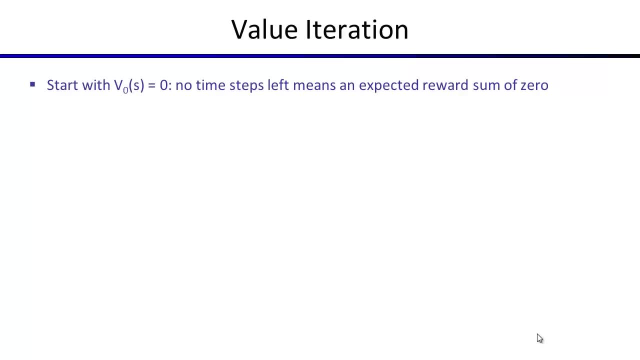 So v0 is, by definition, zero, And that's not a single number, that's a vector. There's one of these v's for every state. It's a vector for each state. Sorry, it's a vector containing an entry for each state. Okay, Then 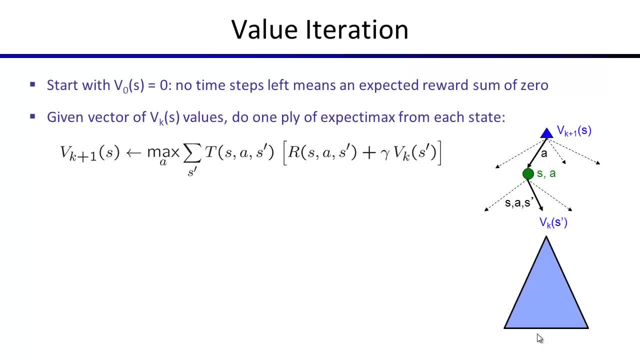 I give you some current v-whatever. So at the moment you've only got v0, but at some point you will have computed v7.. When it's time to compute v10,, you've got v9, sitting there waiting, In essence. 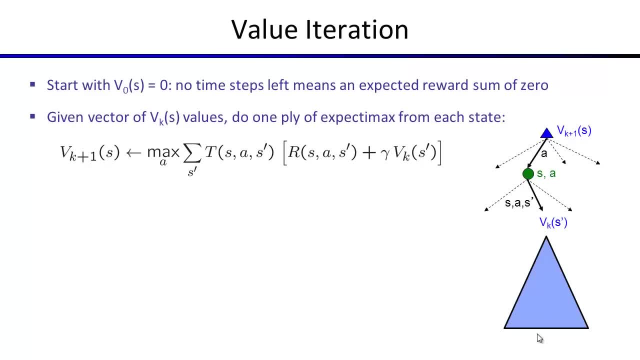 when you compute v10, you've already done the depth 9 expected max values, though you've done them in this value iteration way. So what do I do When it's time to compute vk plus 1, I think, well, what is this? 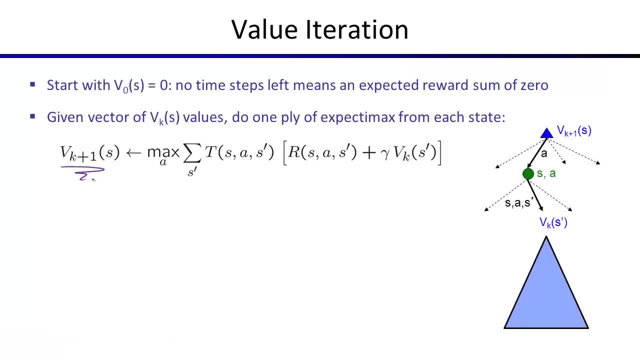 thing. What is vk plus 1?? It is the answer of an expected max search of depth: k plus 1.. Well, how would I do it? Well, here's my expected max tree. So for this state, vk plus 1 involves: 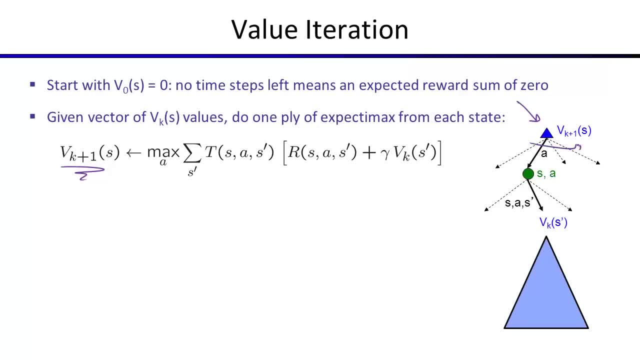 I need to loop over all of my actions a and pick the best one, just like expected max, That's this max right here. For each action a, I need to consider all of the s primes that might result, And here this is the. 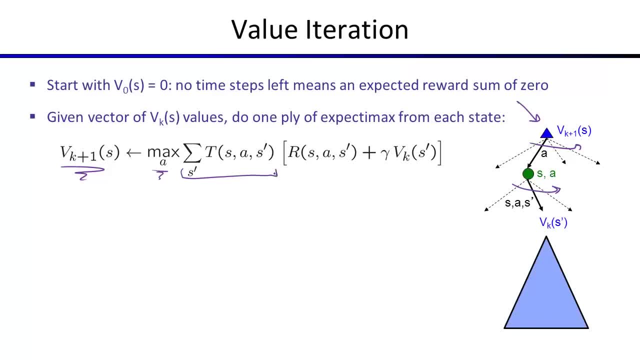 loop over the actions s prime. I consider all the s primes that are possible and then I average them together based on t, their relative probabilities For each of these actions and for each of the s primes that can result, I add together: 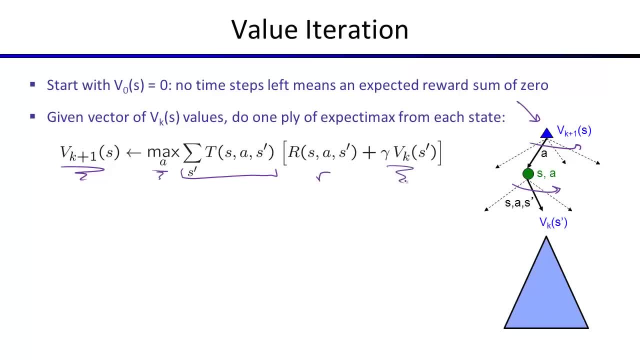 my instantaneous reward and then my future, which is a recursive call. Now, of course, it's not really a recursive call, because I've already computed vk. That's the way this algorithm works, So what I end up doing is to compute the. 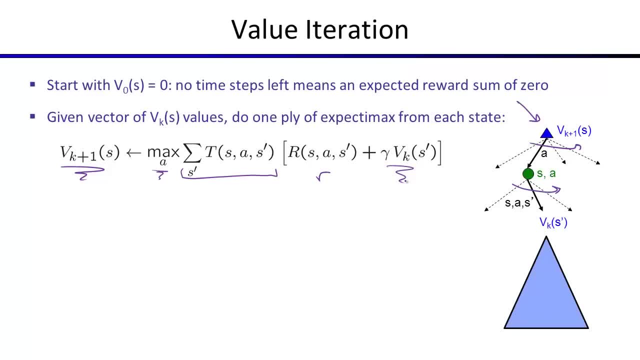 k plus 1 depth expected max. I actually only do depth 1 expected max Once I go down a single layer, my truncation function is already being computed for me, So you can see that over here in this tree The k plus 1 value. 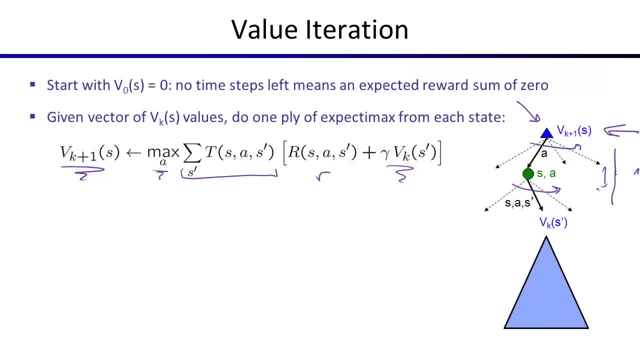 I go one layer ahead of each other. I go one layer ahead of each other And then I plug in vk from previous computation And that's it. You repeat that until convergence. Any questions on this? before we talk about convergence, for a little bit. 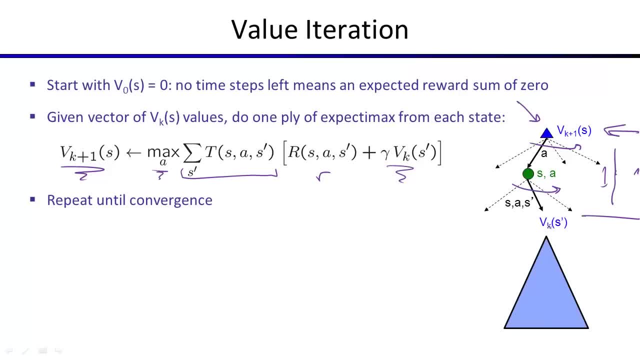 Okay, so v0 is easy. You compute v1 from v0,, v2 from v1, and so on. How long does this take? Well, you don't necessarily know how many iterations you're going to do, so there's some amount of work per iteration. 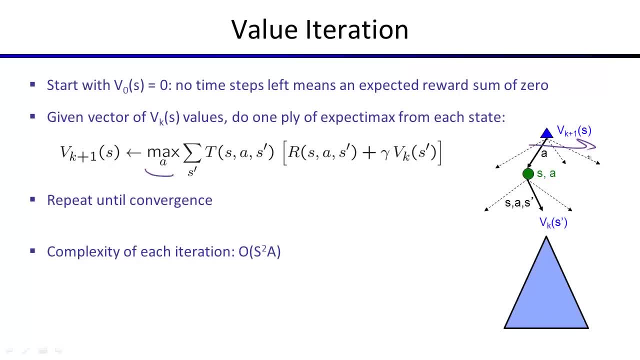 But for each iteration what do you do? You do a loop over the actions So you get a factor of a. You have to try every action from this state. Then you're going to iterate over the s primes, The possible outcomes. 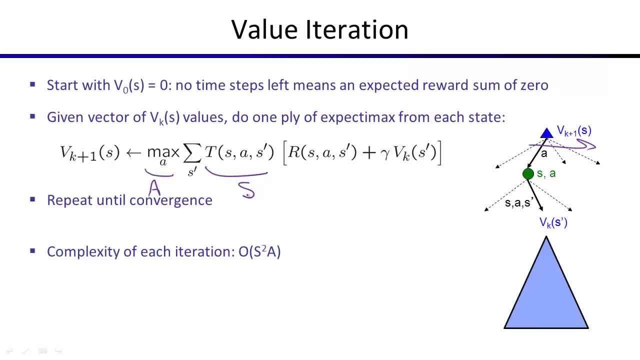 So there's a factor of a for maxing over all the a. There's a factor of capital S, the number of states, because you're looping over all the states to take the average And you have to do this computation for every state over here. 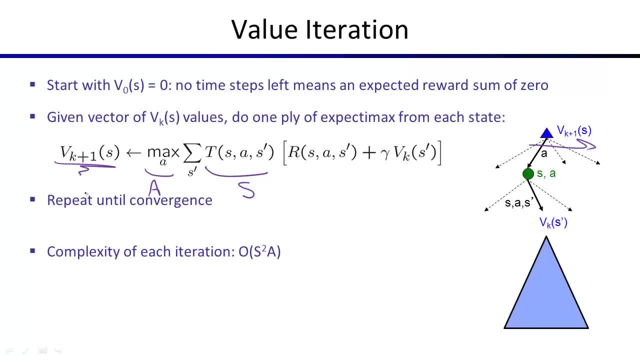 So when you compute vk plus 1, it's not for one state, it's for all the states. So there's a factor of s over here. So this whole thing is s squared a. In practice it's not that bad. 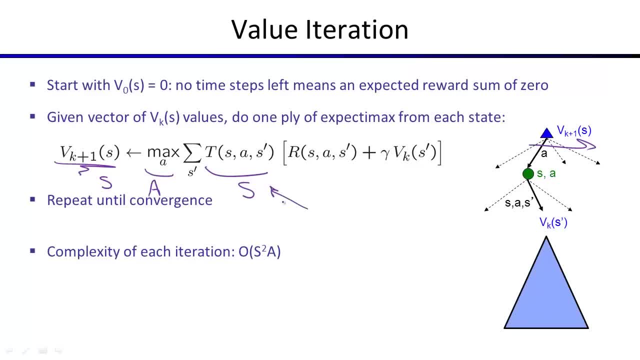 because usually when you take this expectation, there's only a small number of states that are possible. But in the generic case this is quadratic in the number of states, which means this is only going to work if there's a small number of states. 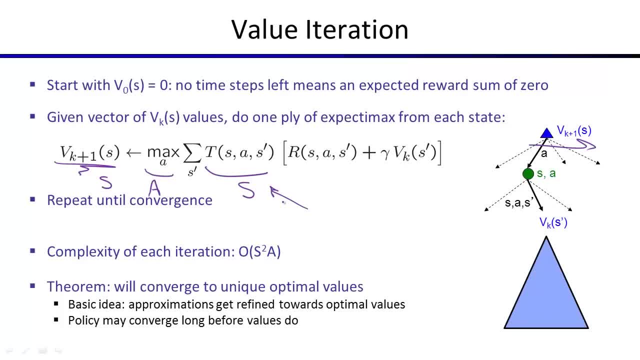 and linear in the number of actions. So what do you guarantee? There's a theorem that says this will converge to unique optimal values. in a fine print, The basic idea is that, as you do iteration after iteration, they start off all zero and they end up with the right answer. 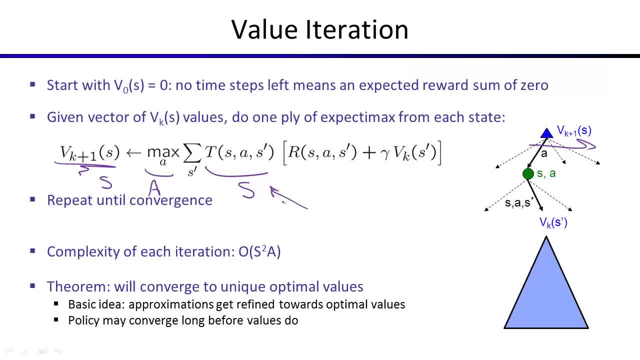 and they get closer and closer to the right answer every iteration. Now I'm going to show you something in a demo for a second that will make this last bullet clear about the policy converging long before the values do. But let's first talk a little bit about an example. 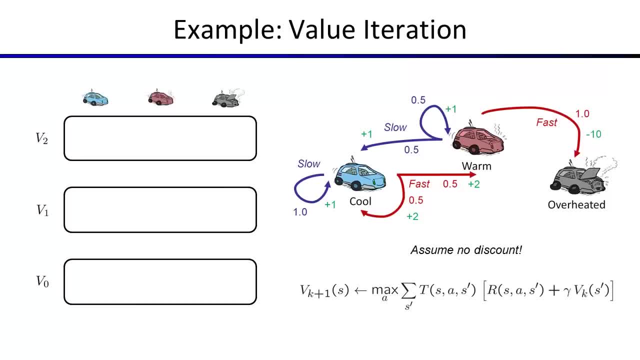 and then we'll talk about convergence and then I'll show you about this issue, from that bullet point about policy: Policy is converging faster, Okay, so v0.. Here are my three states up here, Let's compute. v0.. Easy, Zero, zero, zero. 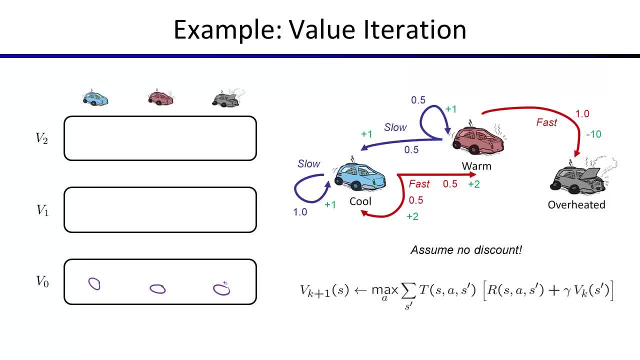 That happens to be the score I would get on average, acting optimally over zero time steps. but it's just zero. Let's talk about v1.. v1 for each state involves a tiny little expectamax that says: what can my score be? 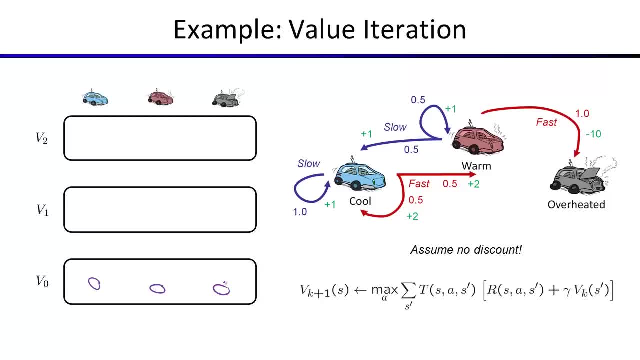 if I have one step left. So let's do an easy one. If I'm overheated, zero. You can never get points again from the overheated state. Let's talk about the red state- warm. Well, what can I do? 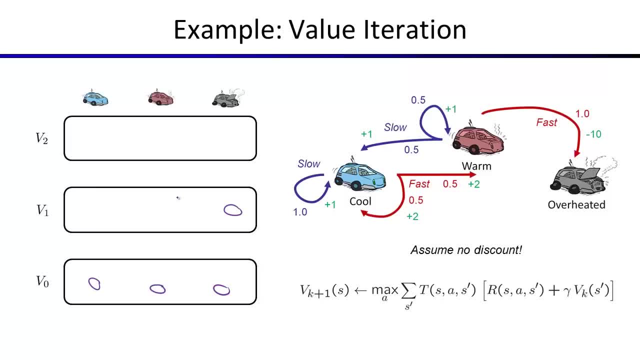 in one step from warm. I can go fast and get a minus ten, or I can go slow and get a plus one, So one is what I should do. That's my expectamax value of depth. one from red. How about blue? 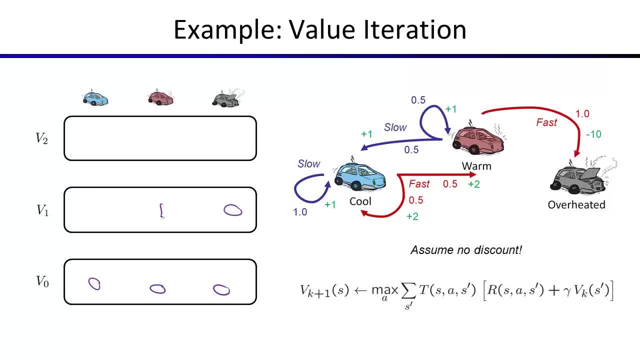 What can I do? I can go fast and get a plus two, or I can go slow and get a plus one. so from blue I should go fast and get two. Nothing's interesting until this next level. The next level is kind of interesting, Except not here. 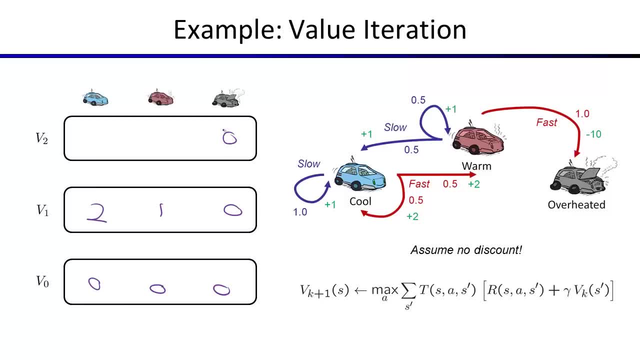 Because it's just zero again from overheated. Let's think about the red state. So we're going to compute this number right now. Okay, What's this computation? look like It's a depth one expectamax where, when I think about the future, I plug in v1.. 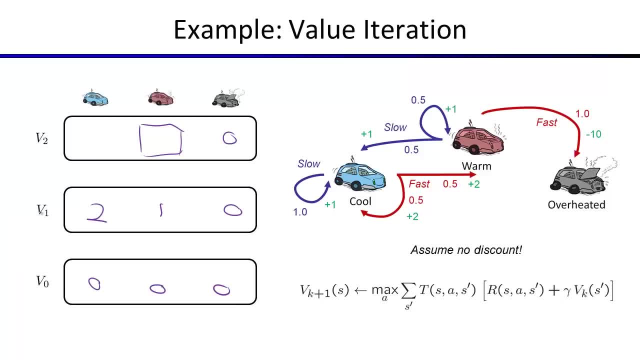 So how does this computation go? Well, I have to consider both of my possible actions, which are fast and slow. Let's think about slow first. If I go slow from the red state, what am I going to get? There's a 50% chance that I'm 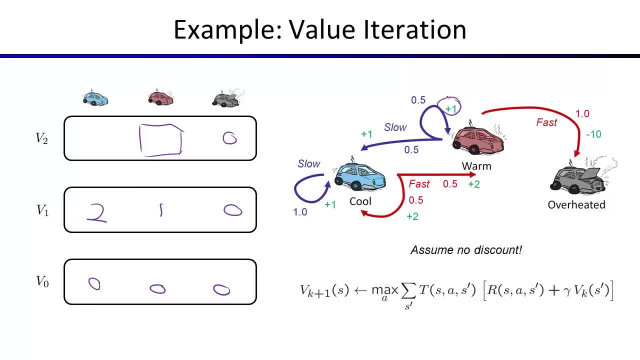 going to get a plus one and then land back at the red state. If that happens, what's my total score going to be- Assuming there's no discount here- Plus one, and then I'm going to land, and then I'm going to act for. 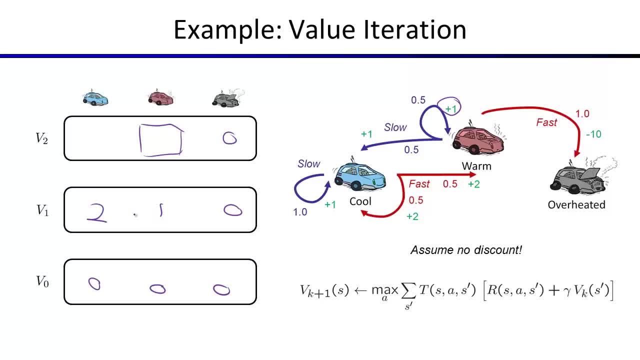 one more time step so I get to there. So one and one, which is two. So one possibility is I could go fast and then I would get a two, Sorry, slow. The other possibility is: I could go fast. What happens if I go fast? 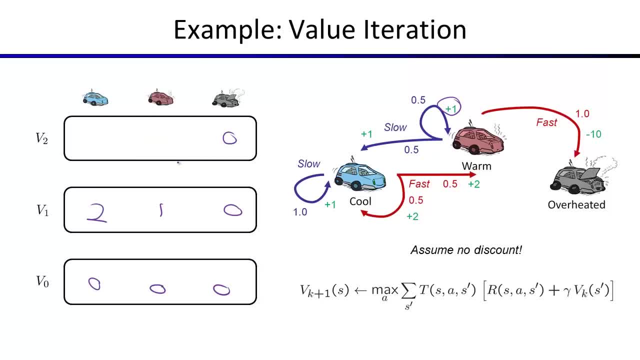 Sorry, I broke this. Let's try that again. So in this computation there's two options. From red there's fast, which is bad. We know if going fast is going to be bad, Because if I go fast, what is my score? 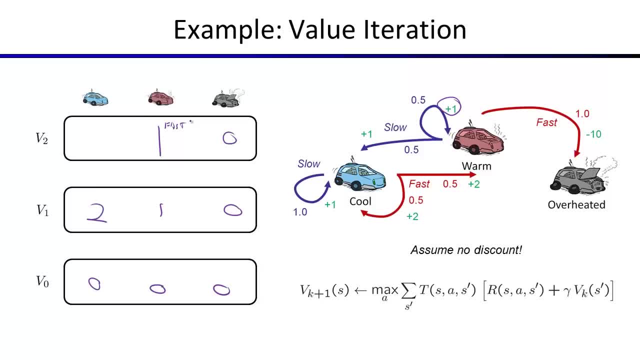 over the next two time steps. It's negative ten. I get a negative ten and the game ends. So if I go fast it's going to be minus ten. So that's probably not going to be the number for v2.. What happens if I go slow? 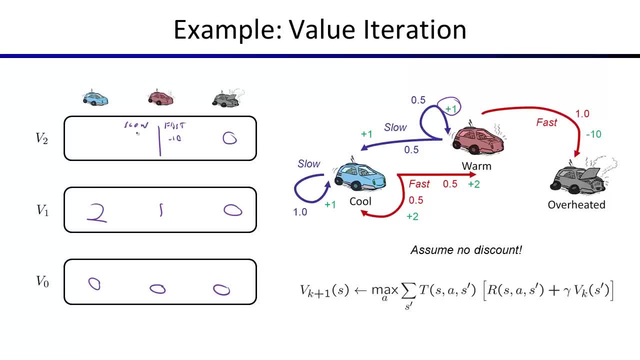 If I go slow. there's two possible outcomes of going slow. One is I end up at one and one is I end up at cool. Either way, I get a plus one immediately. The difference is if I land at cool, then I'm going to have 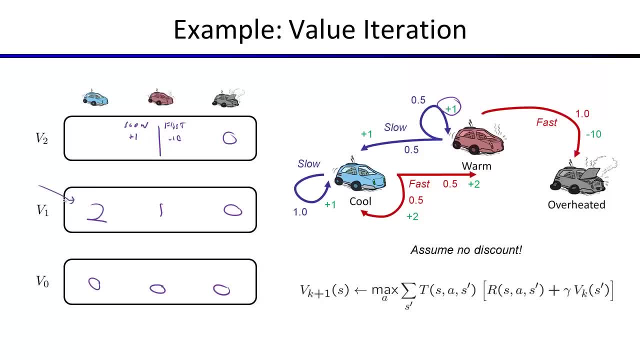 a value of two in the next time step. That's this number. If I land at warm, then I'm going to have a value of one in the next time step. So in the future I'm going to get the average of those. 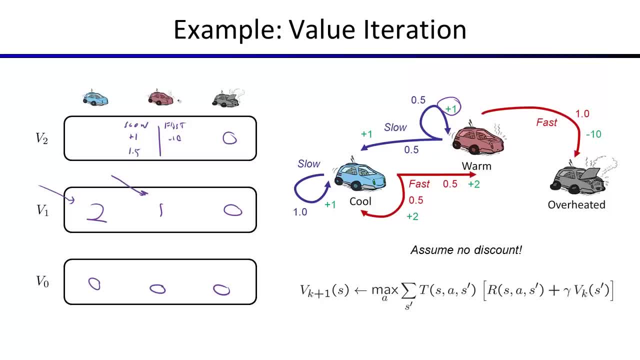 so 1.5.. That means that I should choose slow for v2, and the sum is going to be 2.5.. So if I erase the work table, the sum here is going to be 2.5.. If I work that out here as well. 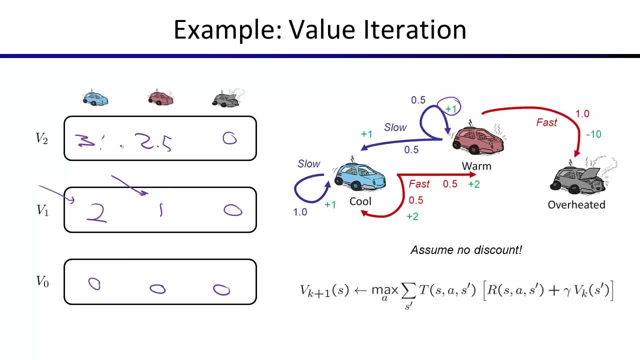 I'll get 3.5.. It's not really a .5,, is it 3.5.. And I can keep doing this And as I go higher and higher. what are these going to converge to? What is v sub 100 of cool?